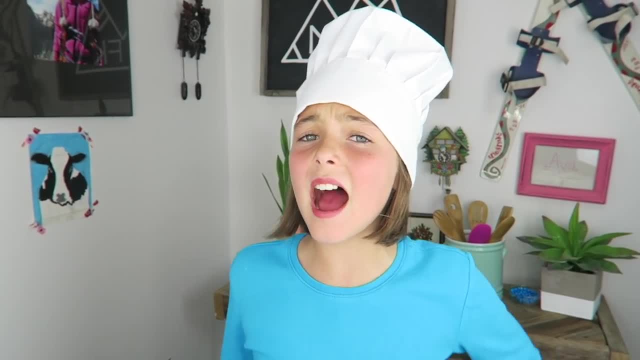 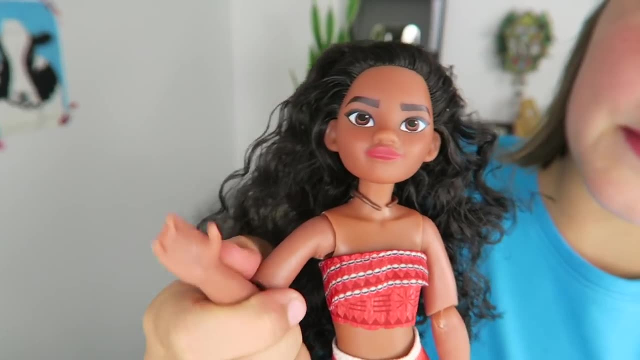 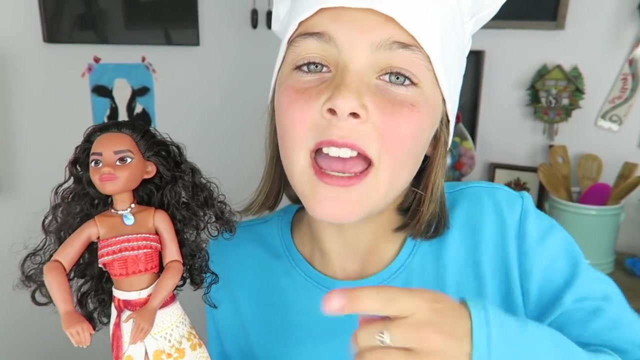 Hello everybody, Welcome back to Kids Cooking Crafts, And today I am joined by Moana. Say hello Moana, Hello, Hello everybody. Let's get this video to a thousand thumbs up. Also comment down below if you saw her movie And what was your favorite part. 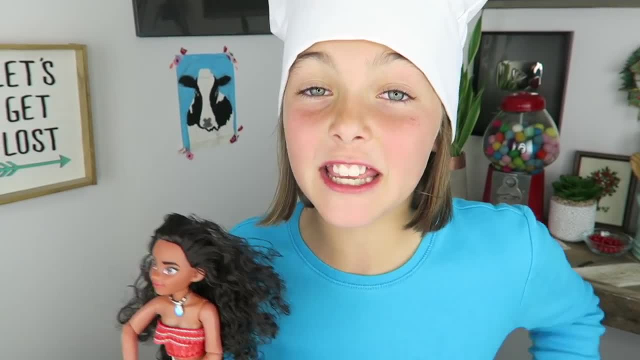 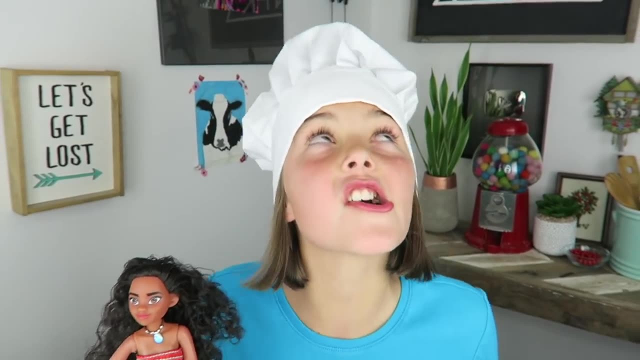 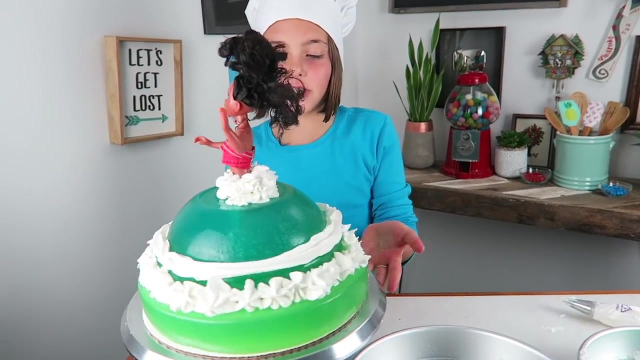 My favorite part was when Heihei figures out that he's in the middle of the ocean and he starts screaming. That was a really funny part. Today, me and Moana will be showing you how to make an ocean jello dress for Moana. 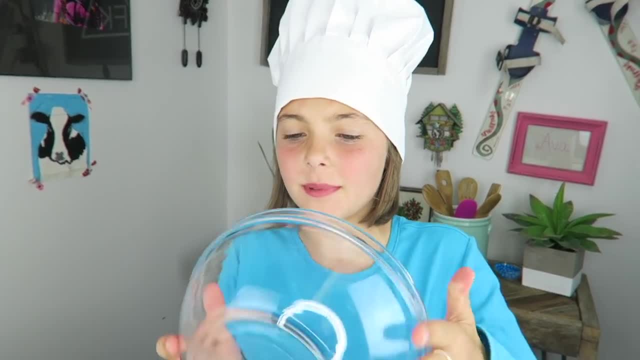 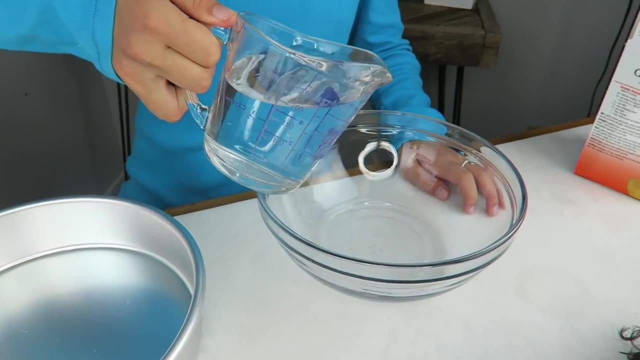 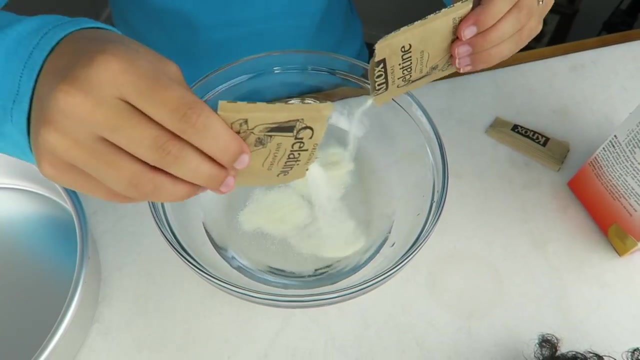 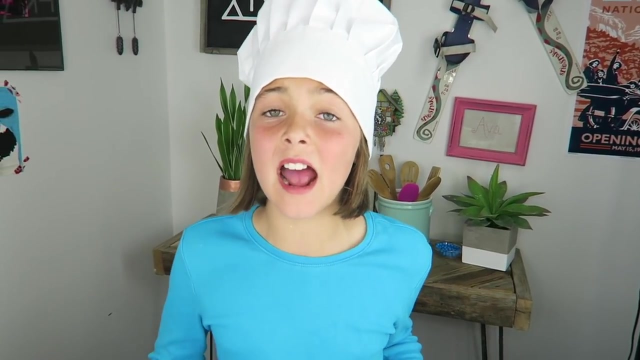 Alright, this bowl is going to be the top of our dress, because it's kind of rounded like a dress, So let's add one cup of water into here And four pockets of gelatin. Alright, we're going to let the gelatin sit and then we're going to add three cups of boiling water. 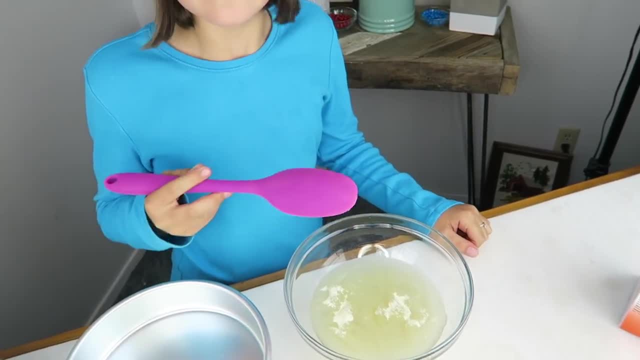 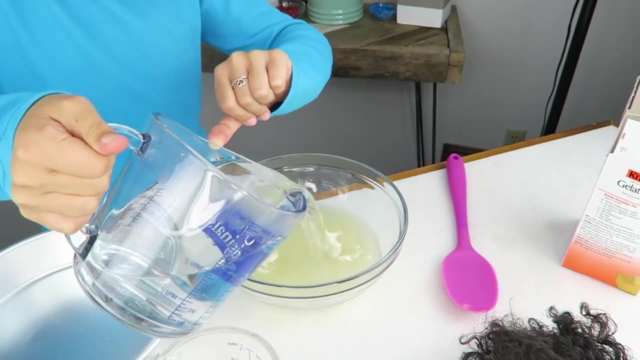 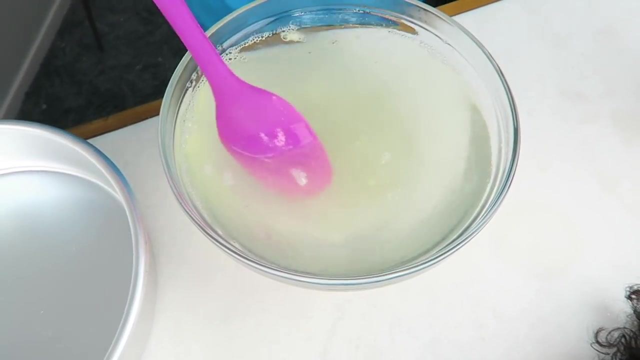 Alright, it's looking pretty soft here, so let's add our three cups of boiling water. Careful, it's hot. Stir it up until the gelatin is all dissolved. Now to add our coloring and flavoring, I'll be using a snow cone syrup. 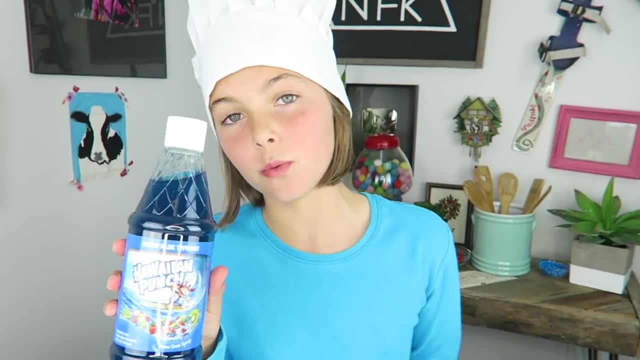 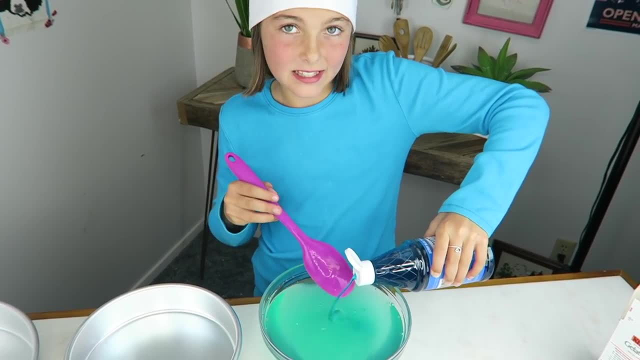 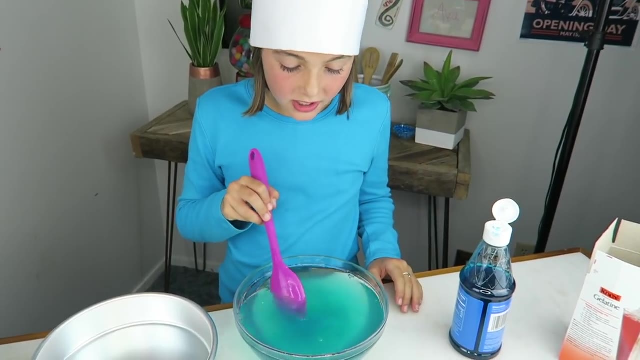 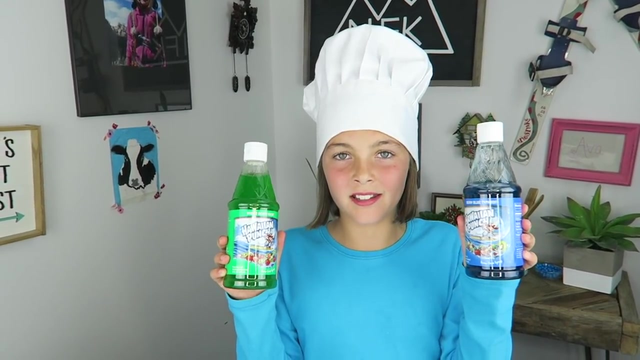 It is Berry Blue Typhoon. This will make it look like the ocean and taste like berries. Alright, I think we're good. We will be doing the same thing for the next one, except we will be using blue and green, So it's like a turquoise color. 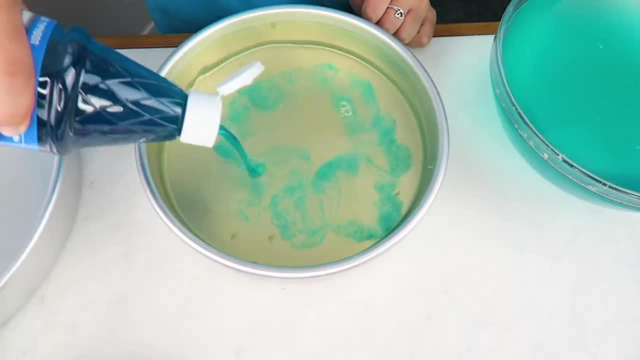 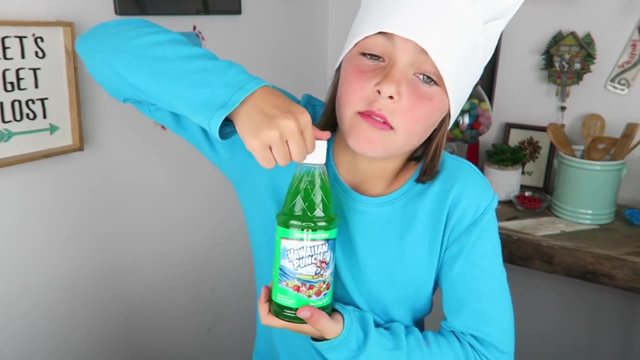 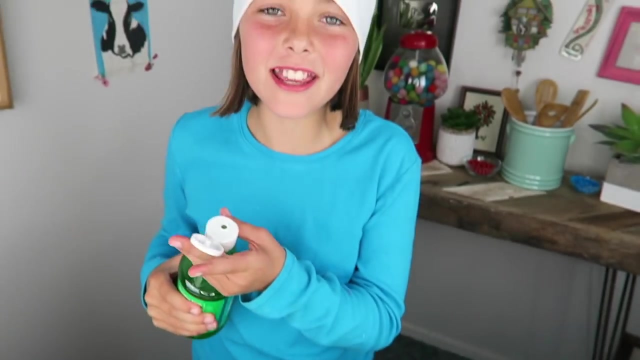 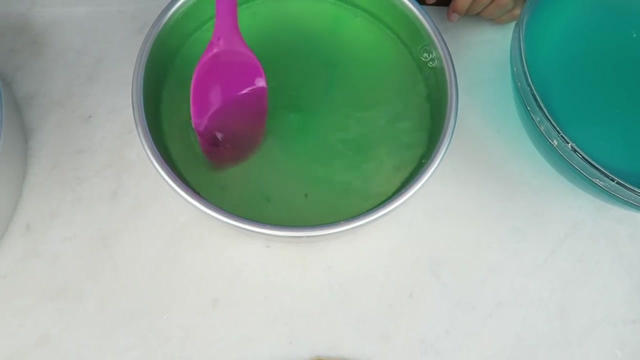 I'm just going to do half and half Now for some green. This one is Greenberry Rush. Well, I'm certainly in a rush. Ooh, look at that, That's so cool. Whoa, Ooh, look at that turquoise goodness. 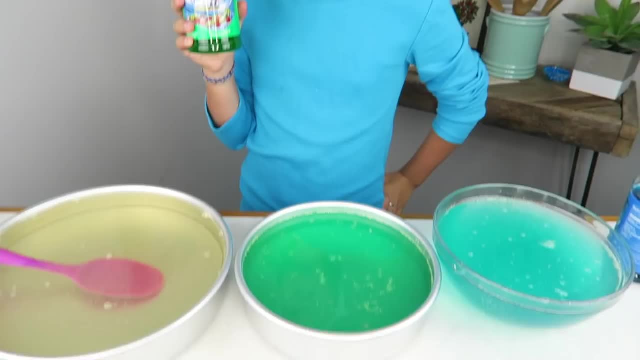 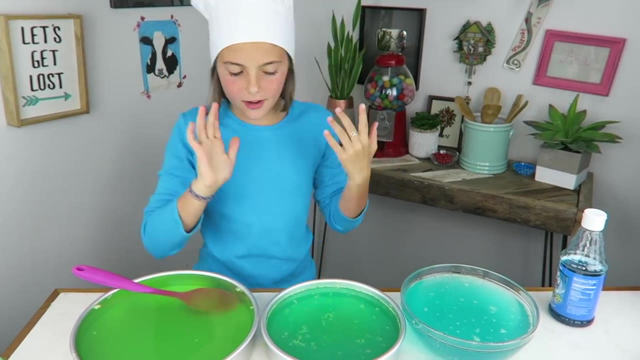 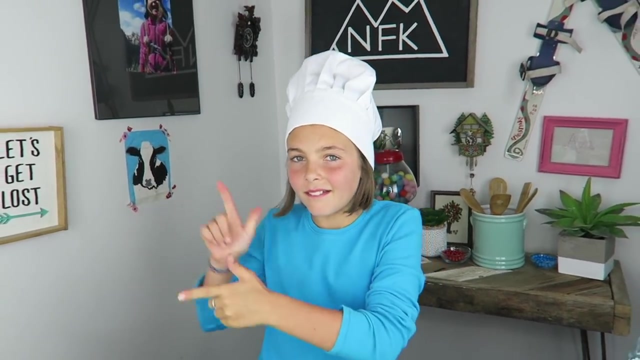 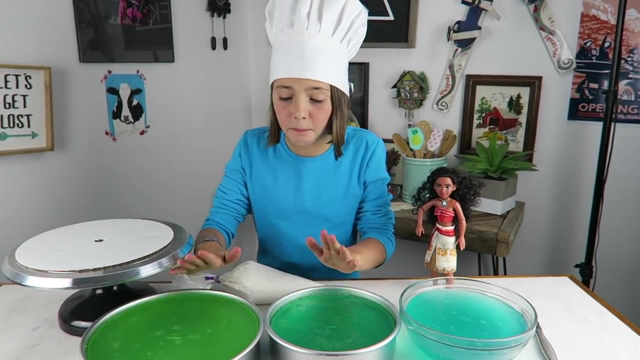 Now let's move on to number three. Time to add our green. Alright, we have our green, our turquoise and our blue ready. Now let's just go pop them in the fridge. Ta-da, Alright, guys, I just got these out of the fridge and they are completely solid. 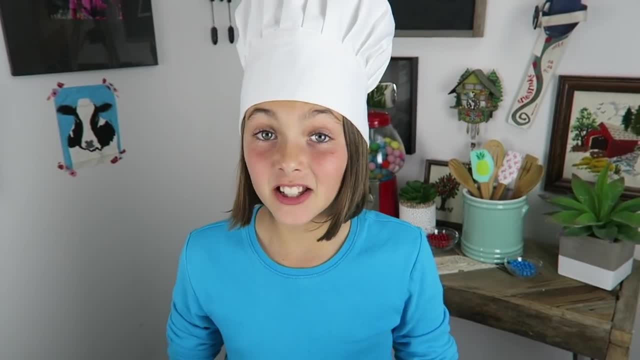 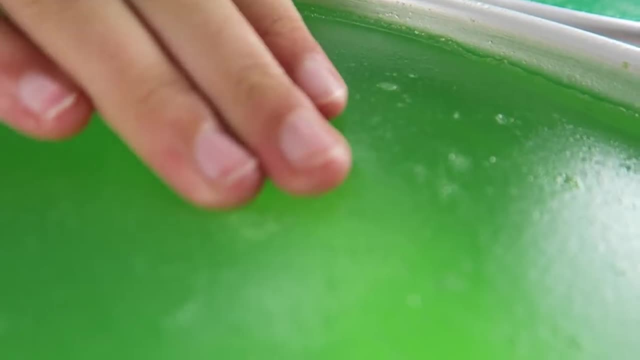 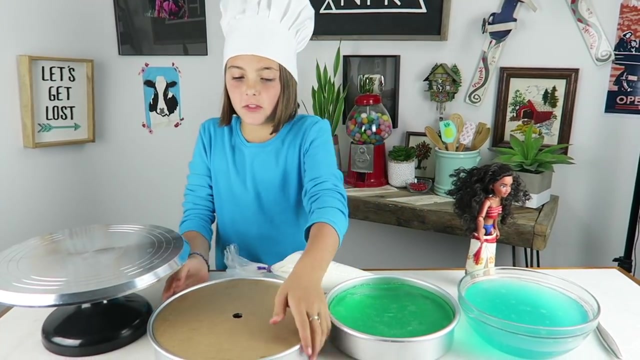 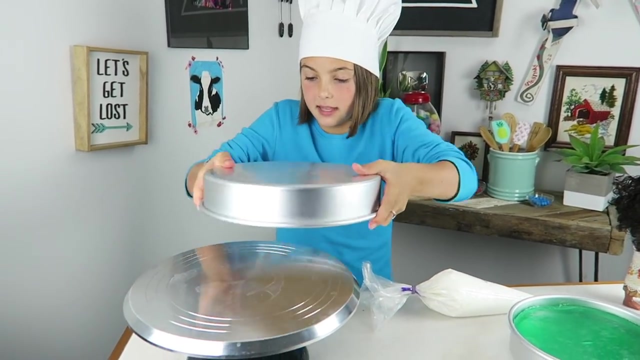 She's alright. Check this out, guys. Look how solid they are. We're going to start with the bottom layer. I'm just going to put the circle thing on there, like that, And then I'm going to flip it over, Set it on here. 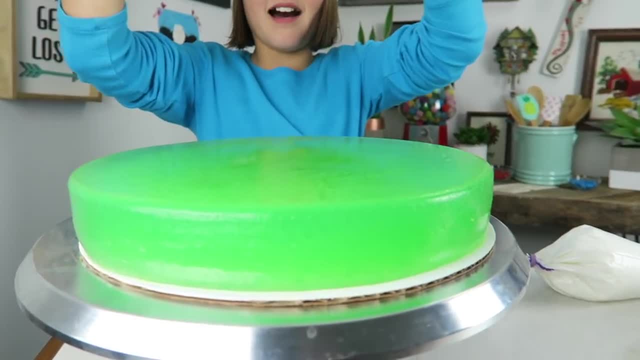 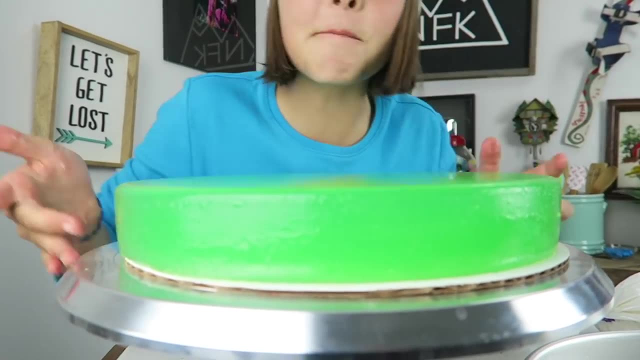 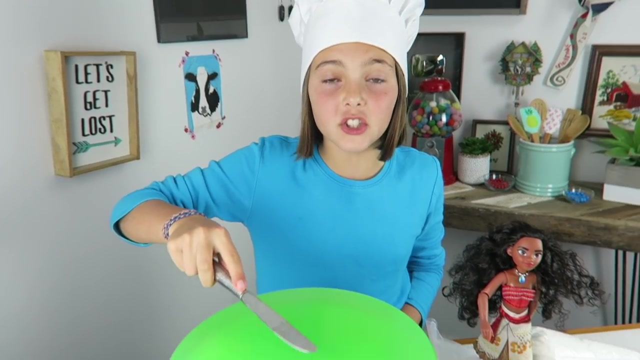 And then Voila Boom. Look how cool this is, guys, Oh my goodness. And it fits like perfectly onto this cardboard circle. Before we put the next layer on, I'm going to cut a hole in the center for Moana. 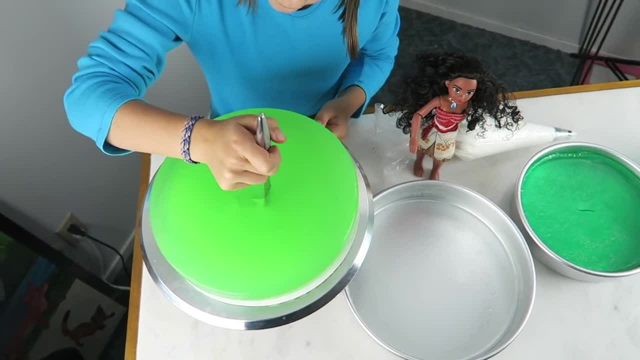 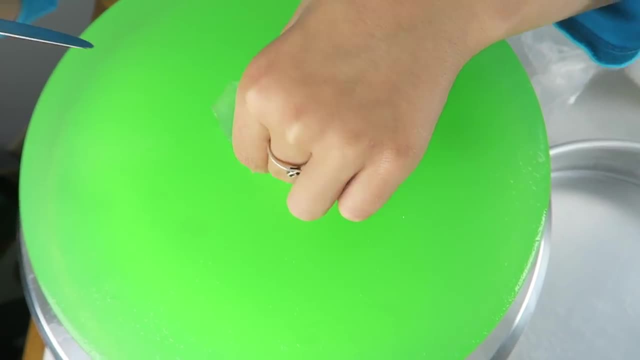 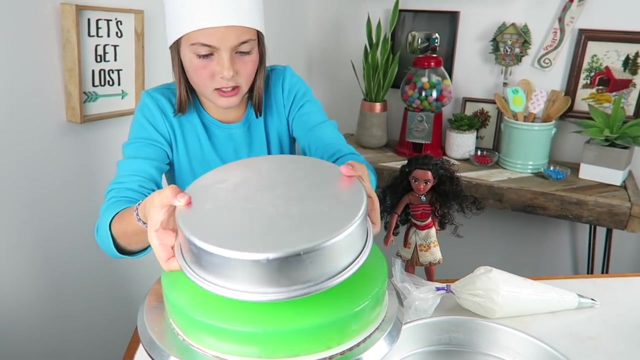 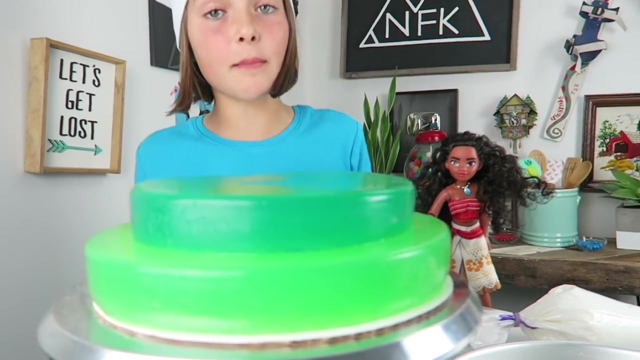 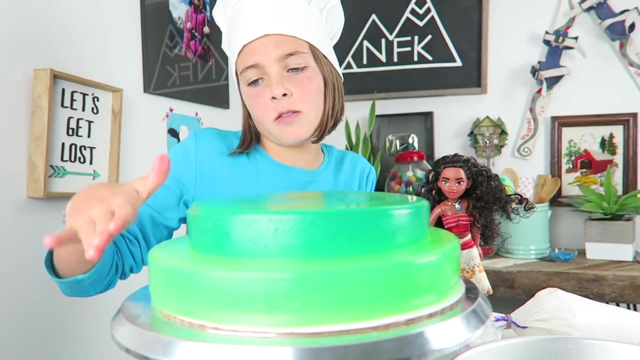 Time for the next layer. Oh, this is why you got to grease it, Because if you didn't grease the pan before you put the gelatin in, then you're going to have a hard problem. It split right out. Oh my goodness, look how cool this is. 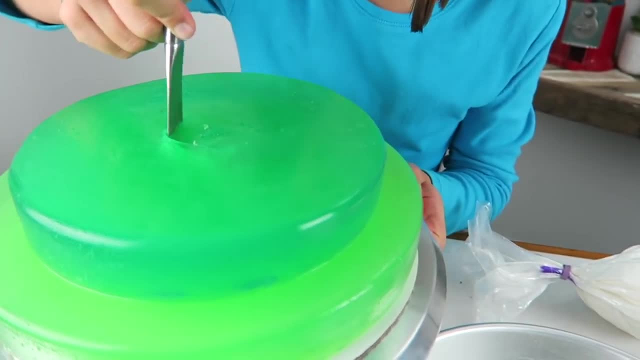 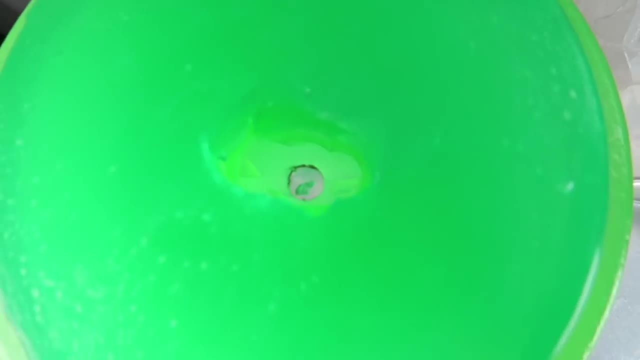 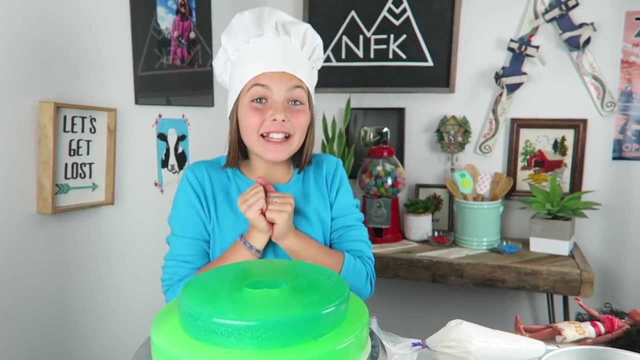 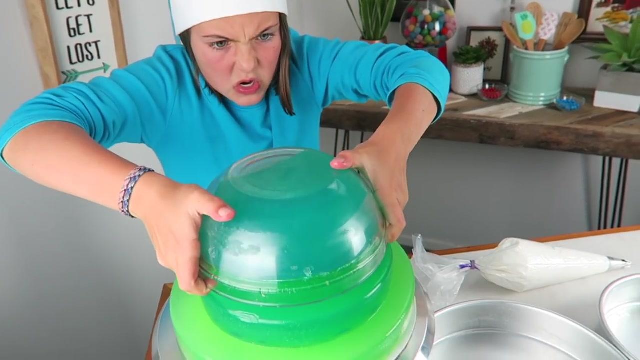 I'm just going to cut another hole. You can see through both layers. That's so cool. Okay, guys, last layer, This is going to be the coolest. Let's cut the last hole. Whoa, This is so cool. It's like blue, turquoise, green. 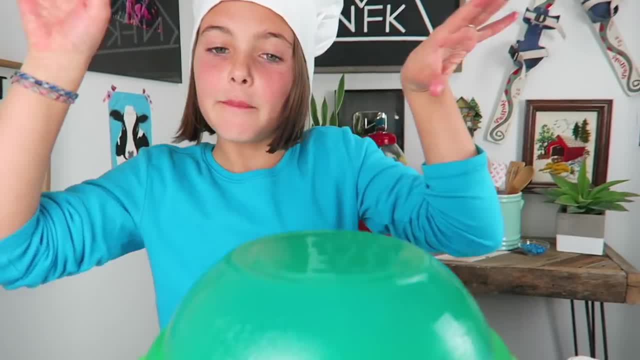 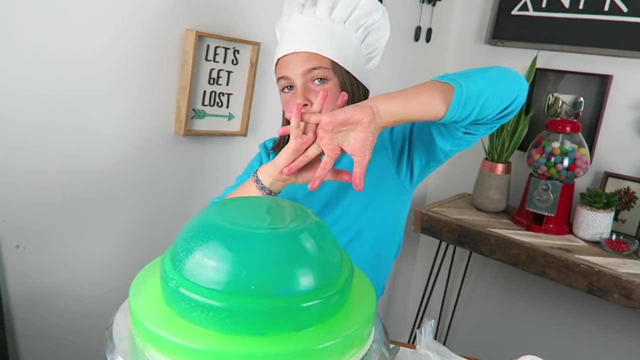 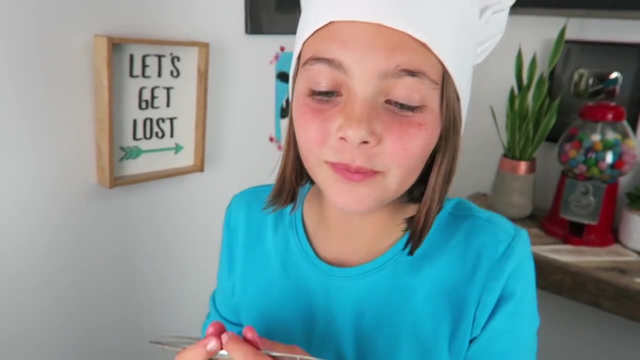 It's like. it's kind of like morphing together, Like the green and the blue are like smudging together to make the turquoise. Let's cut the last hole. Whoa, This is so cool. It's like blue, turquoise, green. 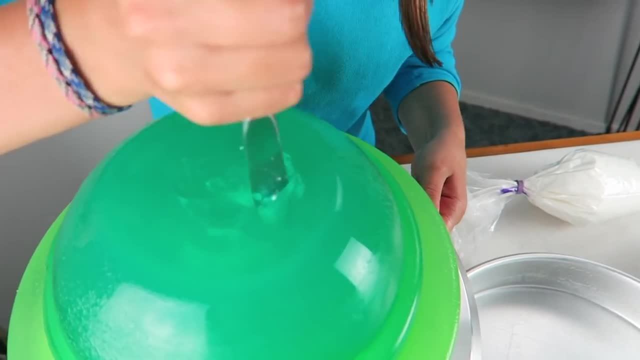 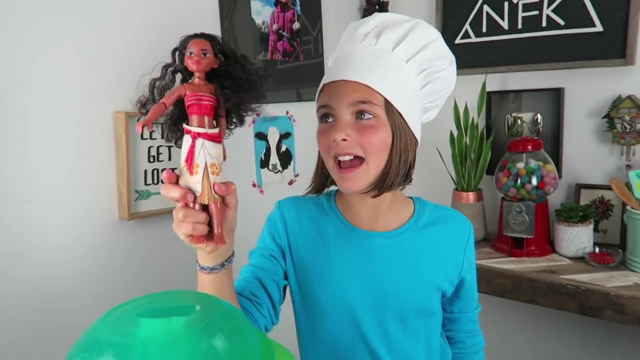 It's like. it's kind of like morphing together. It's like blue turquoise green. It's like blue turquoise green. It's like blue turquoise green. Time for Moana to dive in Yay. 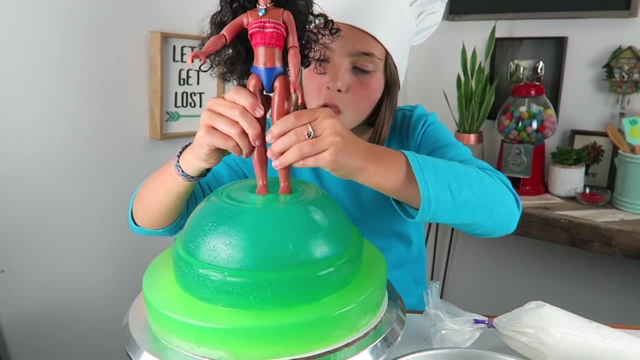 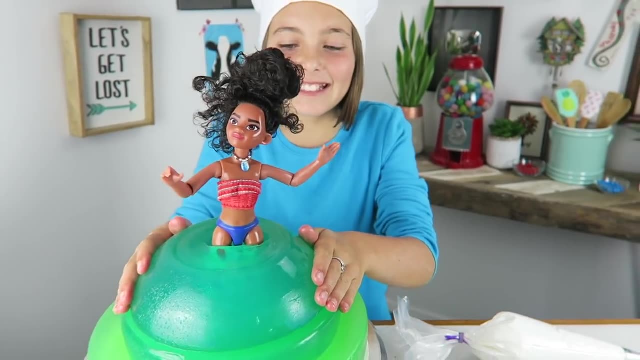 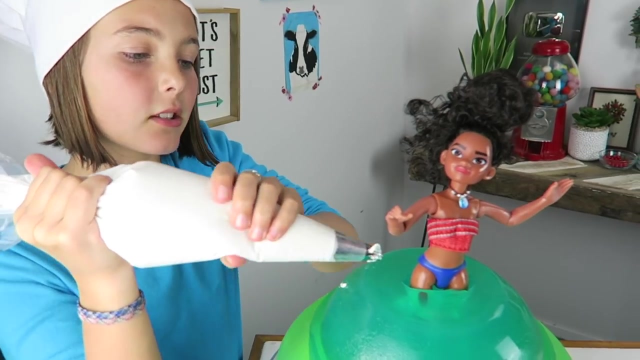 Here she goes. All right, guys, I put Moana's hair. Oh, she's doing a little dance. Okay, I put Moana's hair up so it wouldn't get frosting in it. All right, so I'm just making dots around her waist. 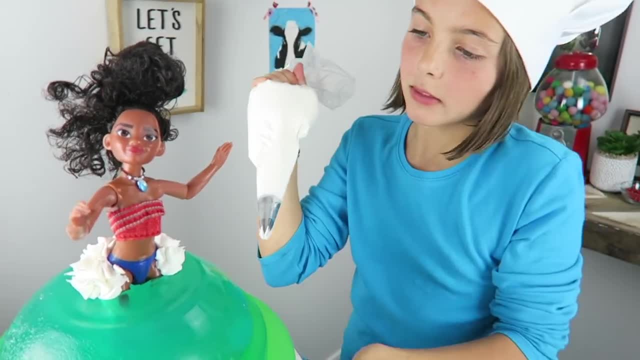 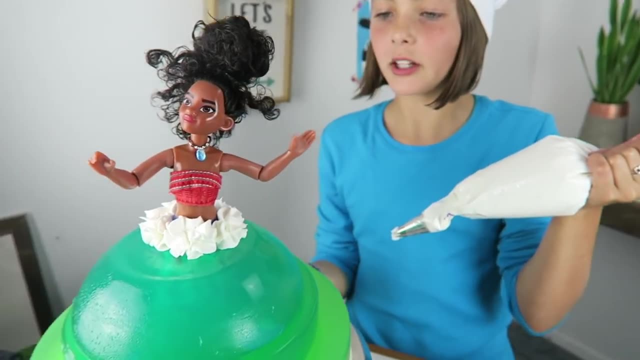 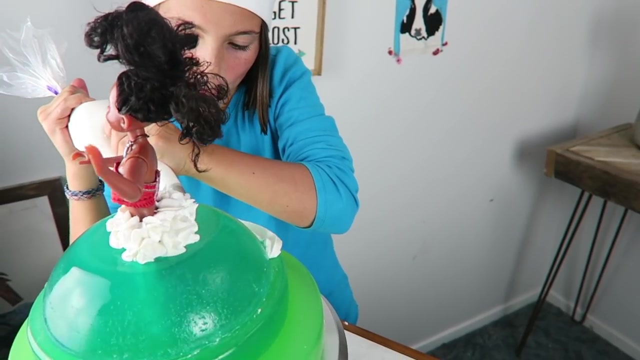 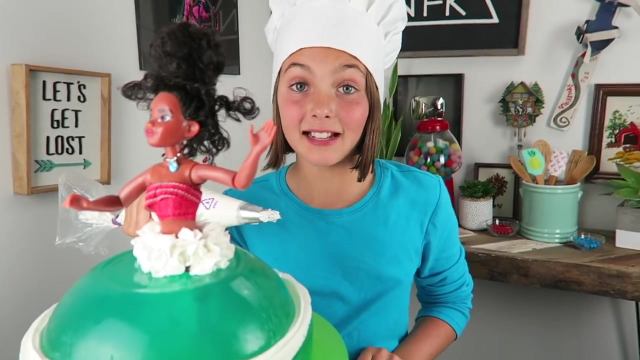 All right, so I'm just making dots around her waist. There we go. The waist is finished, Cha-ching. All right, now I'm going to add frosting to each layer. All right, last layer, And I'm going to put a whole bunch of dots, just like what I did on the very top. 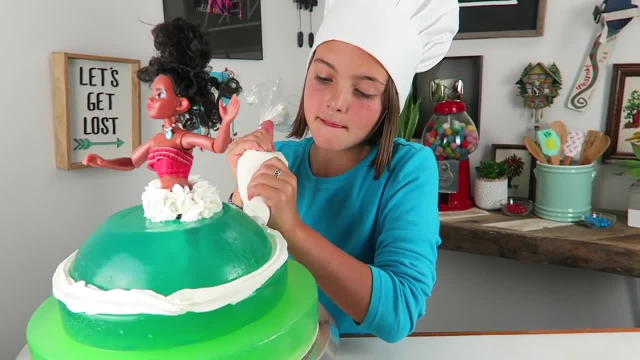 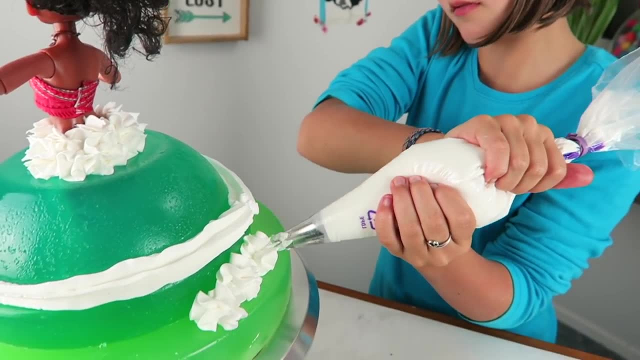 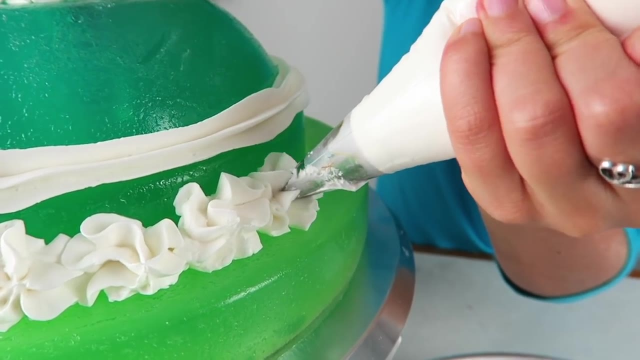 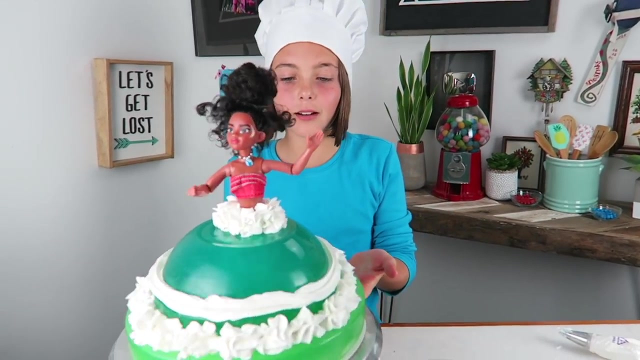 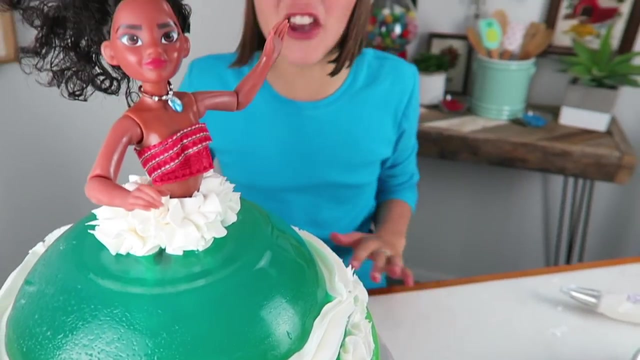 on the very top layer, Fluffy little frosting. Oh, this is looking delicious. There we go, Ta-da, she's perfect. Isn't this an awesome ocean cake? It's like the ocean is her dress. Now let's let her hair down. 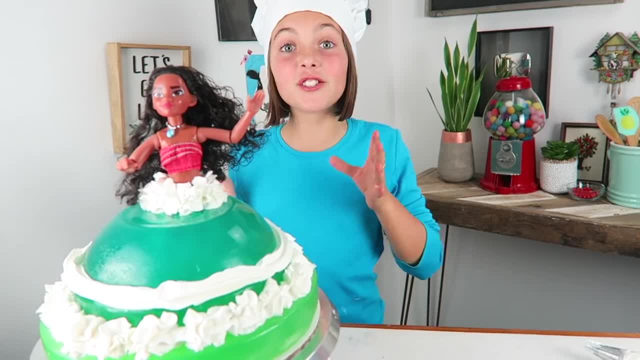 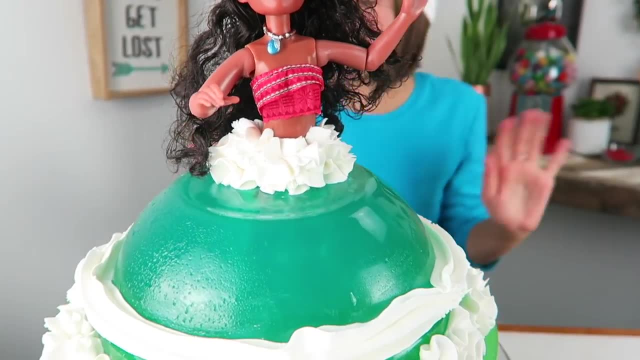 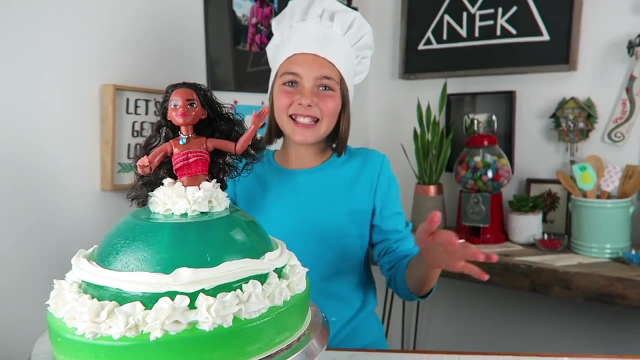 There we go, Ta-da. The Moana ocean jello cake is finished. Watch Jiggle, jiggle, jiggle, Jiggle, jiggle, jiggle. If you like this cake, then you'll like the Anna jello cake that I made also. 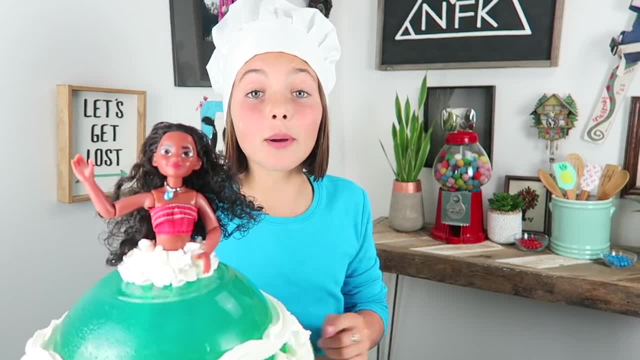 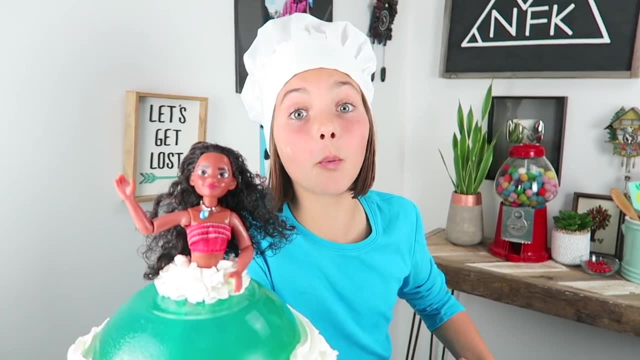 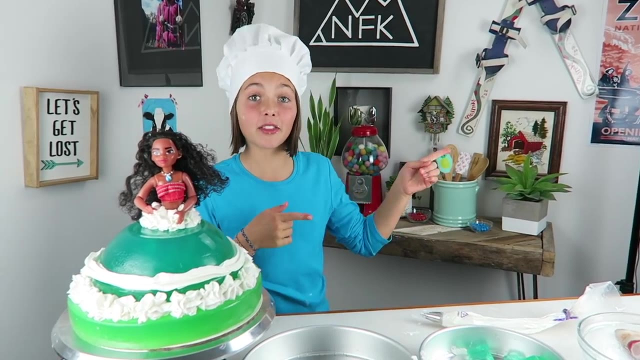 You can check that one after this one. So we usually give our cakes away. but my brothers promised if they would do my chores for a week if they got to destroy this cake. So go watch that video on their channel. Oh, here are the boys. 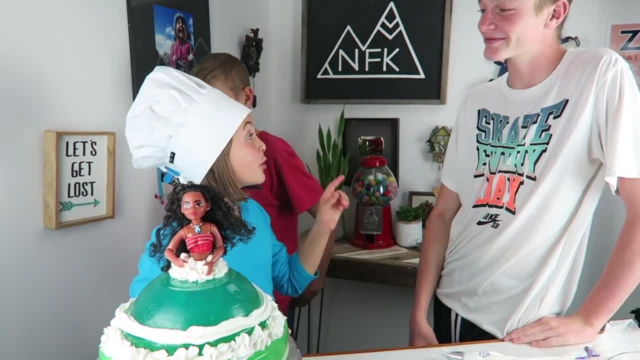 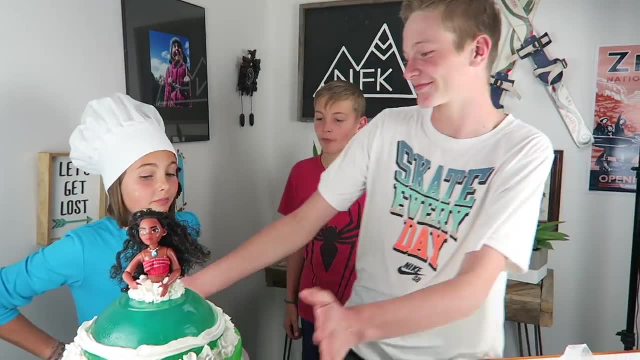 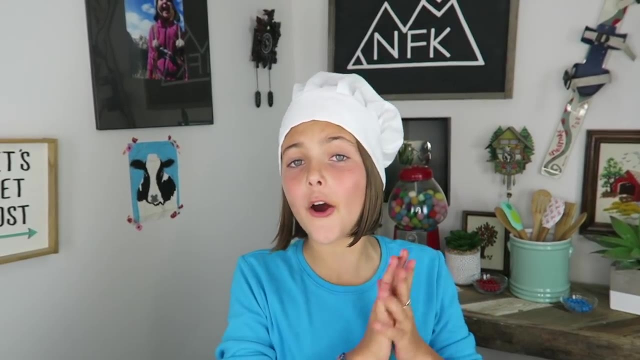 Hey, Hey, How's it going? Okay, do you promise that you will do my chores for a week? Yes, I promise Totally. Goodbye, Moana. Thank you guys so much for making this Moana ocean jello dress with me today. 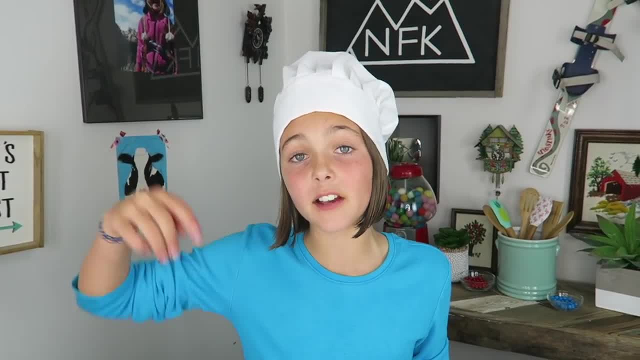 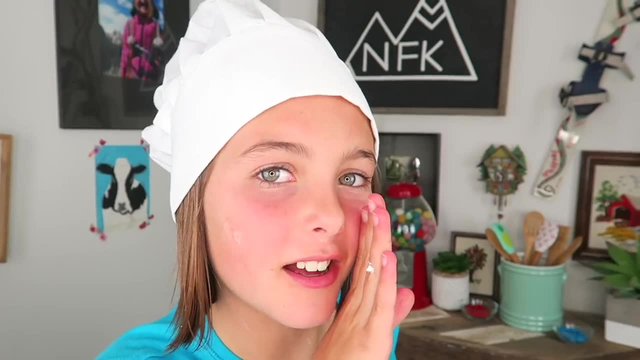 It was so much fun to make. And don't forget to like, subscribe and comment down below what Disney princess jello dress we should make next. And don't forget to watch my brothers destroy the awesome jello dress that I made on their channel C&C. 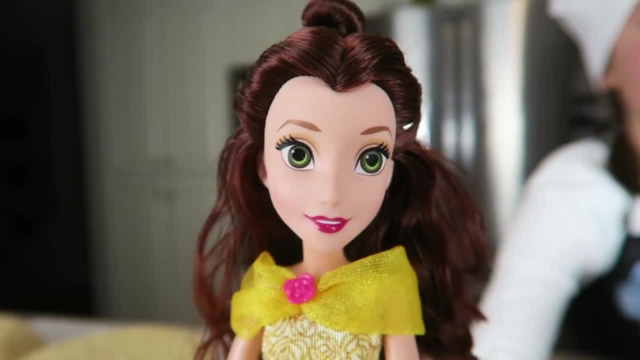 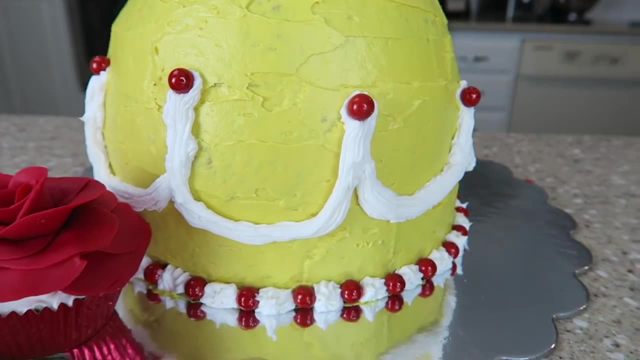 Bye, Hello everybody. Welcome to Kids Cooking Crafts. I'm Princess Belle And today I'll be showing you how to make a Beauty and the Beast Princess Belle Rice Krispie Dress Cake- Just kidding, It's only me, Chef Ava. 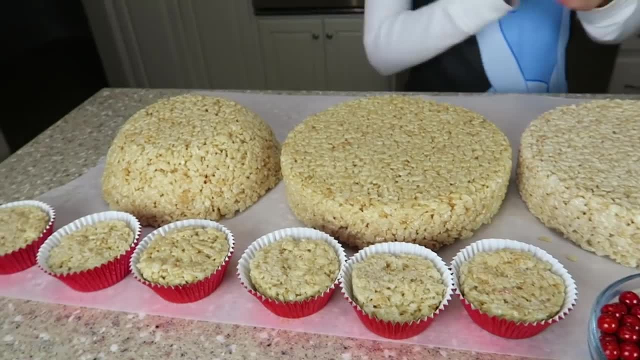 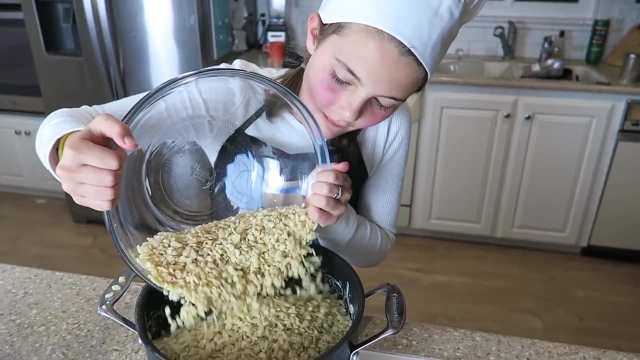 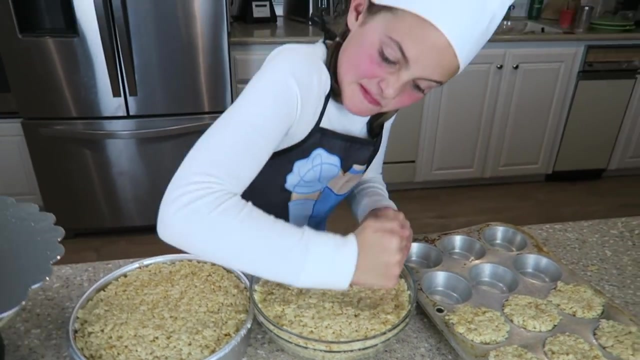 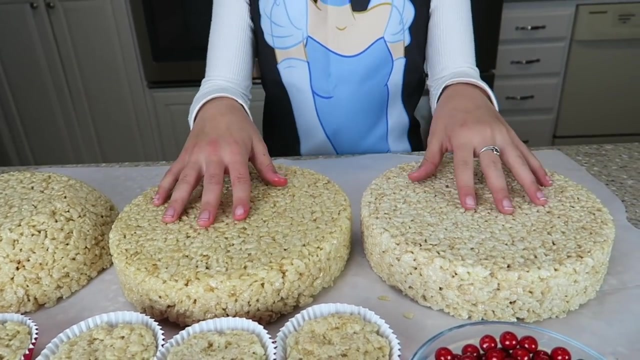 As you can see, I have all of my beautiful cake parts. I used five batches of Rice Krispies. I poured all of our Rice Krispies treats into a mold and pounded it, and so it was really compact. This was our bowl and these were a round cake pan. 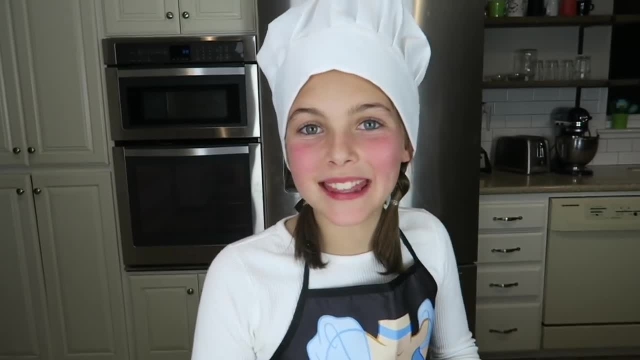 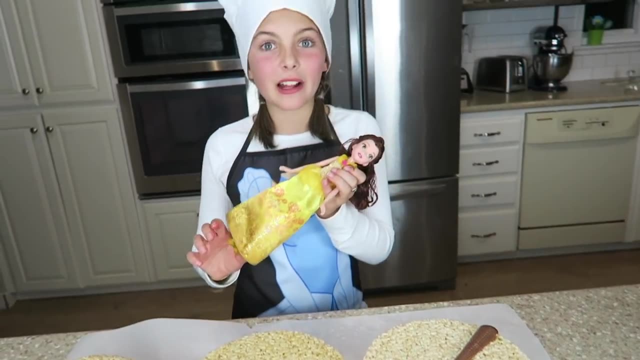 These were in our cupcake pan. Now let me show you how to make this cake dress. So, first of all, what we're going to do is cut holes inside of the Rice Krispie molds and so that Belle can slide right in. 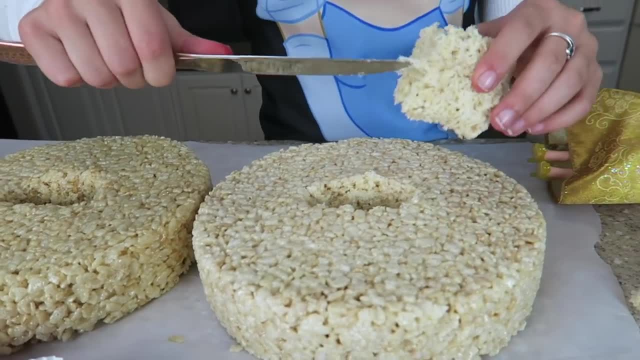 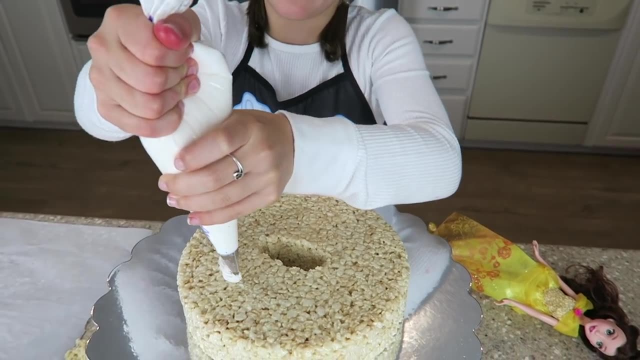 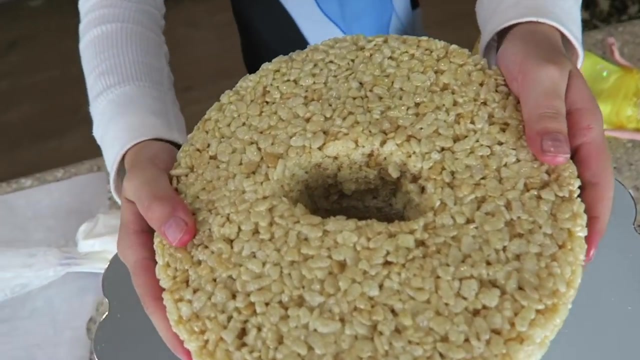 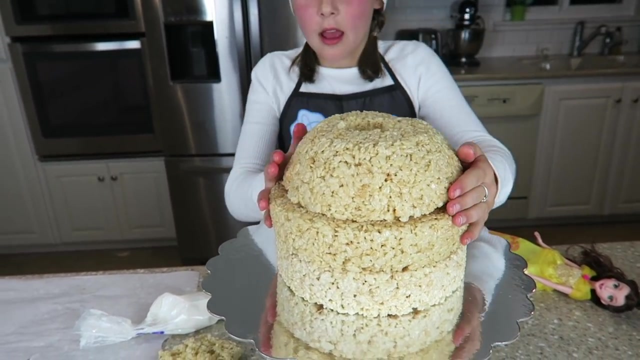 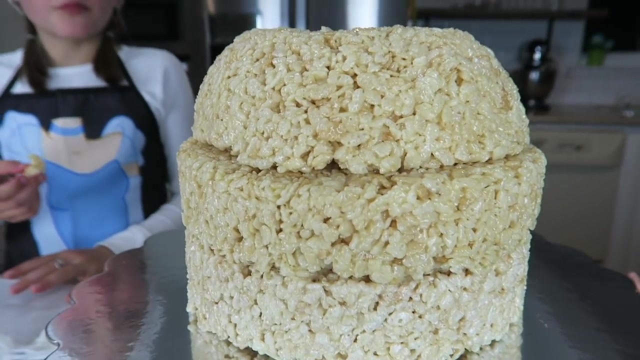 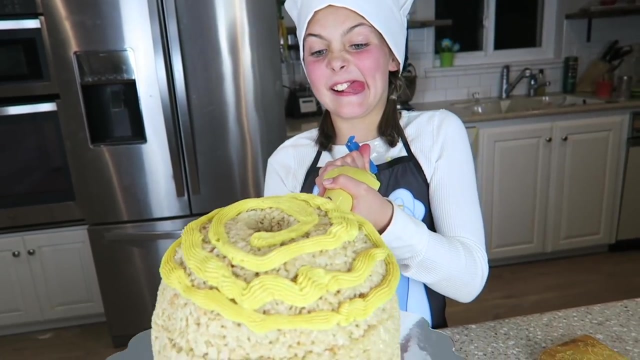 I'm just going to put a little bit of white frosting in here so the next layer can stick. Make sure the holes are lined up. Last layer: See how it's kind of like a bottom of a dress. Okay, Now we're just going to frost the whole cake yellow. 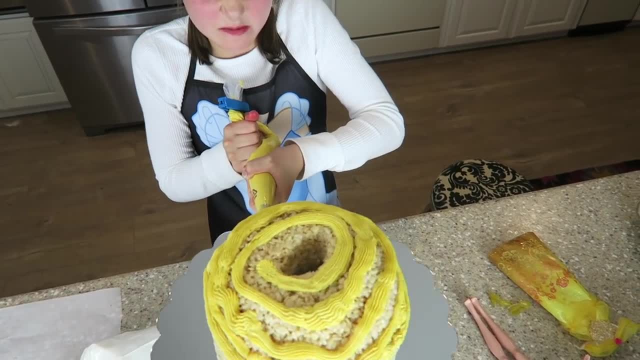 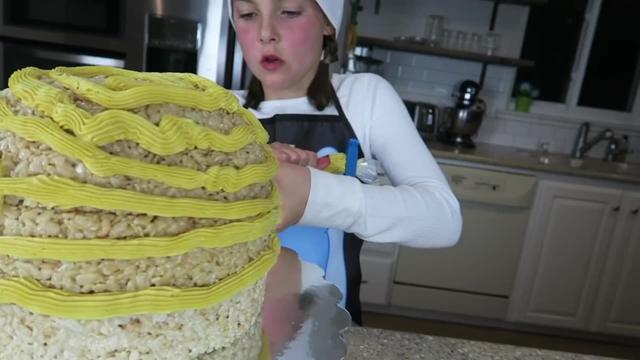 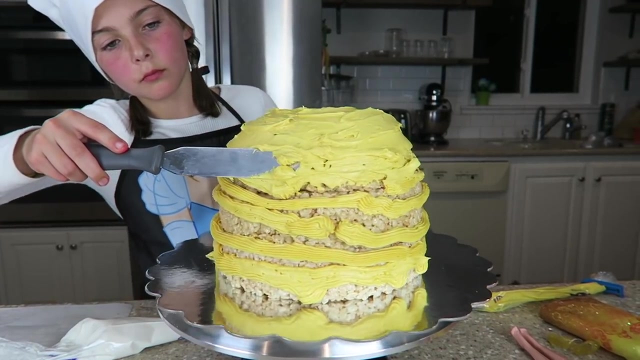 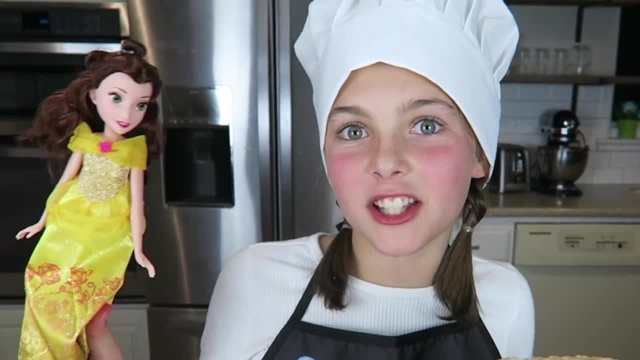 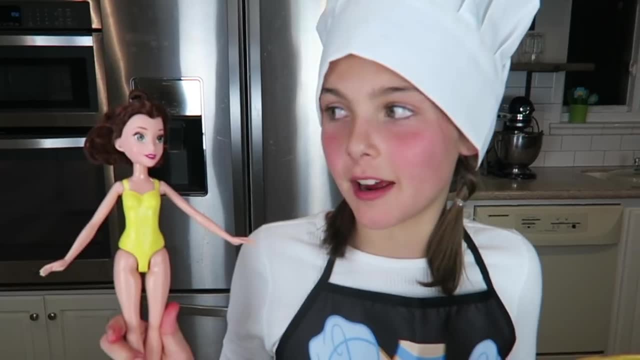 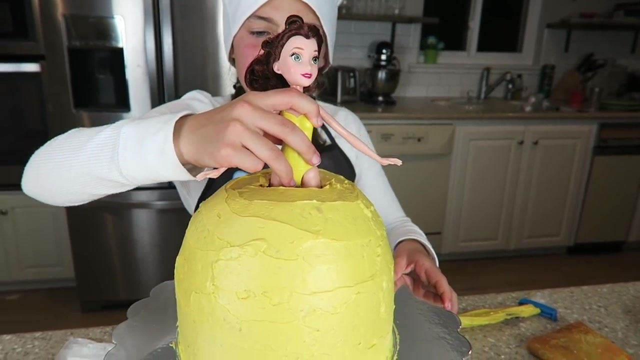 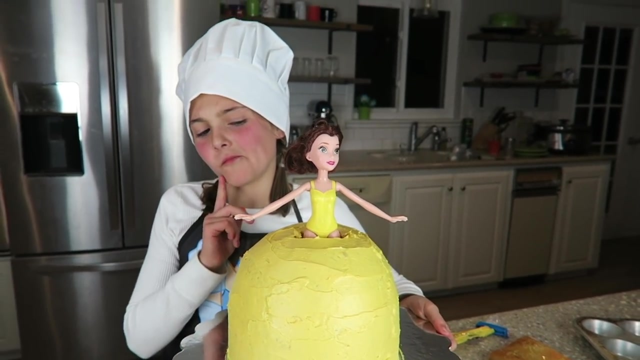 Let's get Belle ready to jump in. Going to take off our pretty little shoes. You're ready to dive in, Belle? Let's do this thing. Found my jewelry. There we go. What do you think? Hmm, I think it needs a little bit more detail. 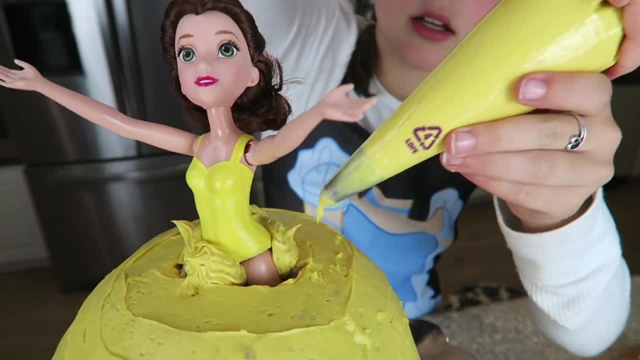 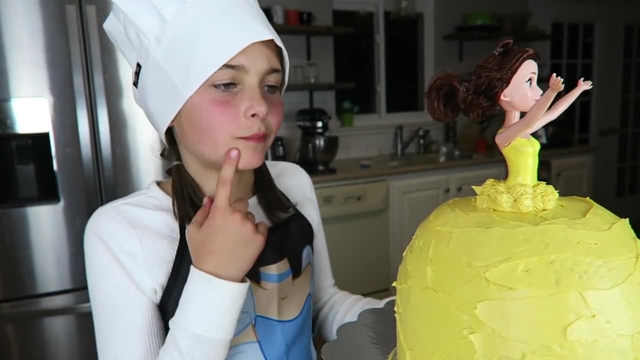 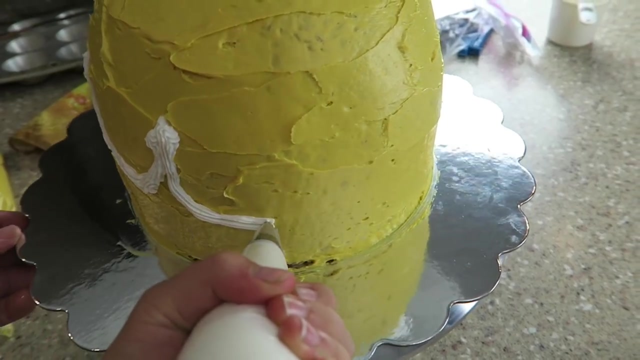 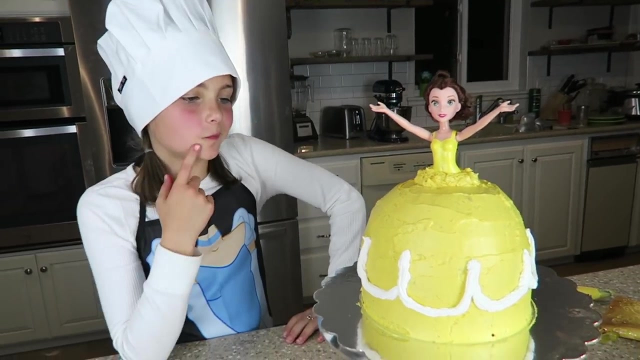 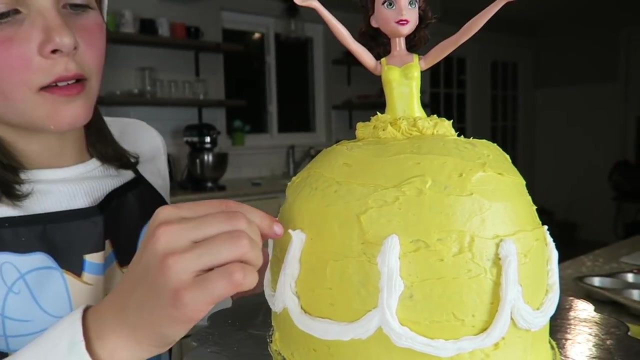 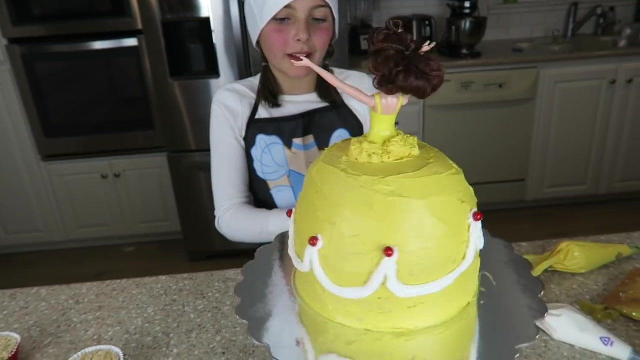 to cover up this gap. there we go. hmm, I still think she's missing something. why don't we add like the loop-de-loops on the side? here we go. hmm, oh, I know I'm gonna add to be chocolate candy on each tip. here we go. wow, and she was awesome. 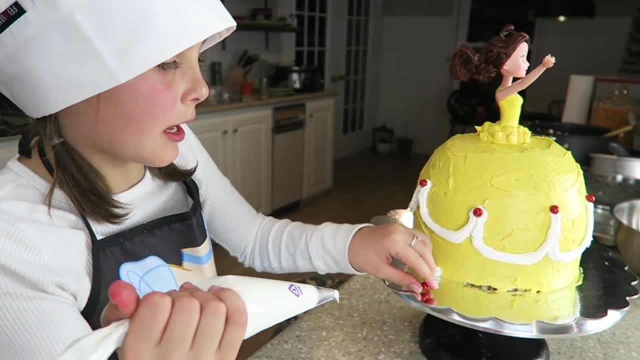 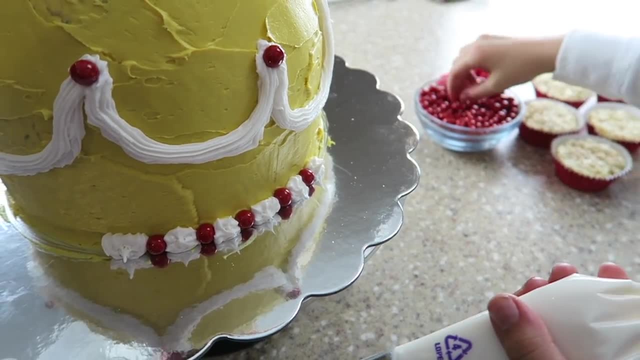 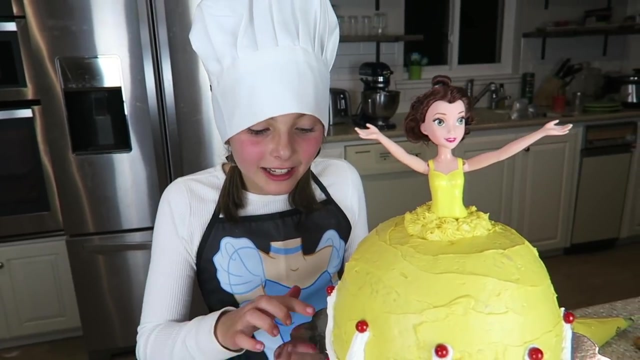 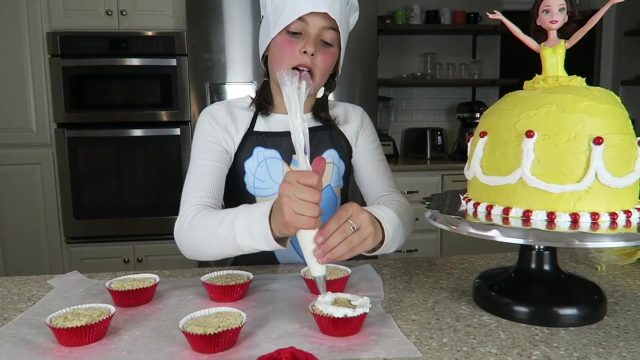 at the bottom of the dress. I'm going to nothing there. candies and the white frosting. wow, this looks so cool. it kind of looks like a candy cane or a Christmas dress. you are probably wondering what we will be using for the little cupcakes here. well, we will be putting a red fondant rose on. 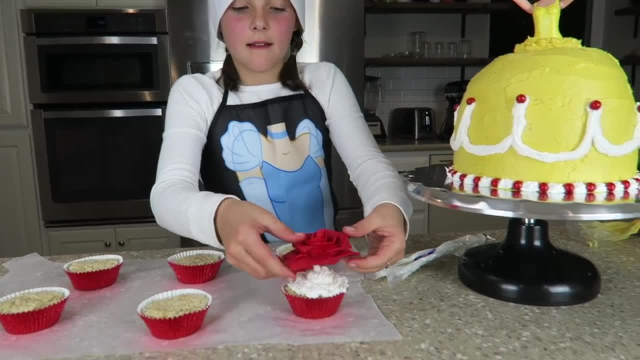 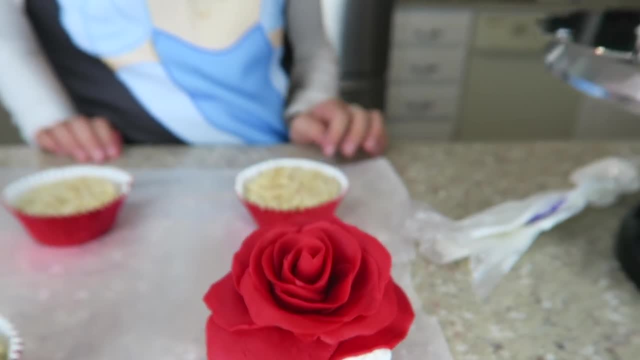 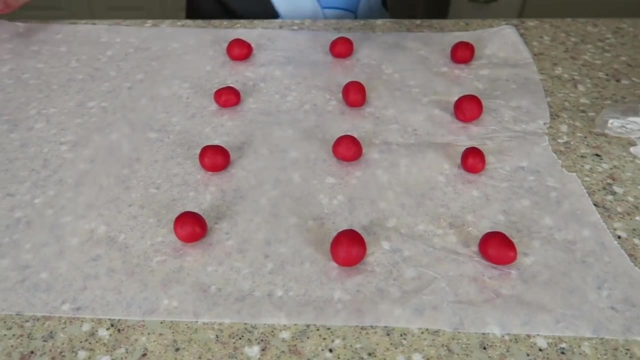 top of it like this. that really looks like a rose, doesn't it? you want to learn how to make them? let's do it. we start with a whole bunch of tiny red balls of fondant, and then we take this wax paper and fold it on top. now we squish each. 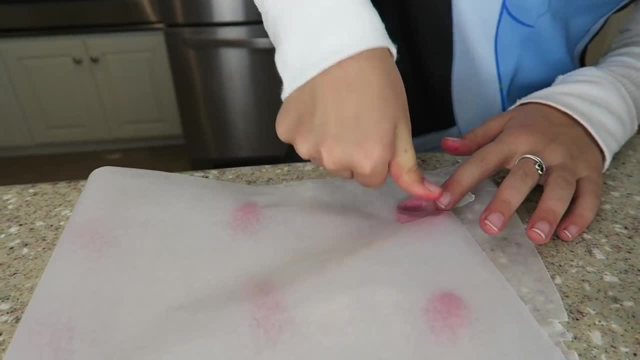 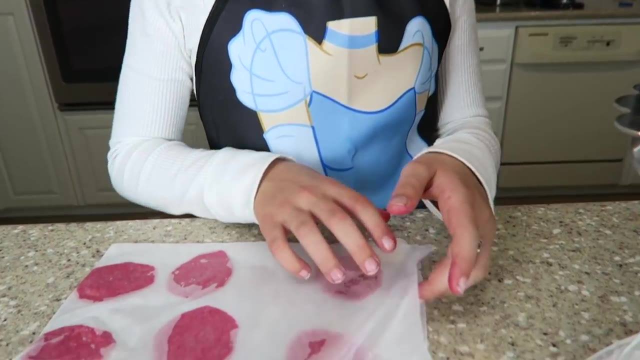 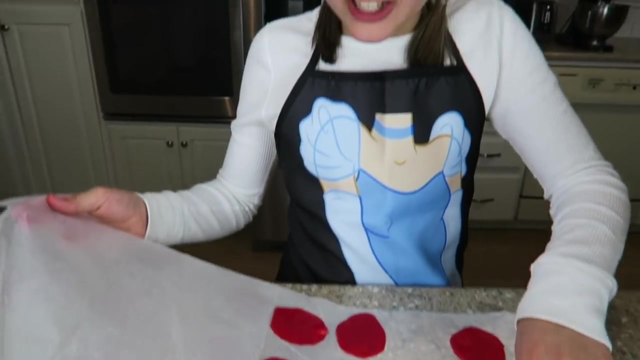 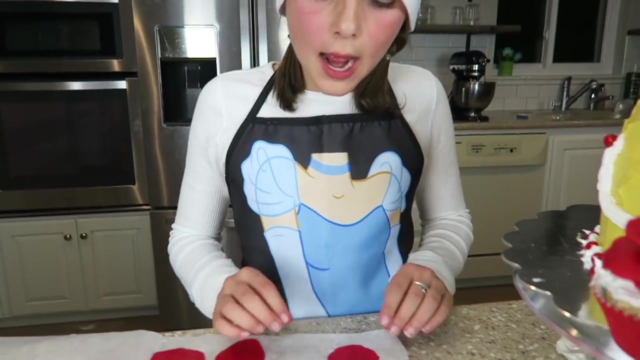 one flat to make the rose petals. now it's carefully. take this off and see what it looks like. oh yeah, these are great rose petals. as you can see on this one, the middle is all curled up, so we're going to take the first one and roll it up. see it, doesn't that look like an? 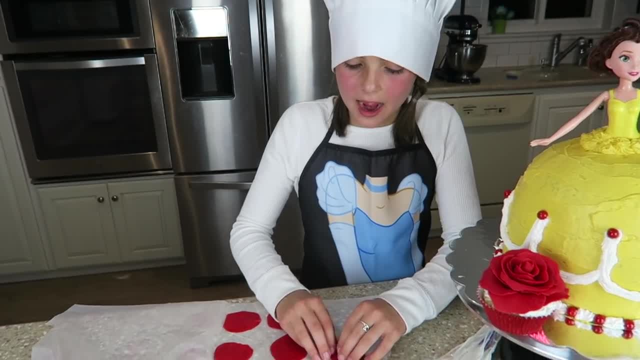 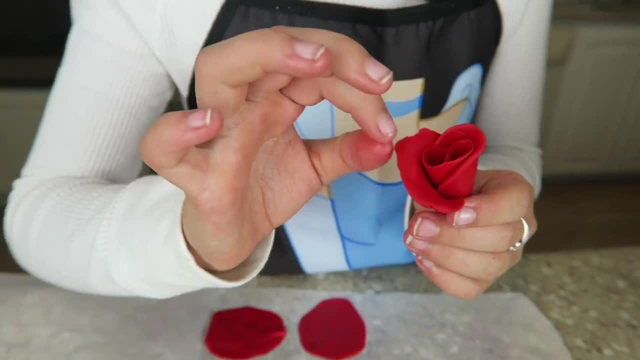 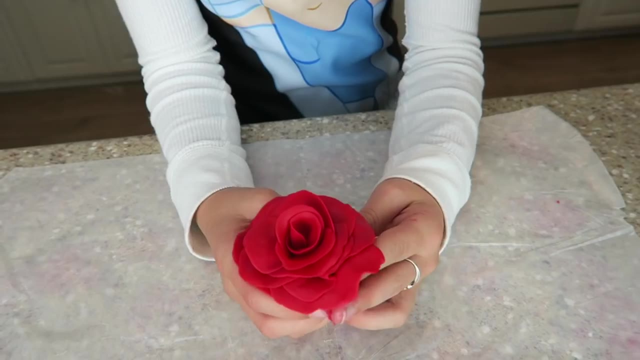 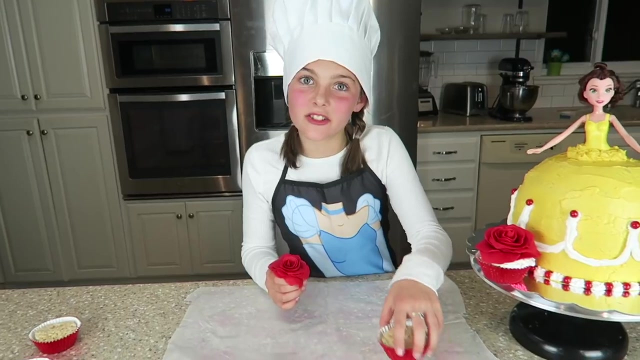 inside of a rose, and now we're just going to add on to it. I'm going to start peeling the edges out so it looks like it's blooming. you just keep staggering them and adding on. whoo, this is pretty. what do you guys think? let's put it on our ice krispy treat. 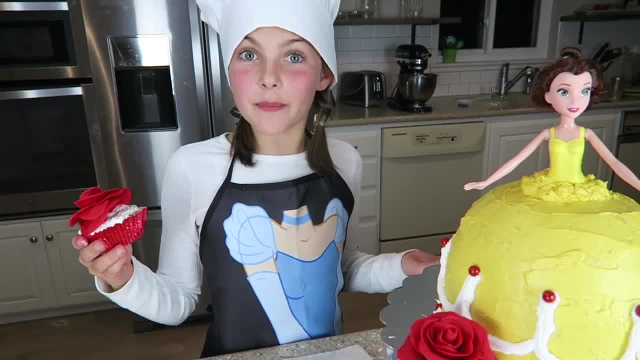 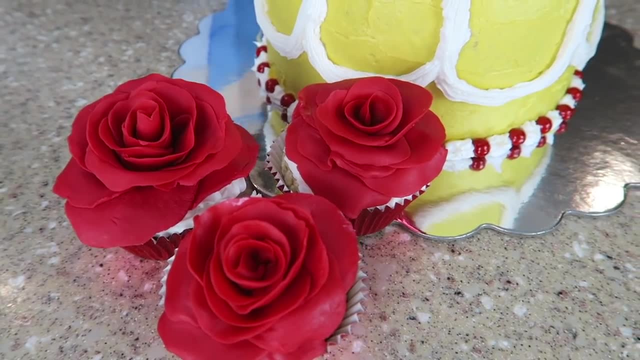 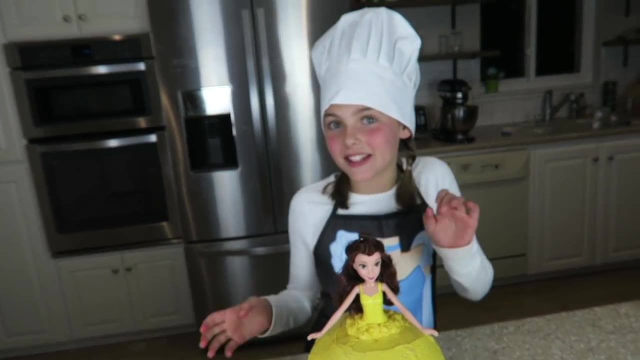 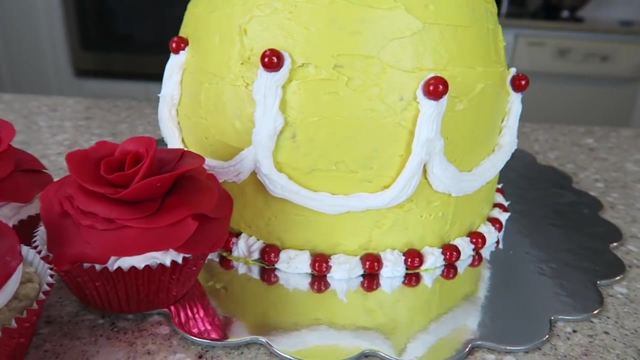 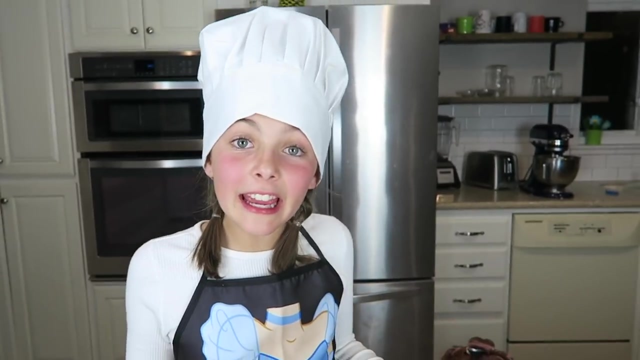 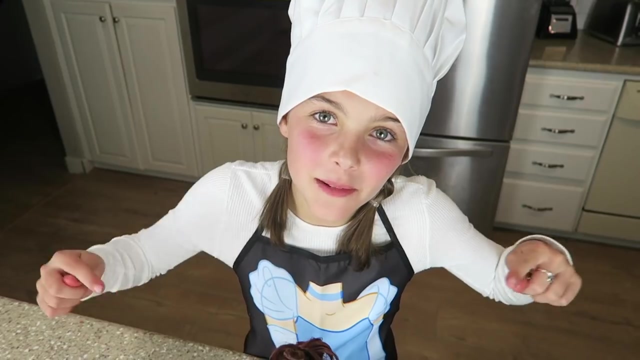 there we go. Beauty and the Beast wouldn't be without the roses. and there you have it. that's how you make a Beauty and the Beast princess bell dress cake made from rice krispies. this is a great cake for birthday parties and any fun occasions. have you guys seen the movie yet? comment down below: oh, I just love these pretty. 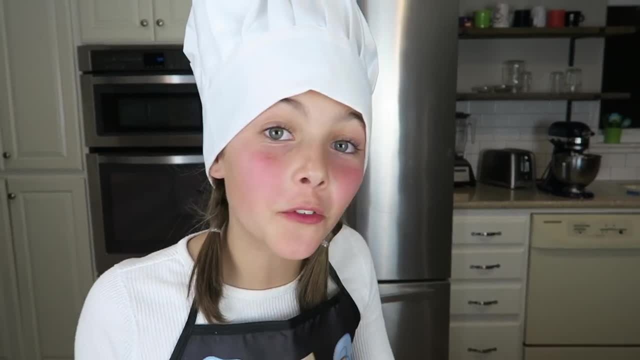 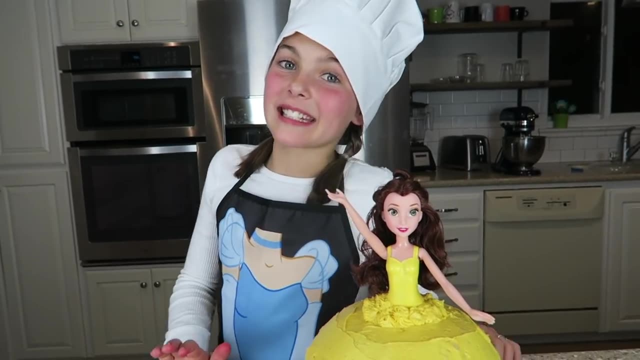 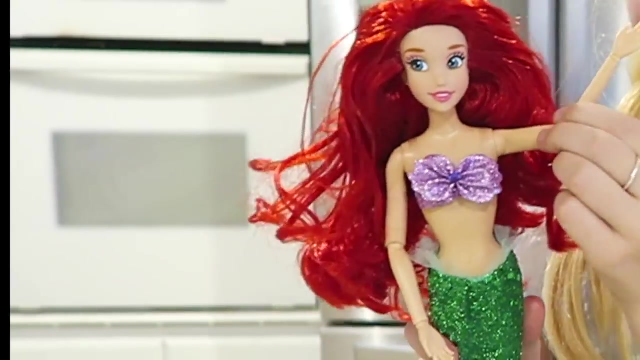 little roses. if you guys make this treat, don't forget to tag us on Instagram or Twitter. we love to see your creations. bye, don't forget to Like, subscribe and comment below. hi, you guys. welcome back to kids cooking and crafts. hey, so today we're going to show you how to make a cute little rose cake. 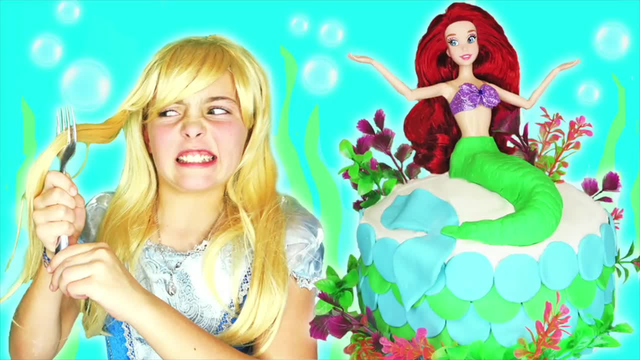 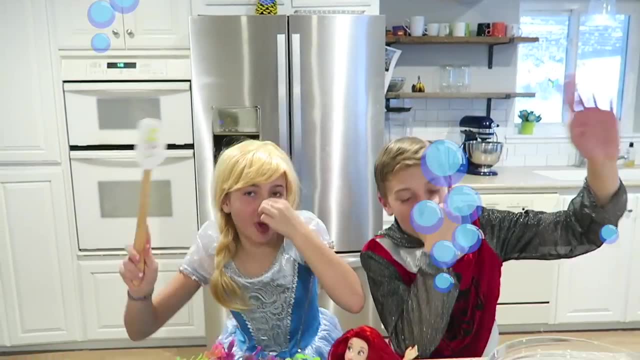 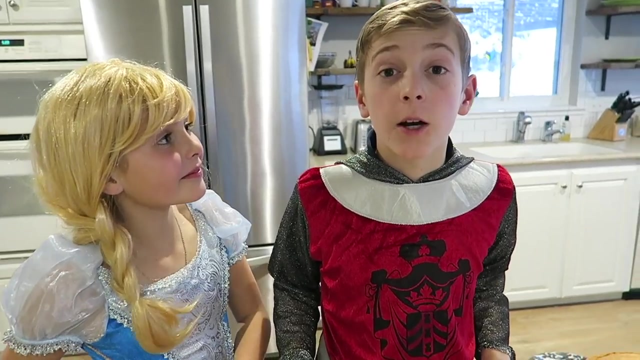 so today we're going to show you how to make a cute little rose cake. so today we're going to show you how to make a cute little rose cake. decorate a Disney princess, Ariel, Little Mermaid ocean cake. it's going to be delicious. let's get messy. let's get messy. first, we're going to stack all of our cakes to. 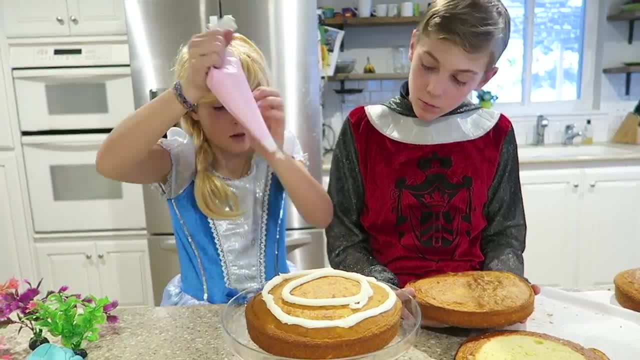 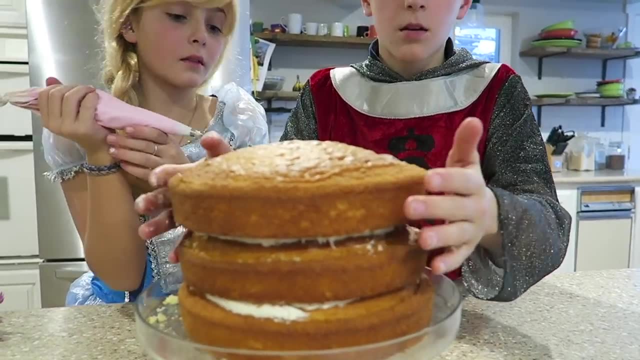 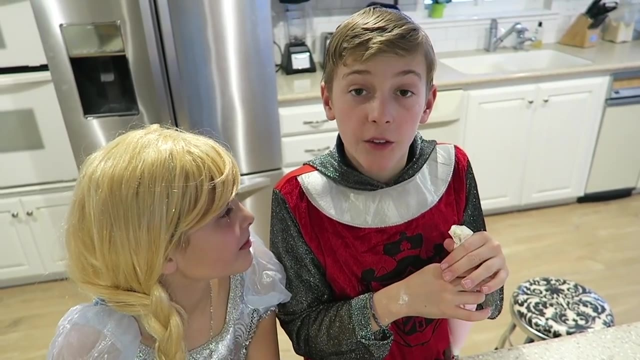 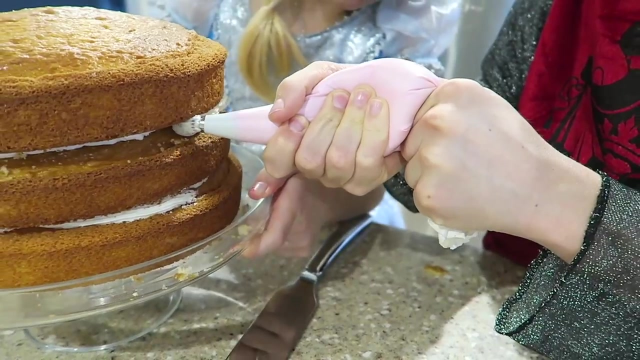 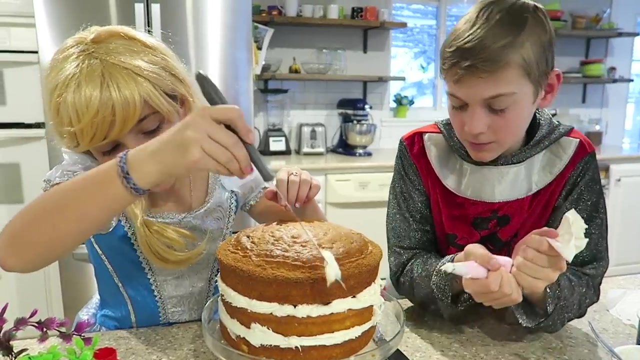 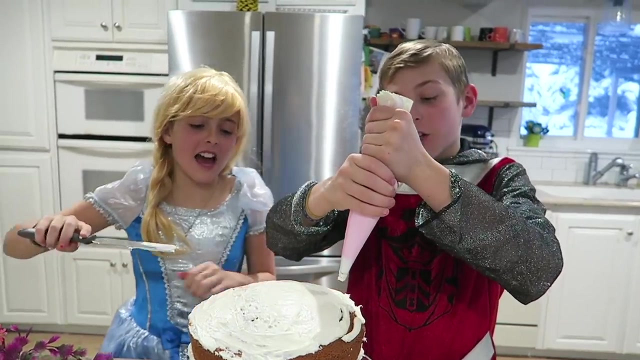 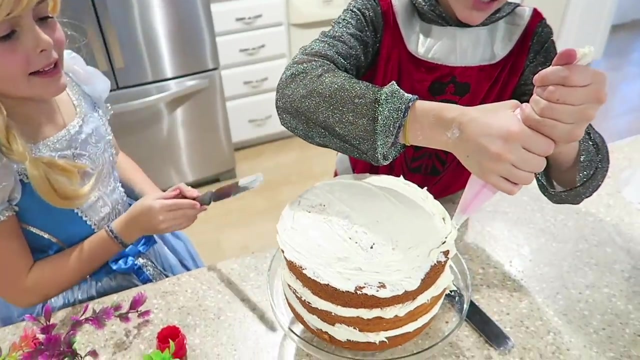 save a little bit of time. we've already made them. now we're going to fill in all the cracks with frost. I'm gonna, princess Ava, spin it while I decorate. now we're gonna decorate the top Under the Sea. Under the Sea, Darling, it's better down where it's wetter. take it from me. 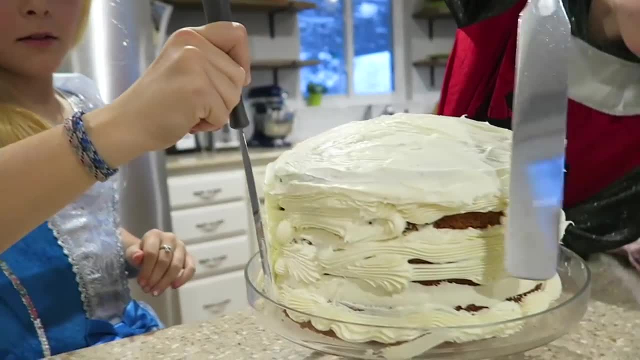 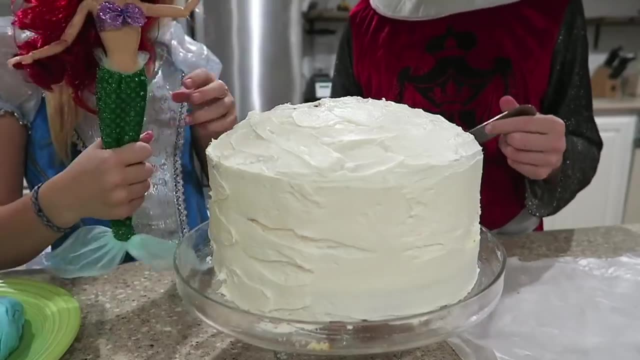 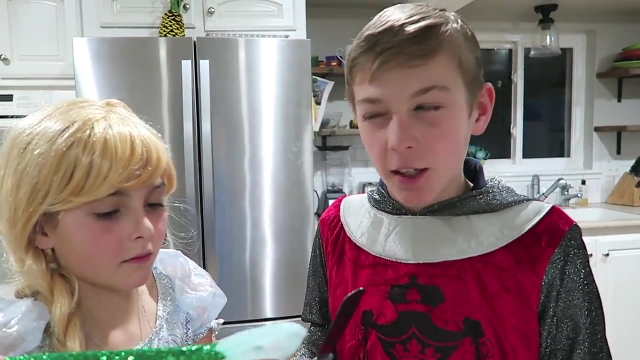 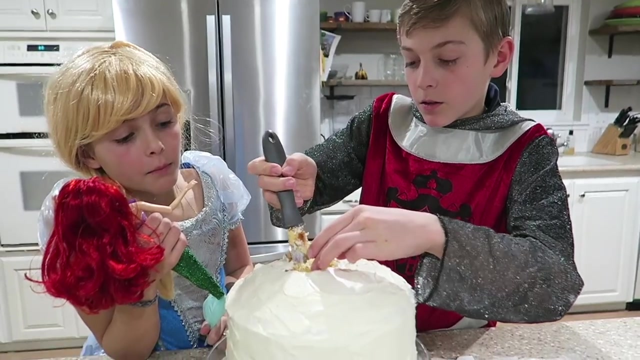 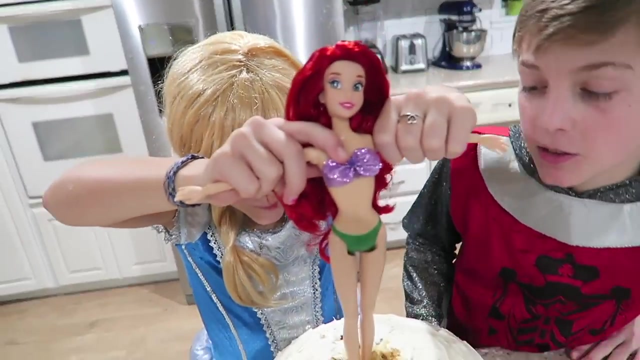 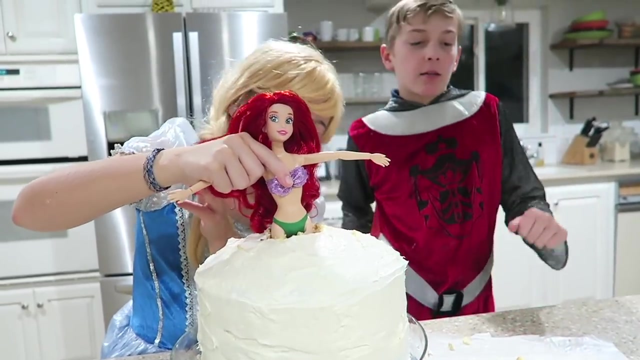 Now I'm just going to smooth it all out. Now we're actually going to put Ariel into the cave. Let's cut a hole out for her legs, I mean for her tail. All completed, Let's put it in. Yes, we did it. 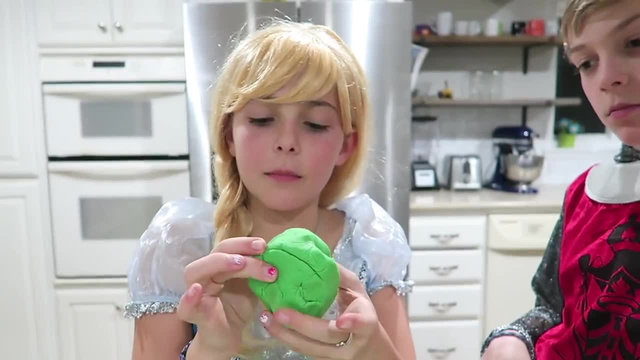 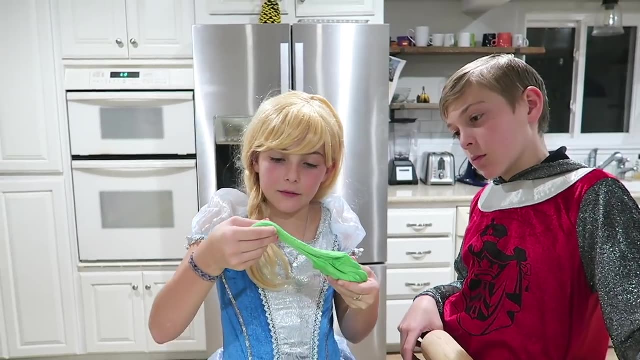 Alright, so we're going to use this fondant stuff. It's like a marshmallow-y play-doh stuff that you can eat. It's easy to form into stuff. It's stretchy. You can technically make anything out of this. 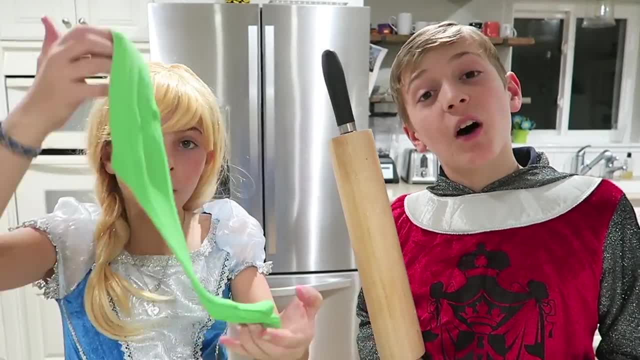 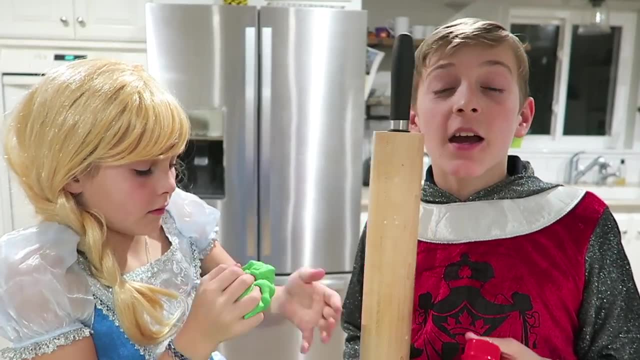 It's like edible play-doh. Now we're going to roll out all of our fondant with a rolling pin And we're going to use our little cookie cutter And we're going to make a whole bunch of little tiny circles And make them the fish scale. 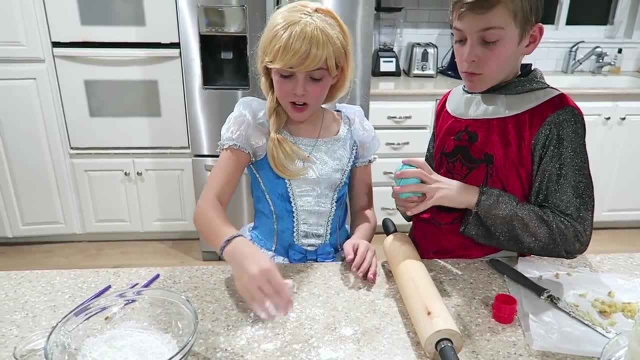 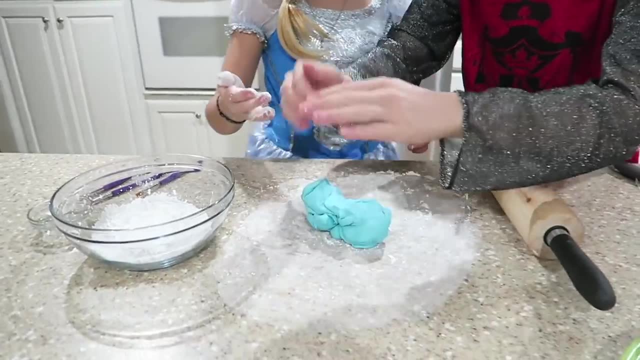 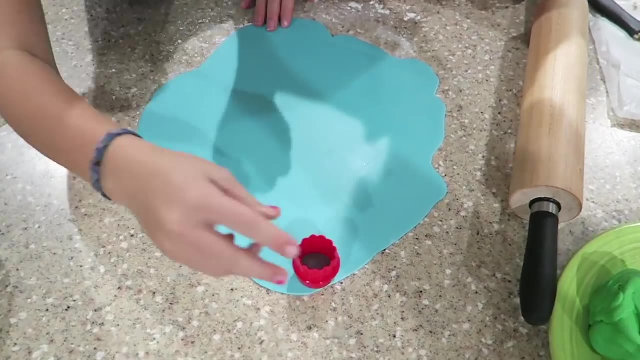 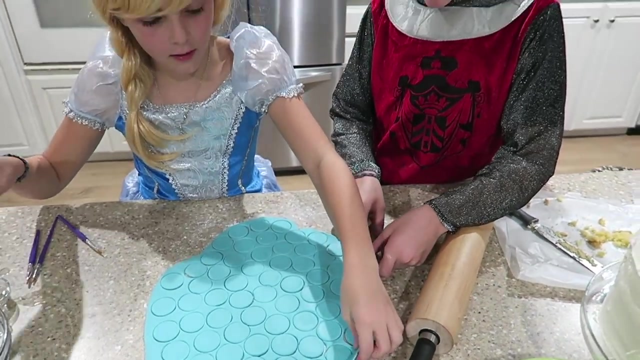 Let's get to it. Let's put a little powdered sugar, That way it won't stick. We want it nice and flat, so we can make as many as possible. Let's start cutting Last one There. nice, Alrighty, let's take this out. 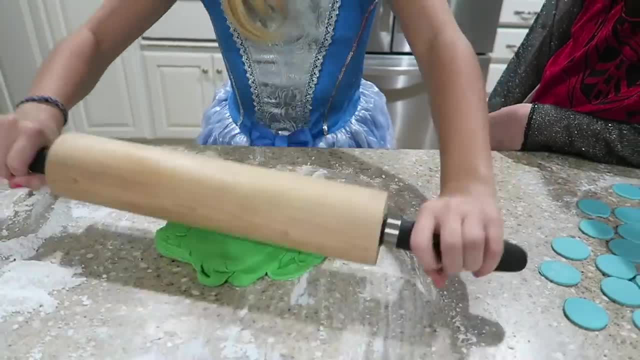 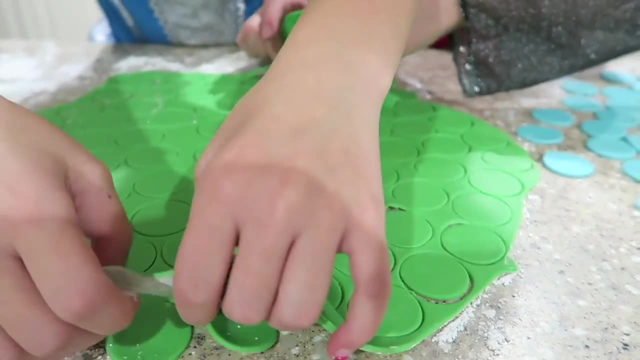 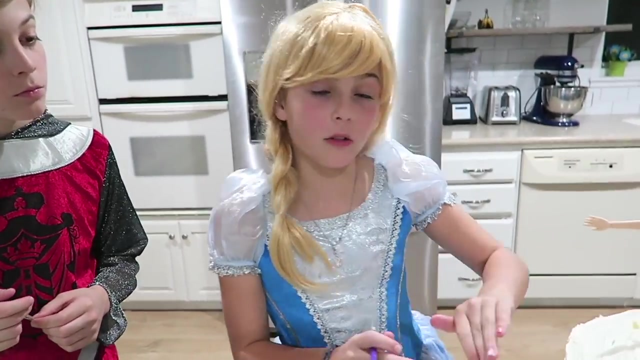 Now we're going to do the green. Yes, we're done. Alrighty, Let's peel it off. Now we're going to put the scales on the cake. We're going to start with a layer of blue around the bottom To help the scales stick better. I'm going to add a bit of water onto the back. 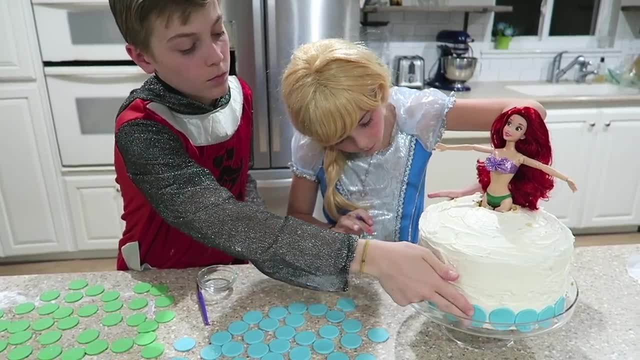 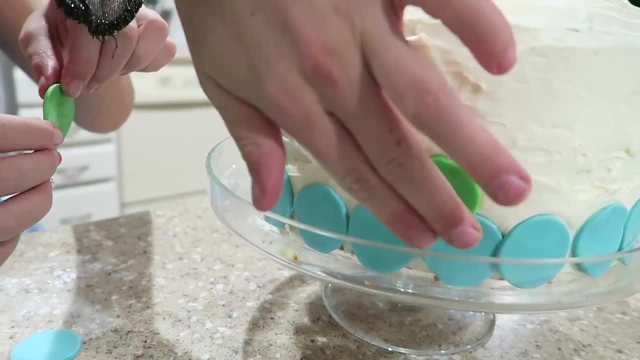 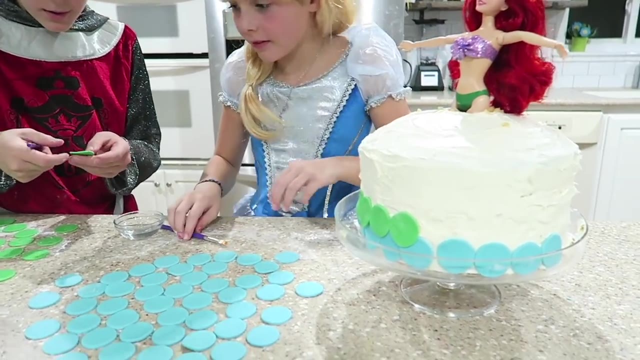 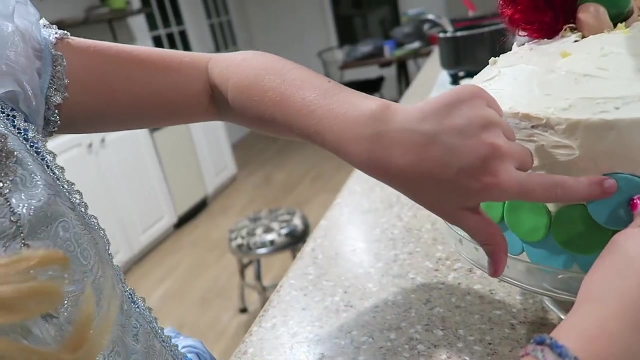 Do-do-do-do. Now we're going to do our greens. You want to stack them right in the middle of these blues. Layer number three: This is when it really starts to look like mermaid scales. Whoa, What I'm so excited to see what it looks like. 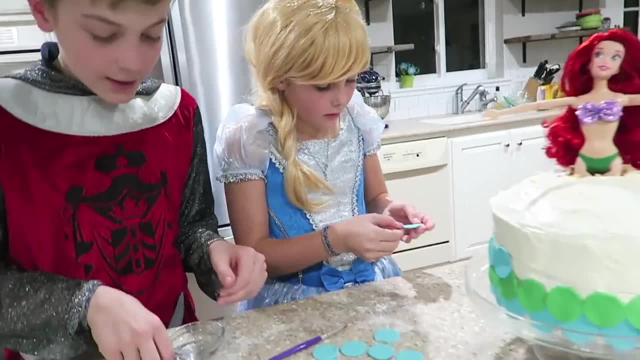 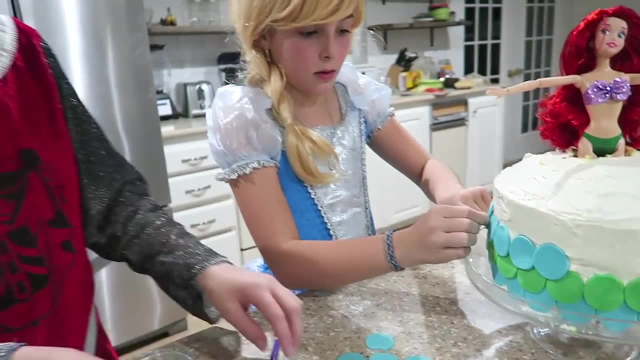 Thanks, That's what it looks like when we're all done. I know right, It's like the coolest thing ever. Yeah, I've made some other cake videos with fondant in them, like the Rapunzel cake. Yeah, we had to cut off her hair. 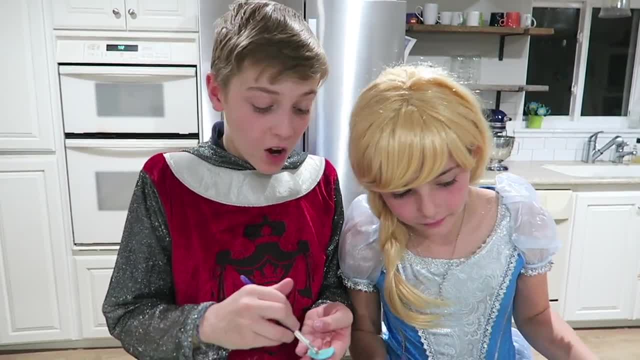 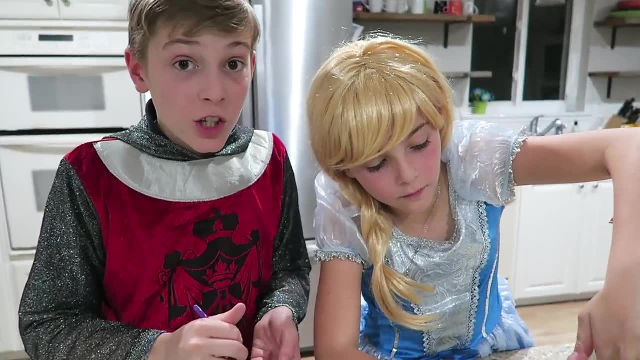 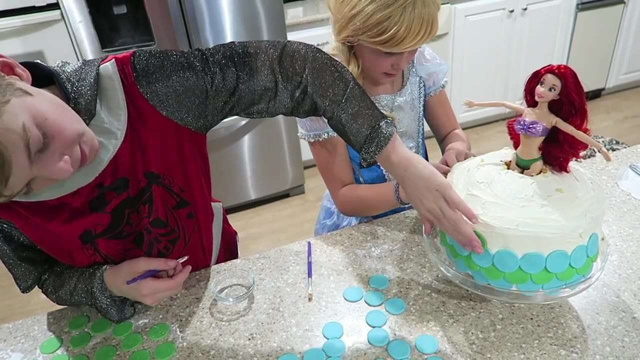 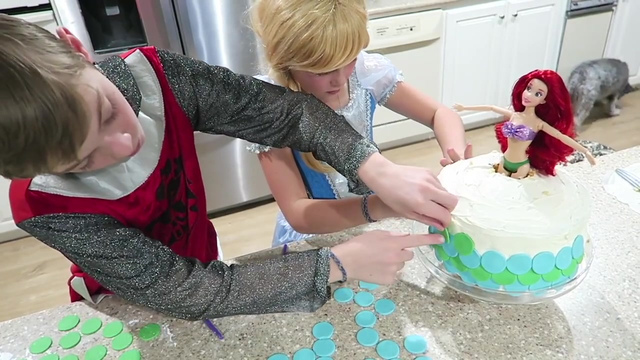 It was kind of sad. We used the same fondant making her hair. It was just yellow fondant. You guys should go and check that video out too. when we're done, Layer number four, Last layer, Let's get to it. 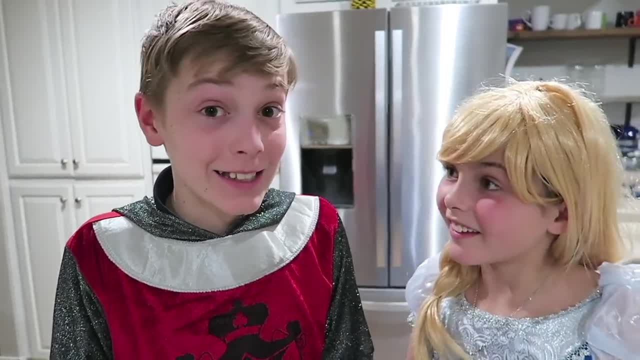 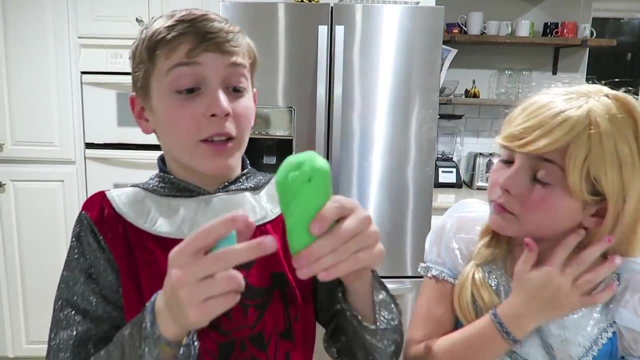 This is so cool. I think we should make a dragon cake next. What do you guys think? I'll finish with the mermaid scales Now. let's make her tail Now. we're gonna make her tail with the leftover fondant, All right? 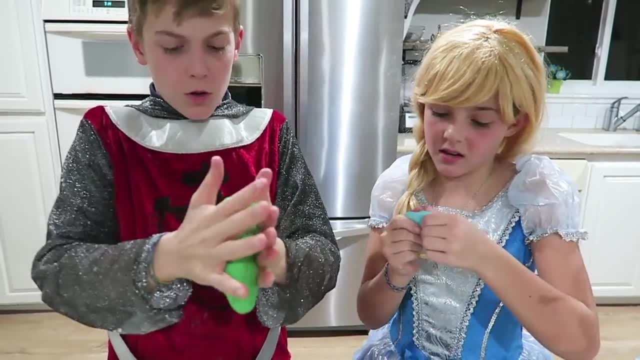 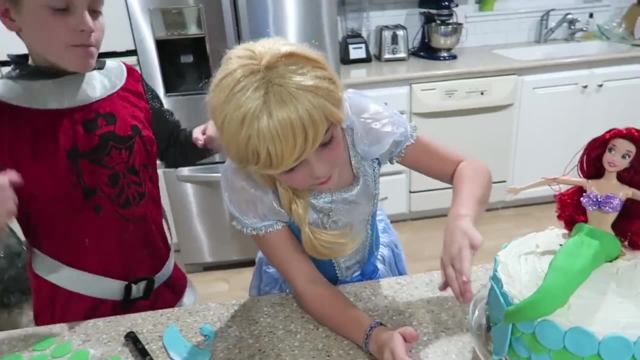 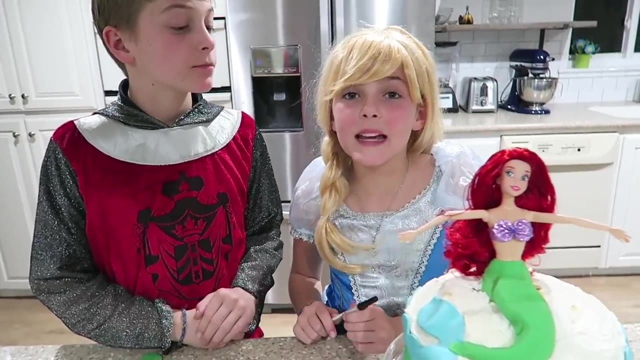 So you have the blue and we'll have the green here. This is good. Now just form it into a mermaid tail like this. Okay, that's good. Booyah, Now to make the scales on her fin. we're gonna take a pen cap, not the pen the pen cap. 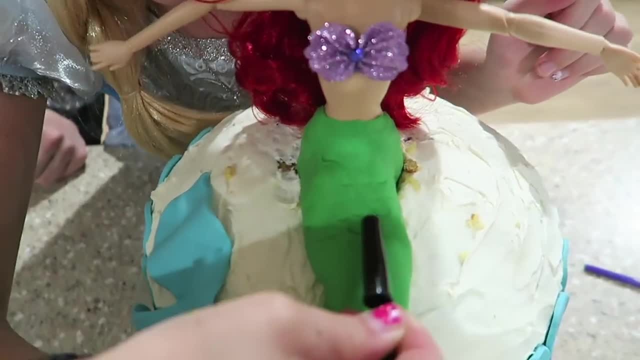 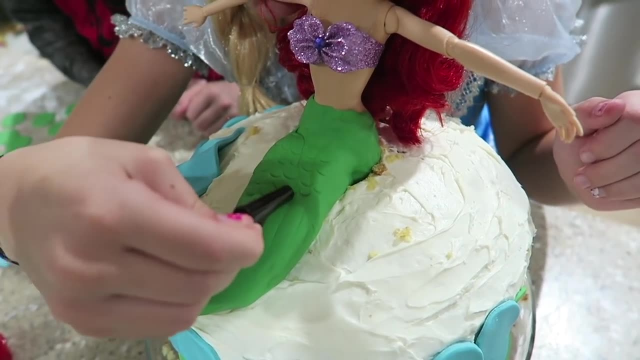 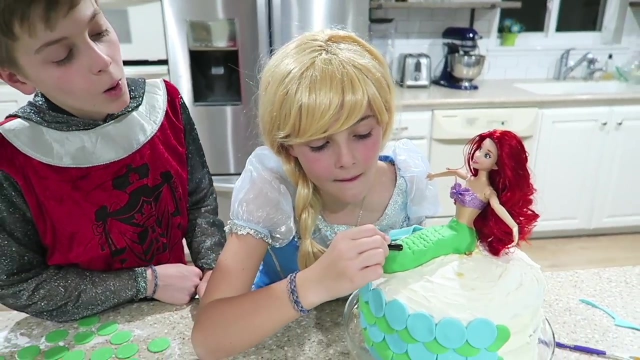 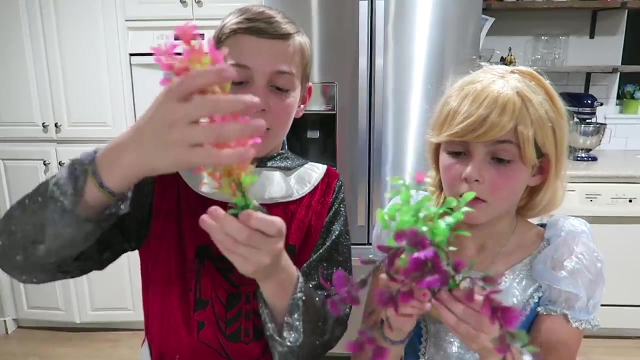 And we're gonna tilt it sideways and put it just just like this. That looks good, Thank you. This is gonna look so cool. Wow, Now for the finishing touch. These are fake fish tank plants. Now we're gonna use them on our cake. 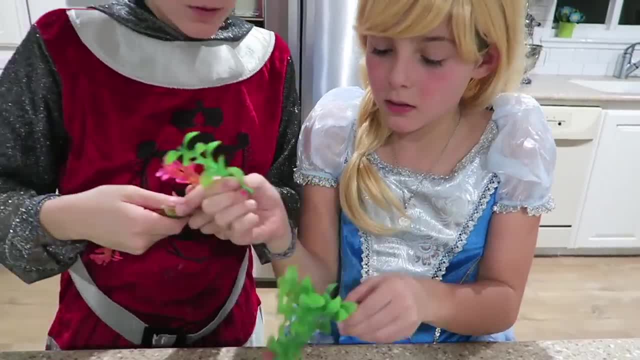 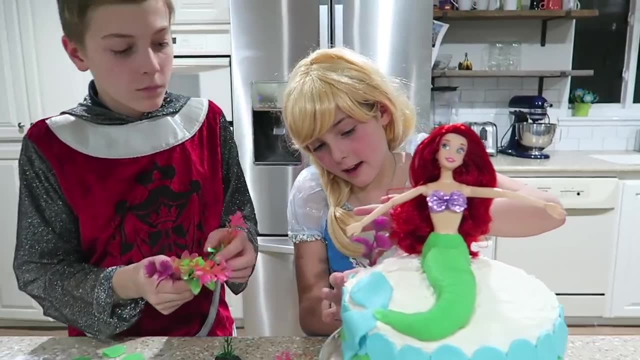 So let's pull them off. So I'm gonna add a little bit of green ones, So okay, and then just like some red and purple. This one's on the side, All right, so I'm gonna go on this side, right here. 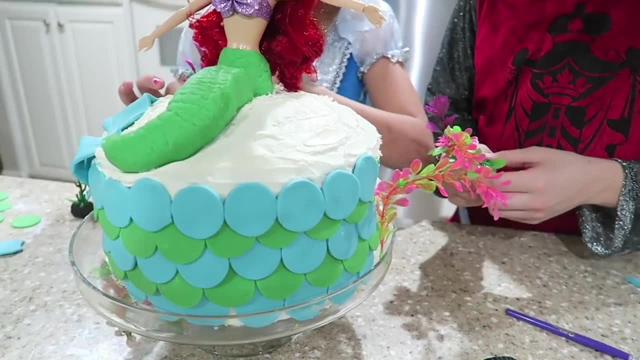 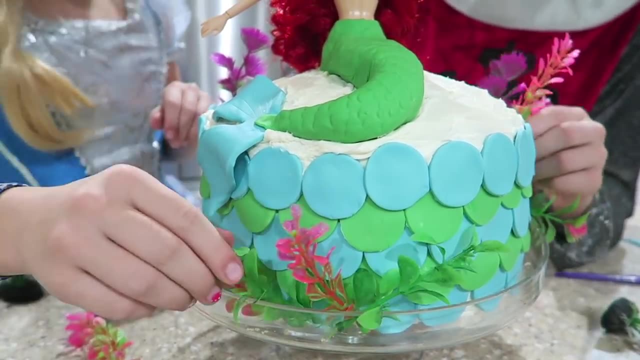 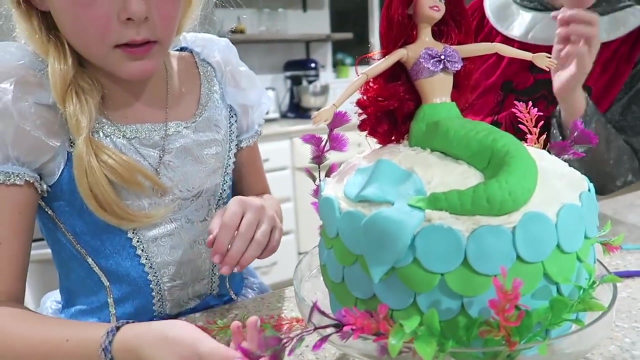 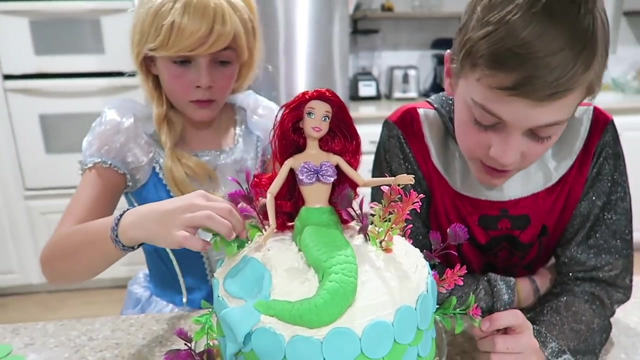 Just like stick it in, And then I'm gonna get another green one. I need some purple over here Down, And then I'm gonna put purple on the edge. Oh, this looks good. What do you guys think? Is it pretty cool? 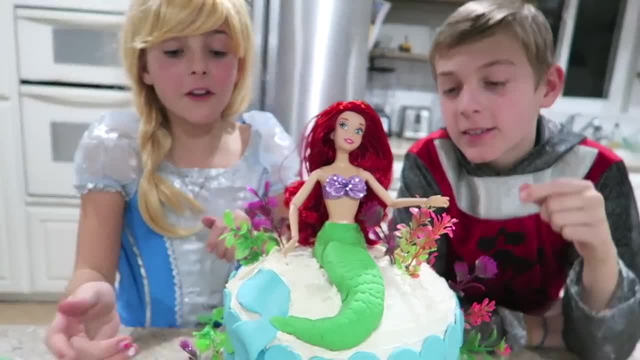 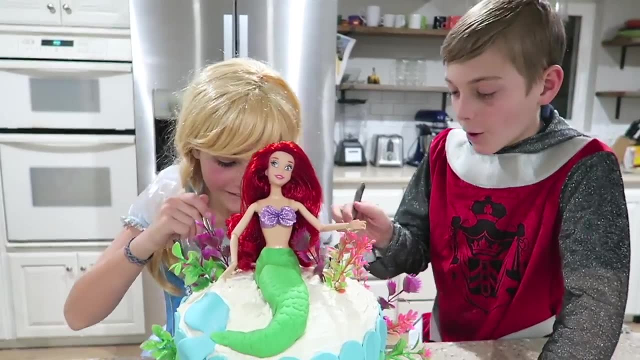 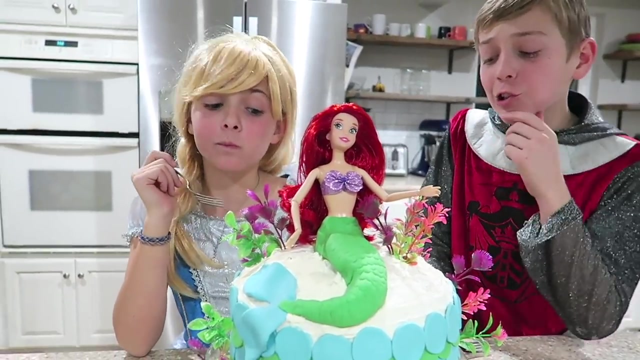 I like these purple flowers. My favorite ones are like the pink and green ones. Oh yeah, the tall ones. Yeah, Now let's take a bite, All right, Mmm, Mmm, That's really good, That's a good cake. 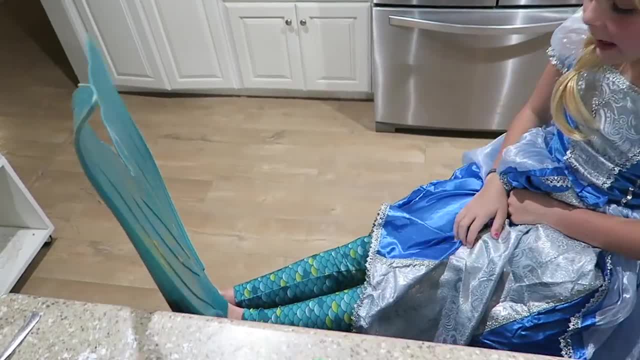 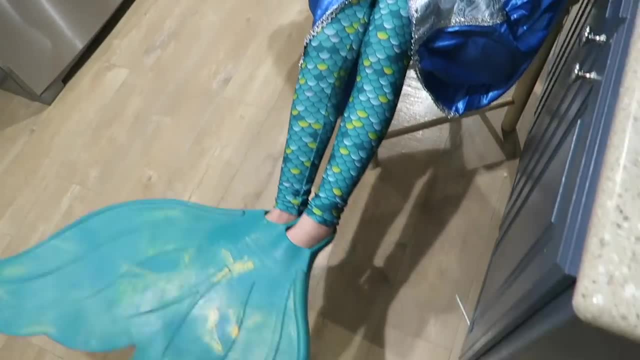 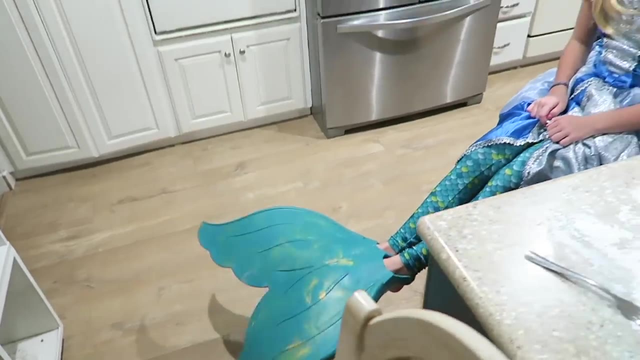 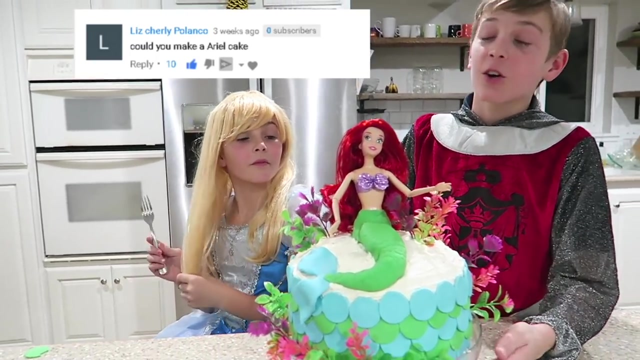 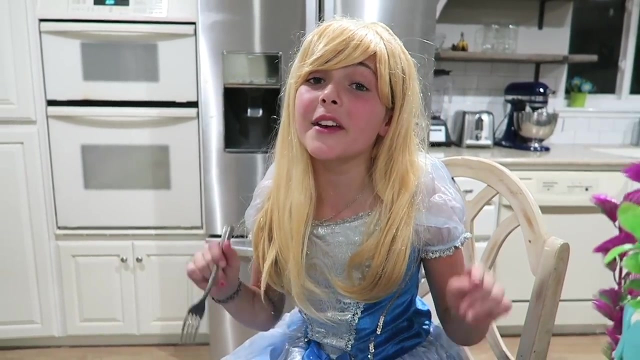 What, What? I have a tail. It's kind of cool. Now I know how Ariel feels. A big shout out to Liz Polanco for giving us this great idea for this little mermaid ocean cake. If you have any other awesome ideas for kids cooking crafts, let us know in the comments down below. 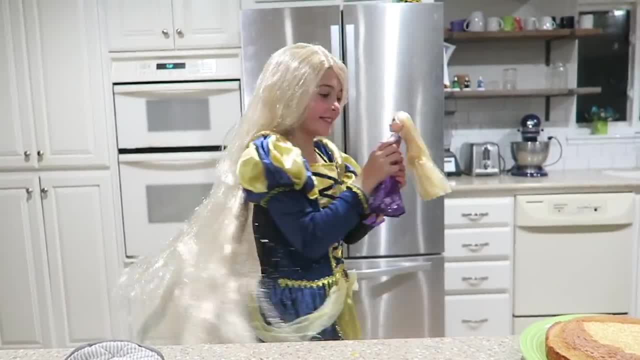 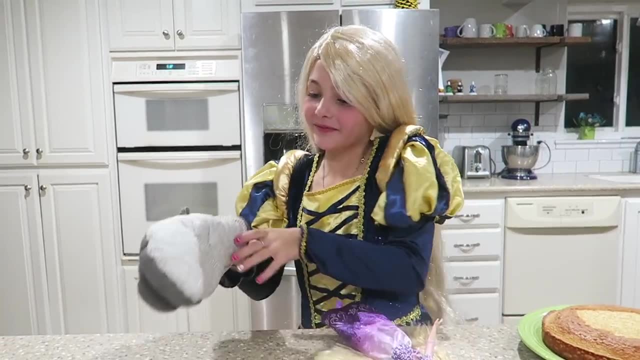 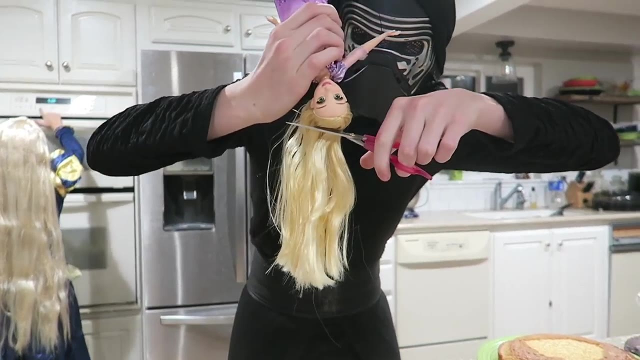 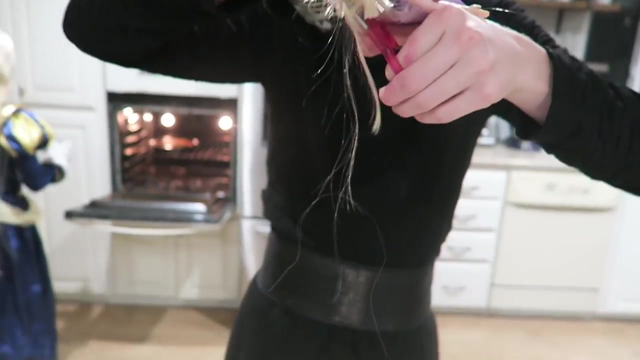 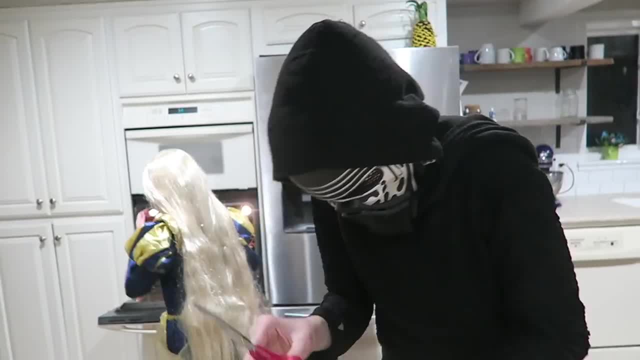 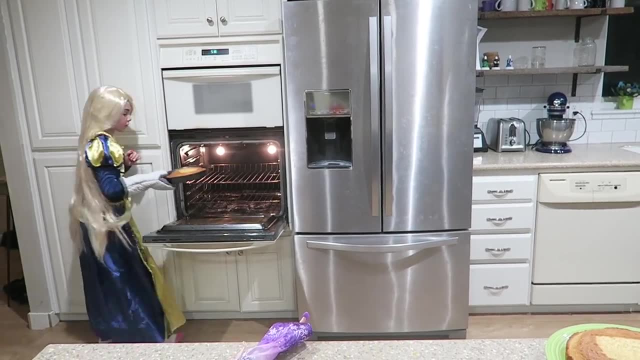 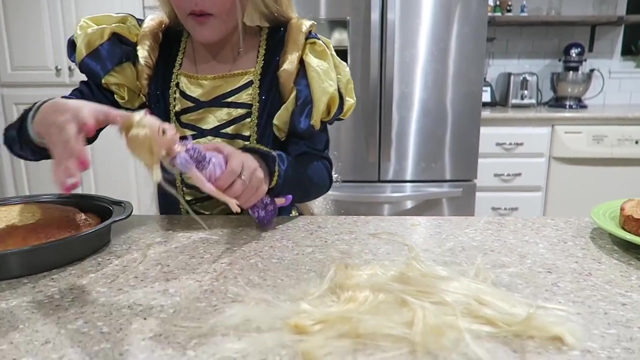 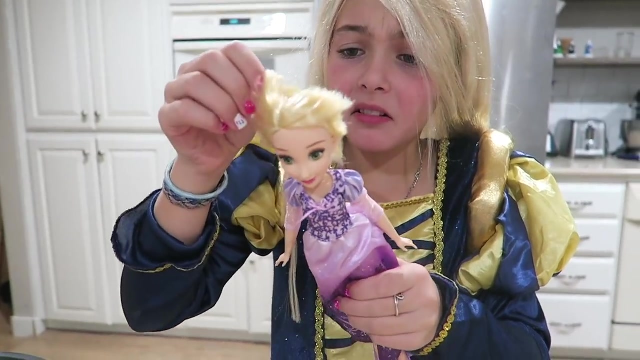 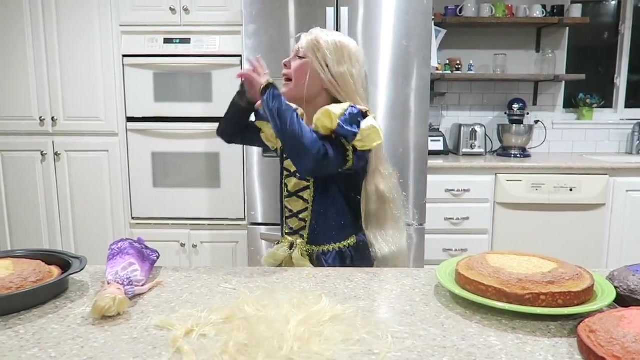 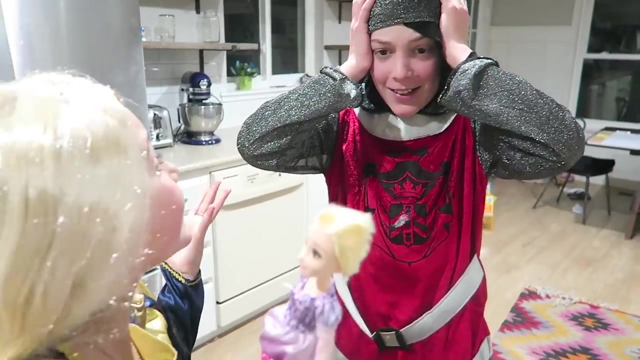 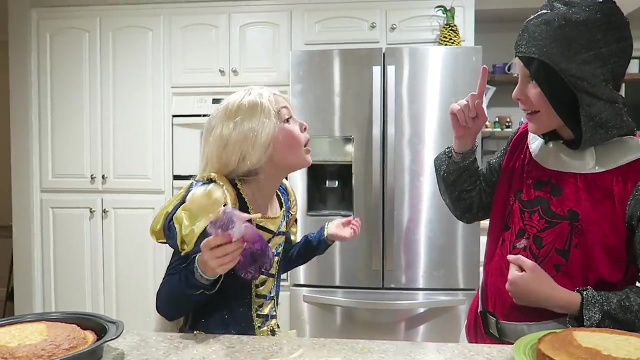 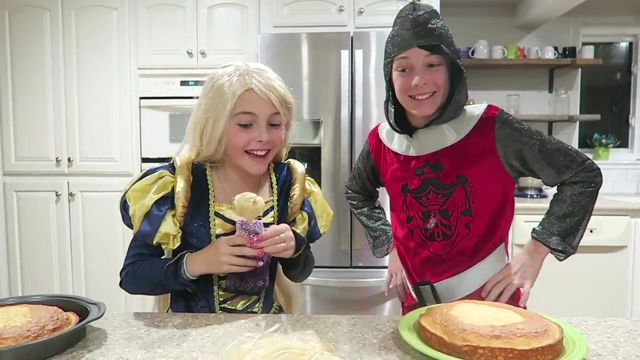 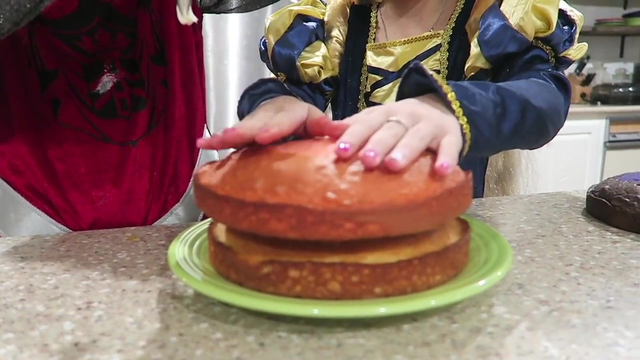 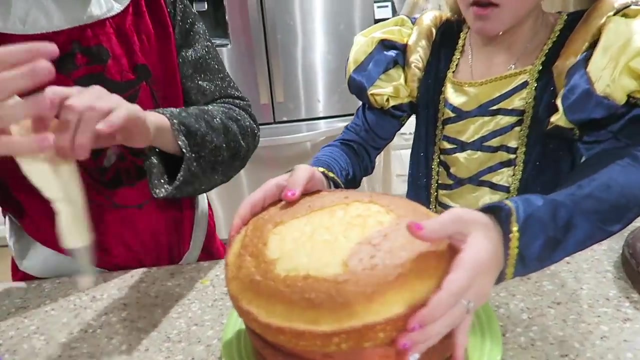 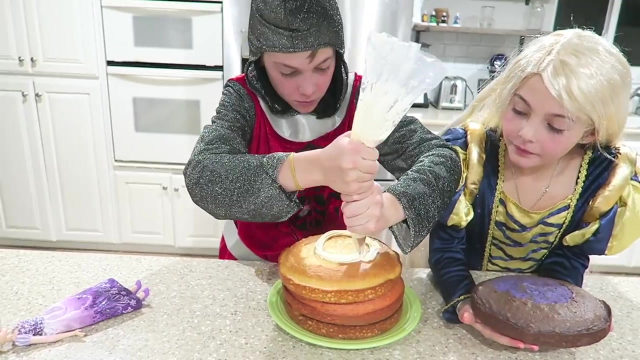 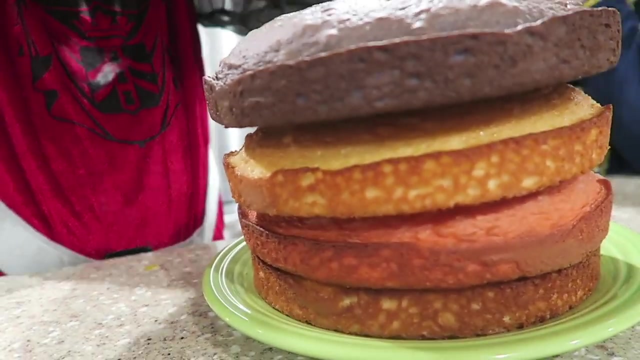 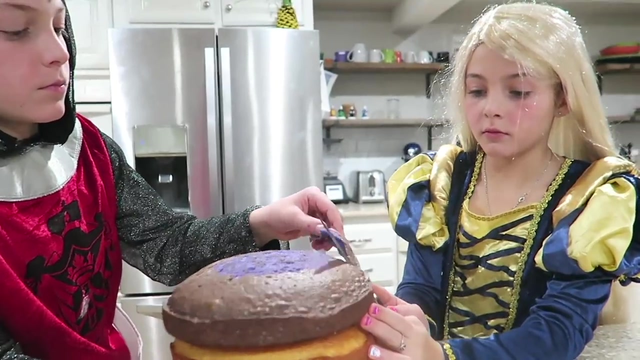 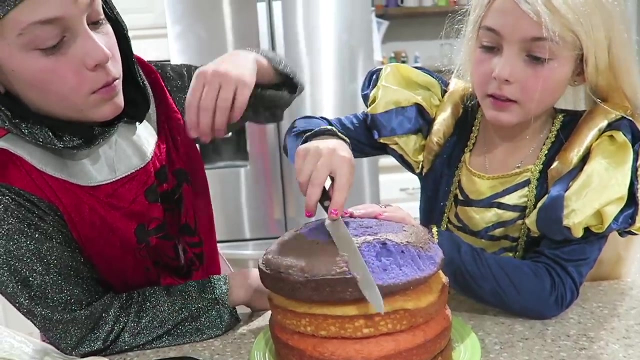 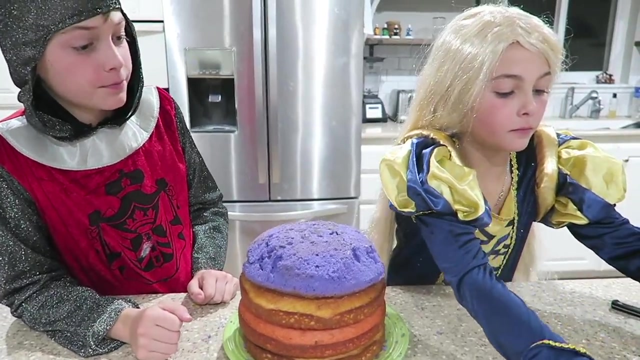 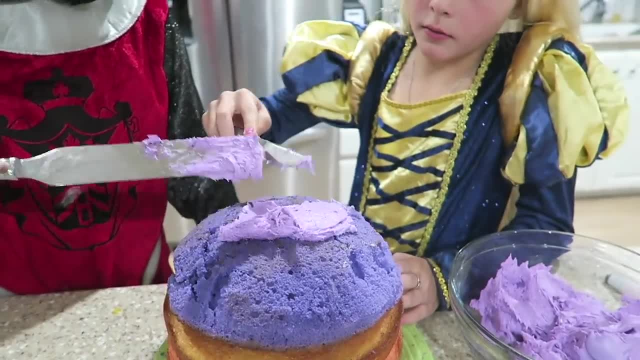 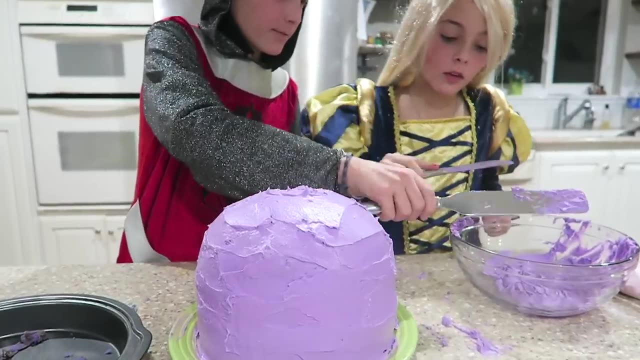 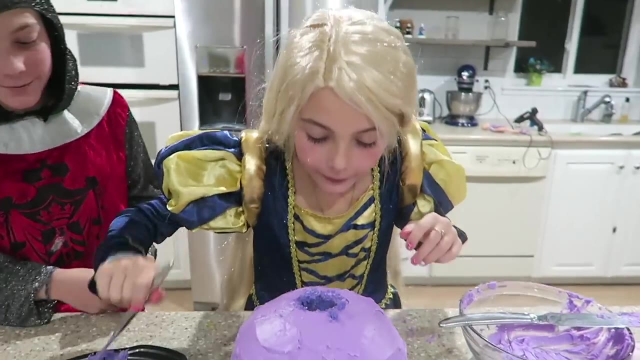 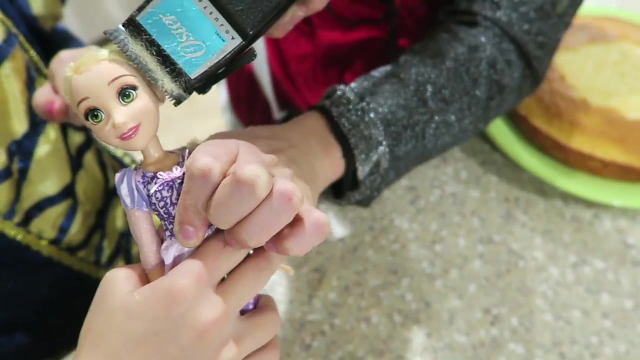 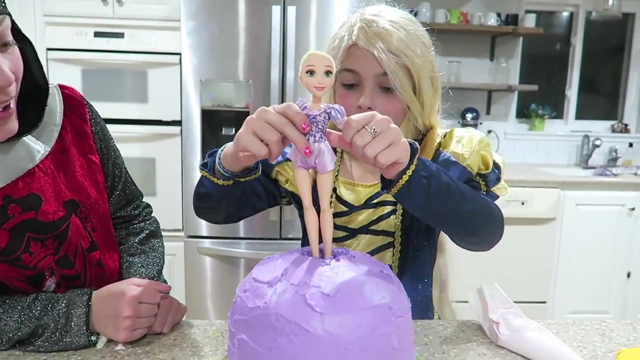 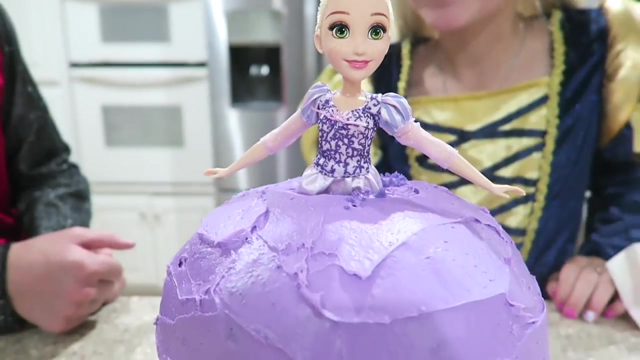 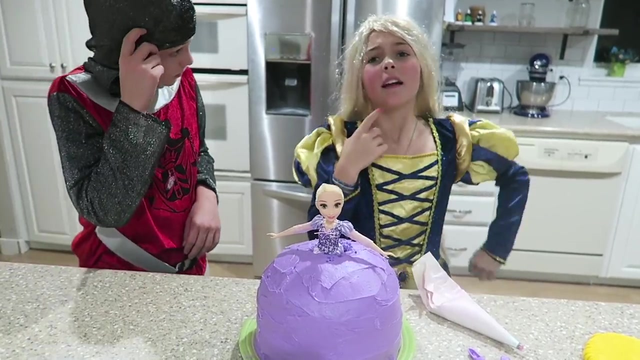 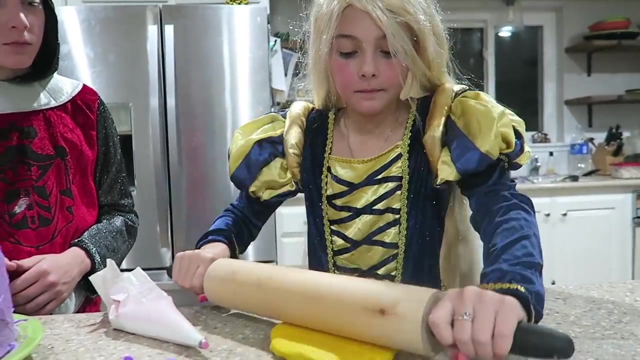 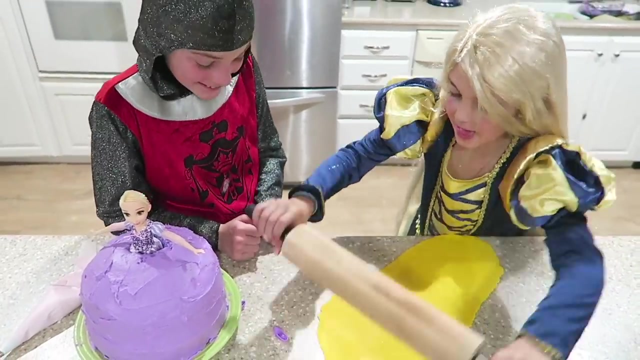 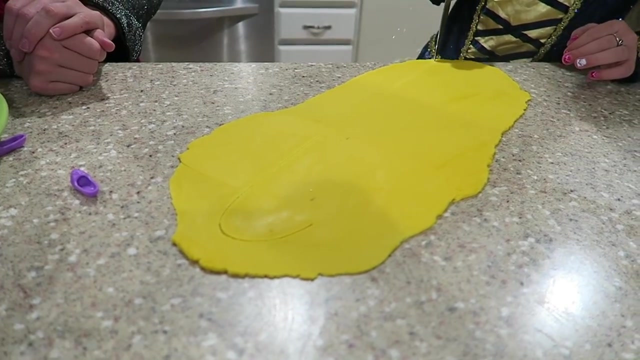 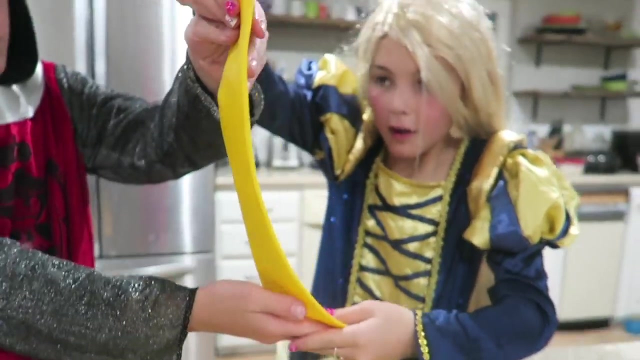 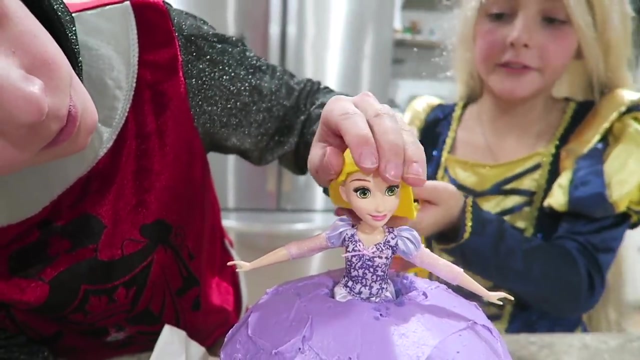 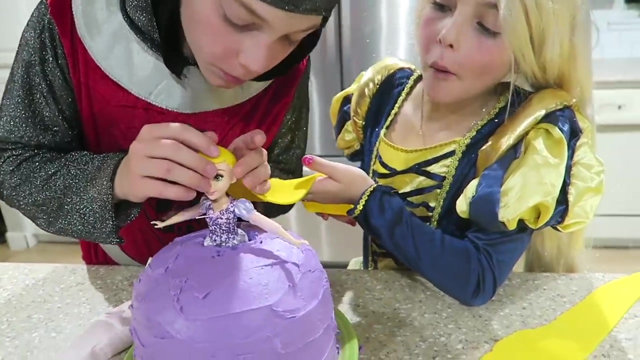 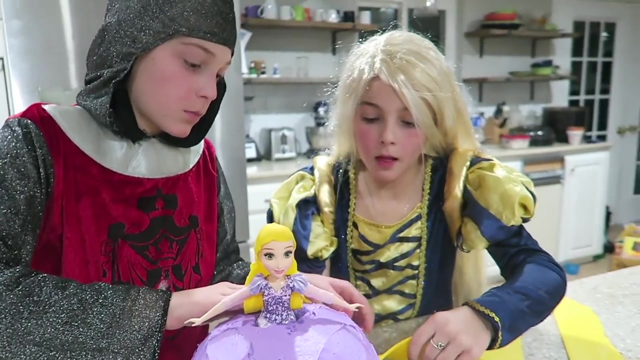 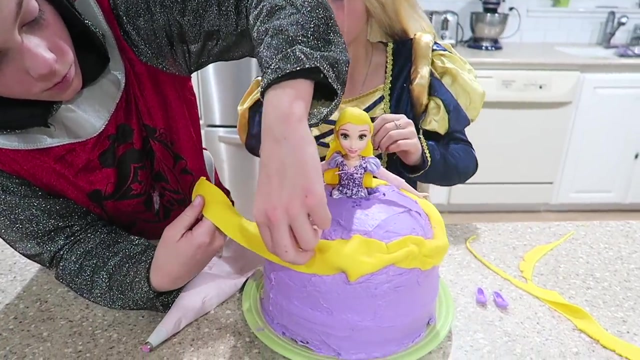 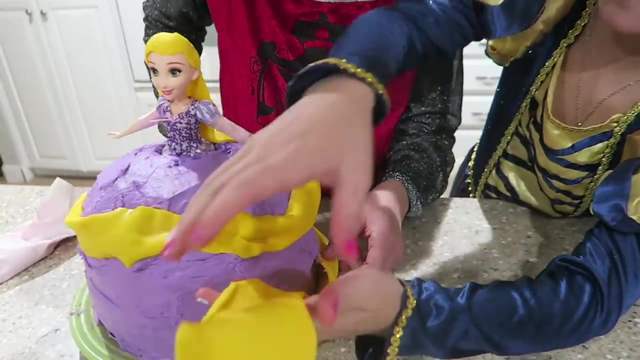 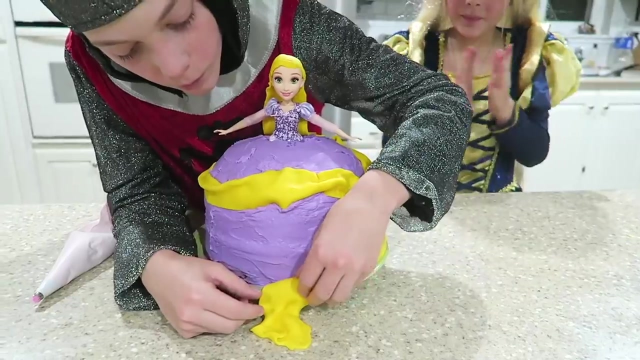 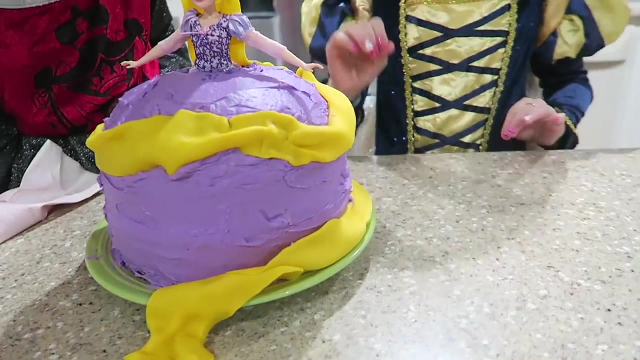 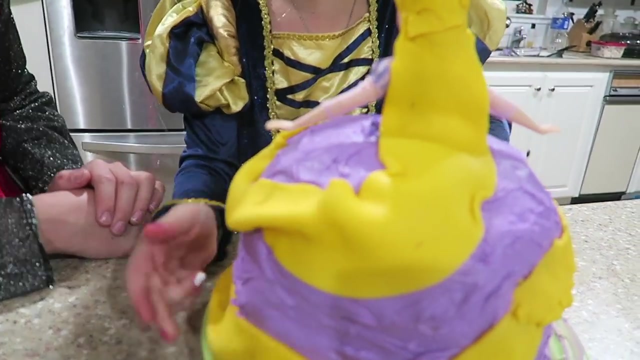 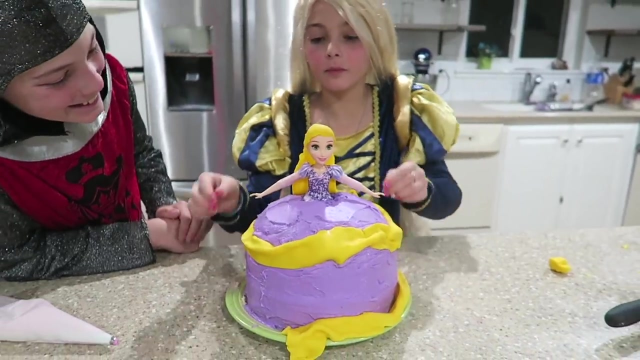 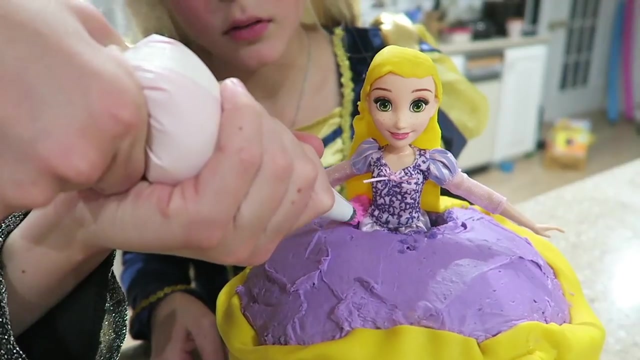 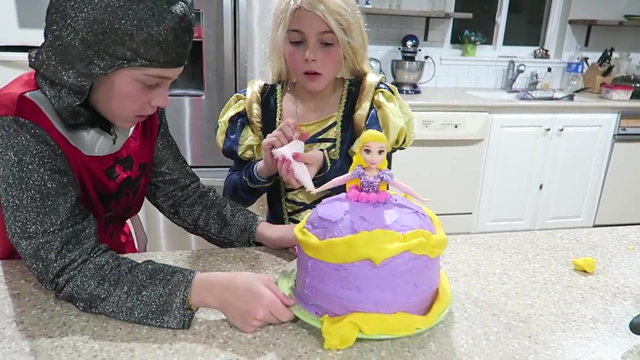 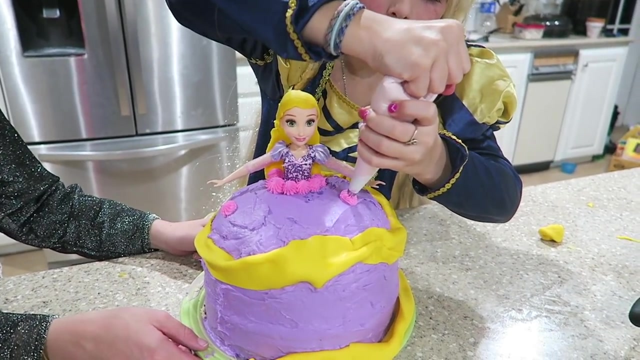 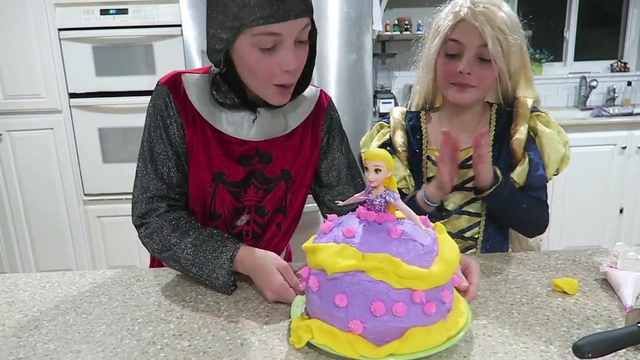 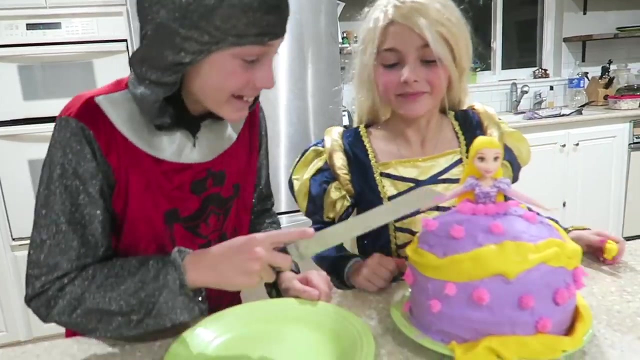 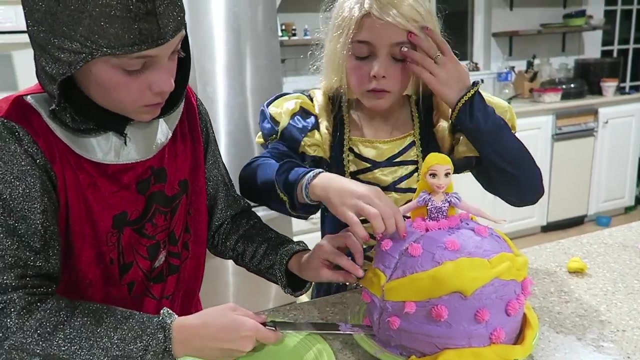 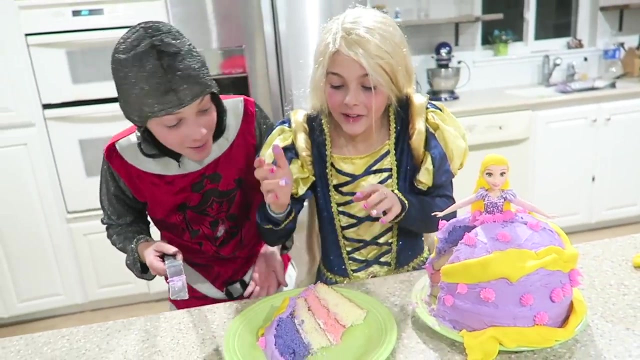 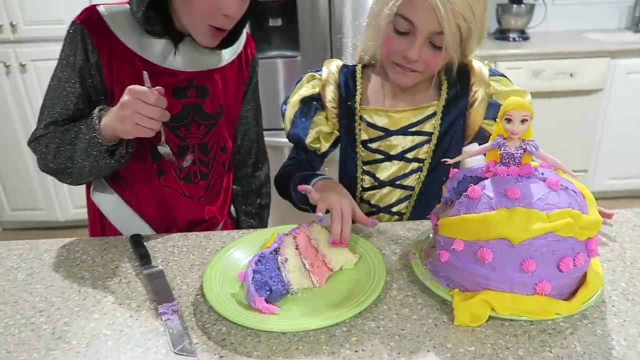 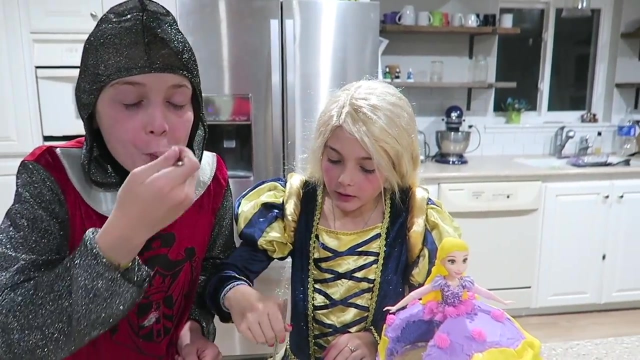 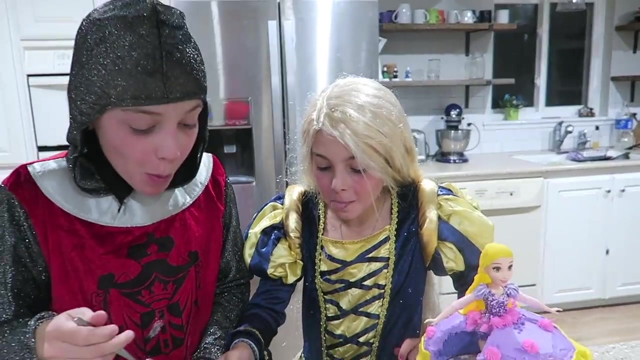 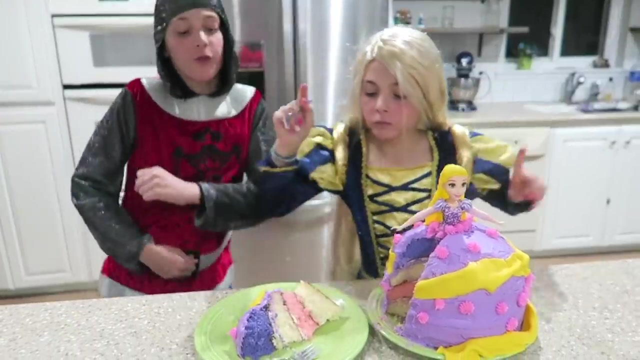 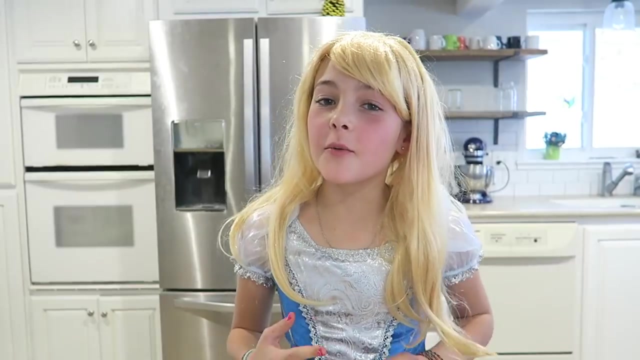 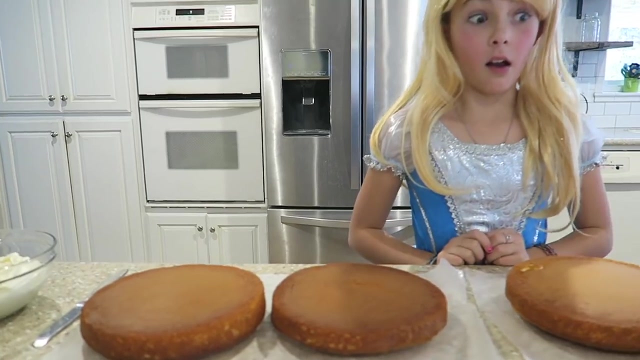 Bye-bye, Bye-bye, Bye-bye, Bye-bye, Bye-bye, Bye-bye, Bye-bye. Today we'll be making an eight-layer sleeping beauty cake. That's a lot of cake. Oh, and this is Prince Charming. 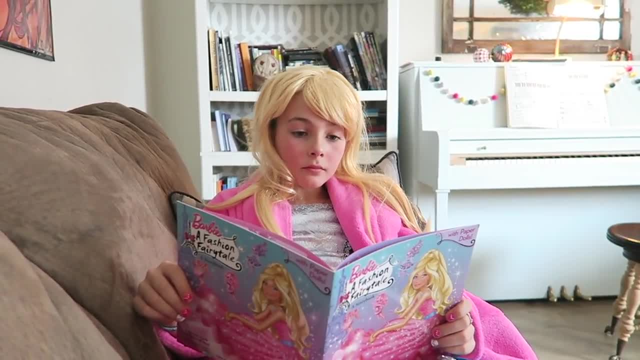 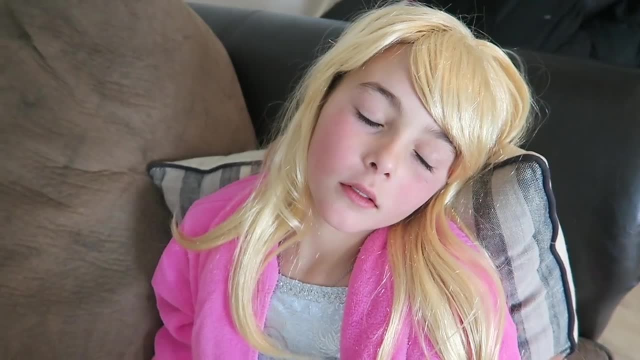 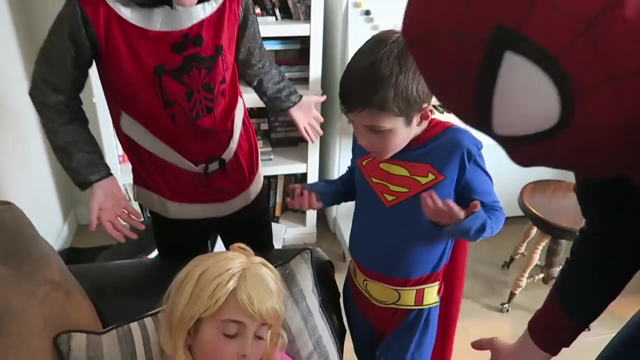 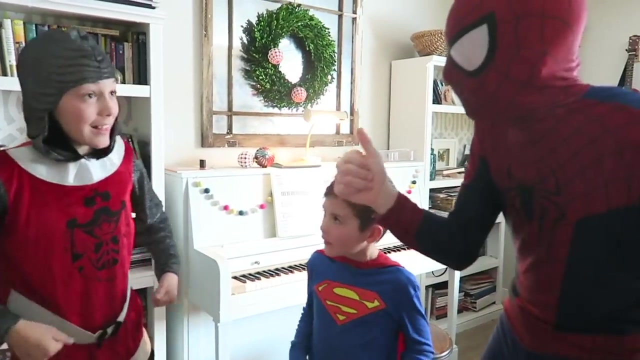 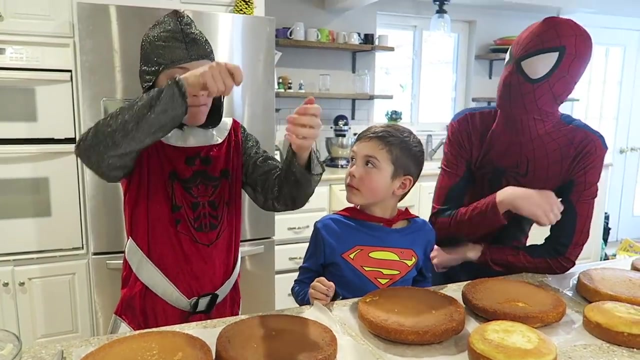 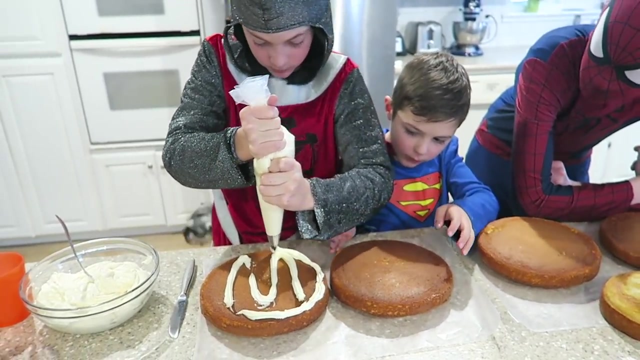 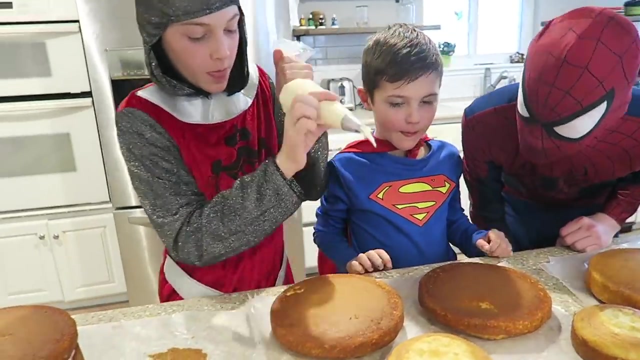 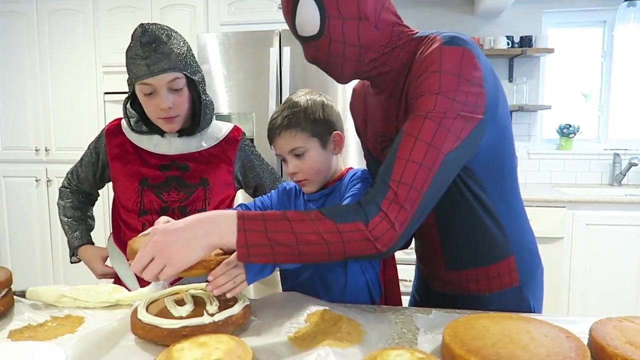 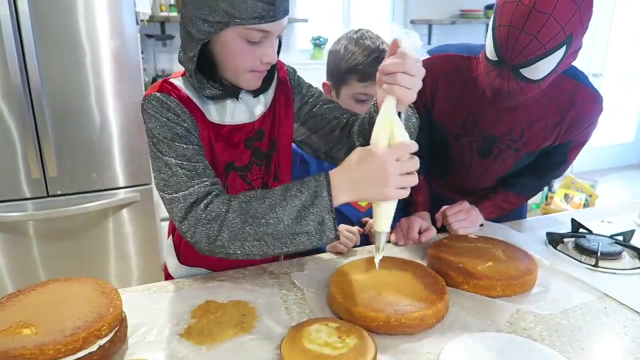 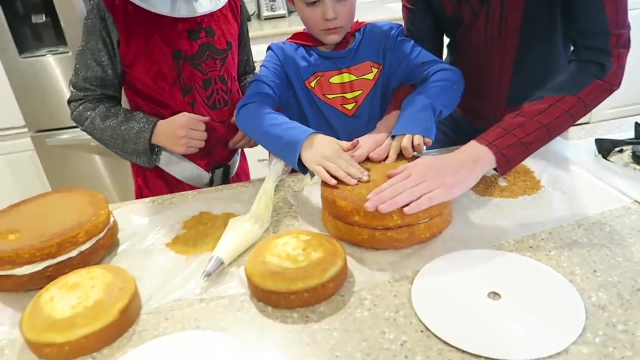 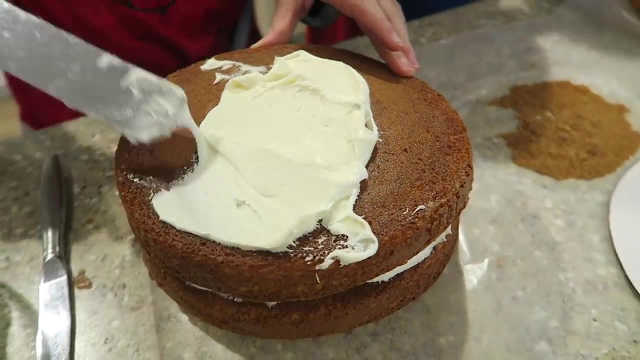 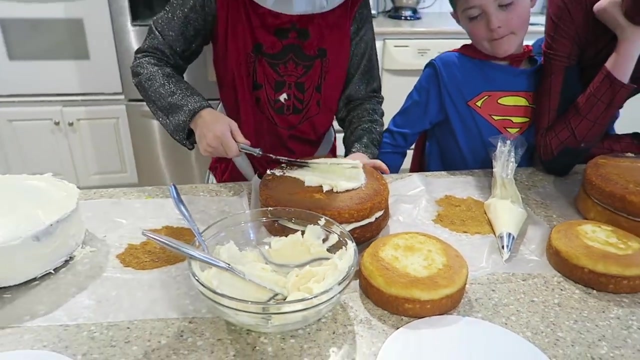 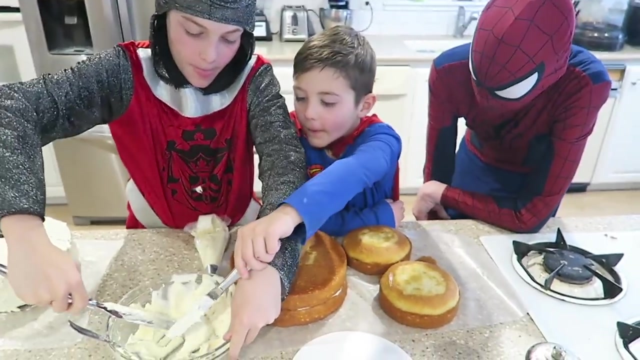 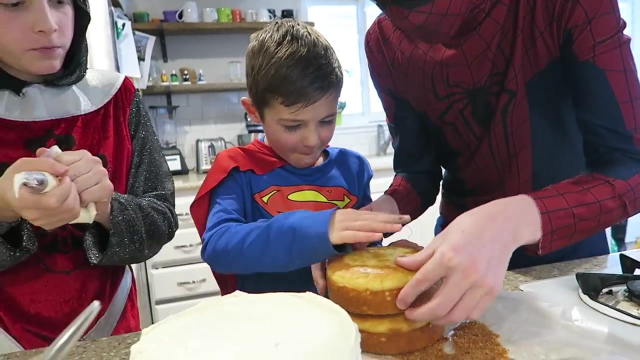 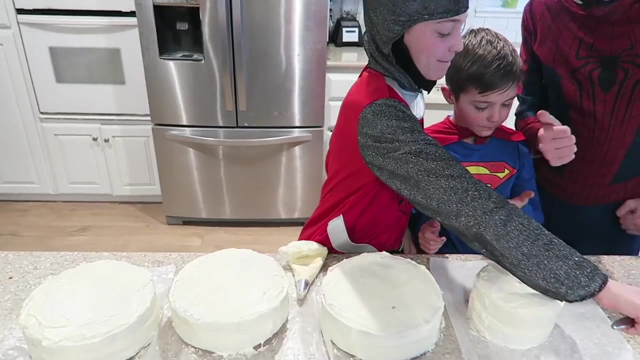 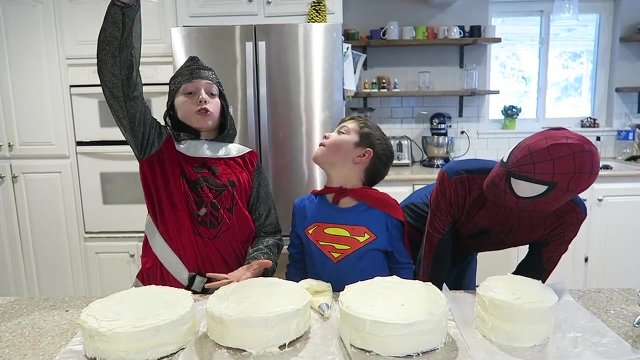 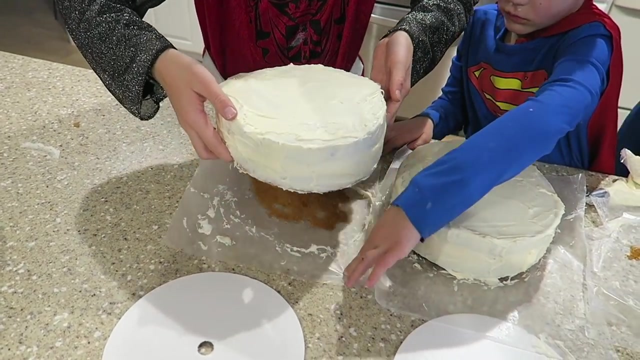 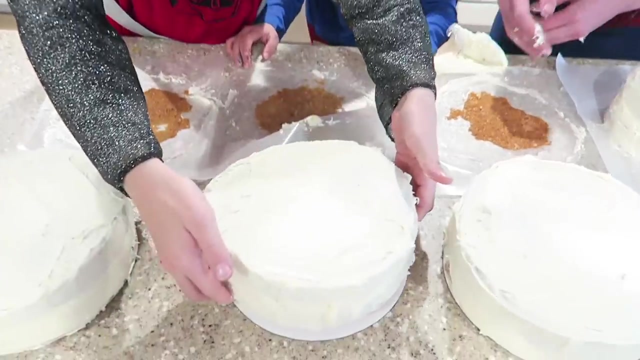 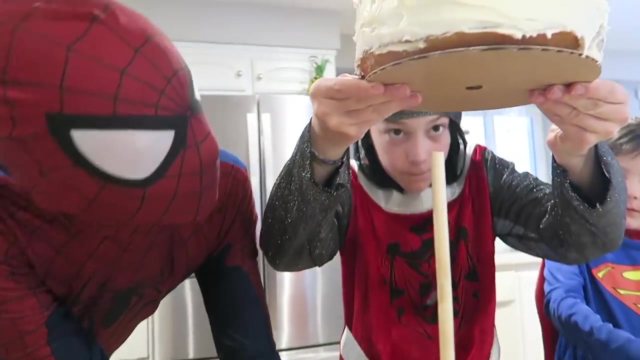 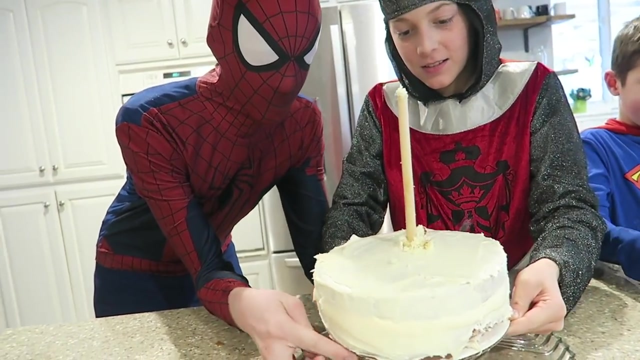 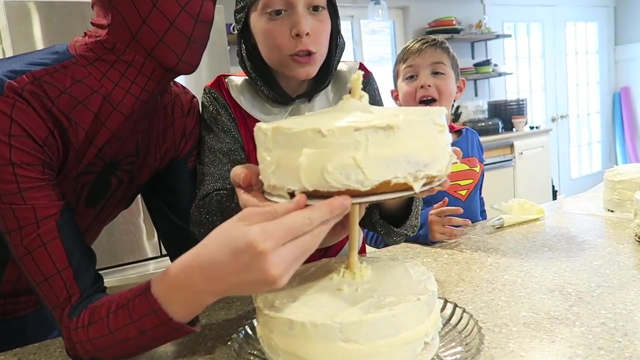 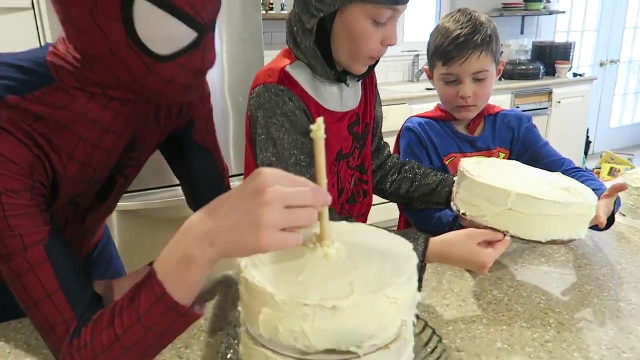 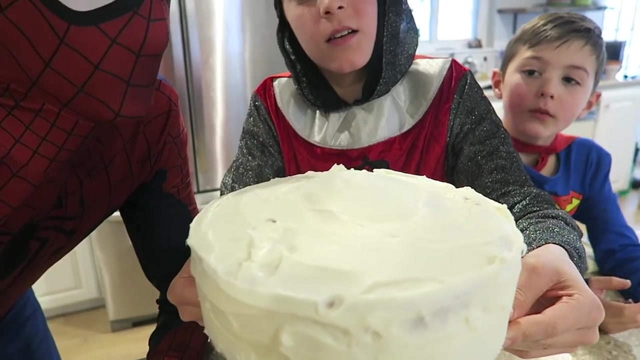 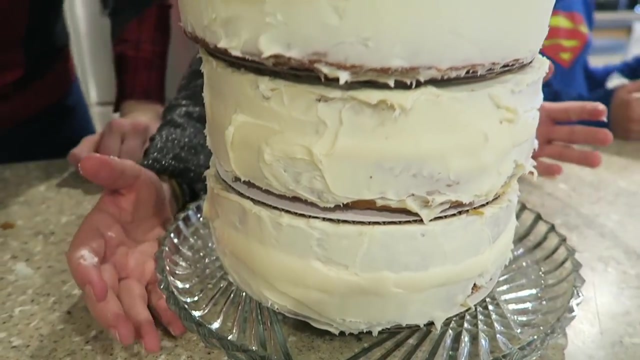 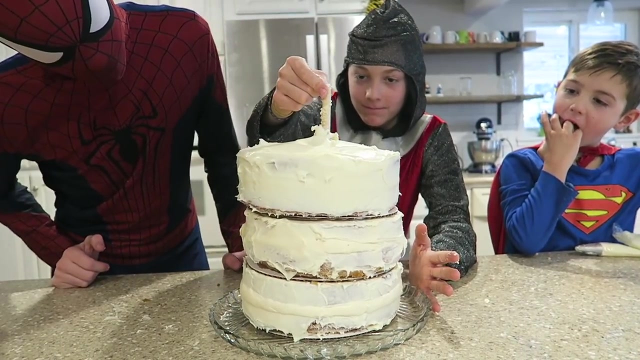 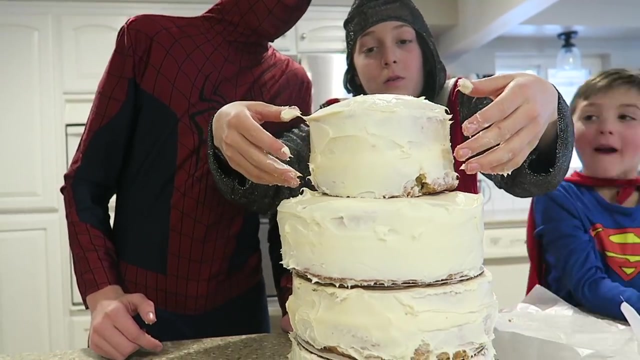 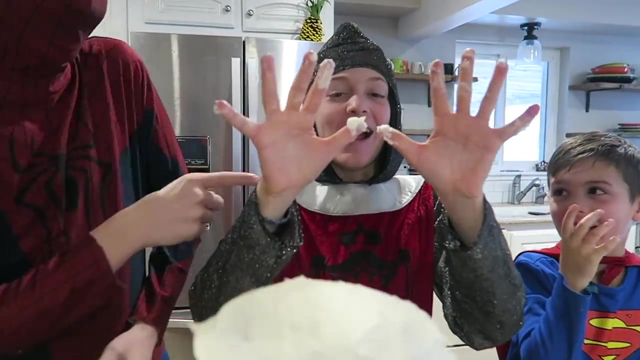 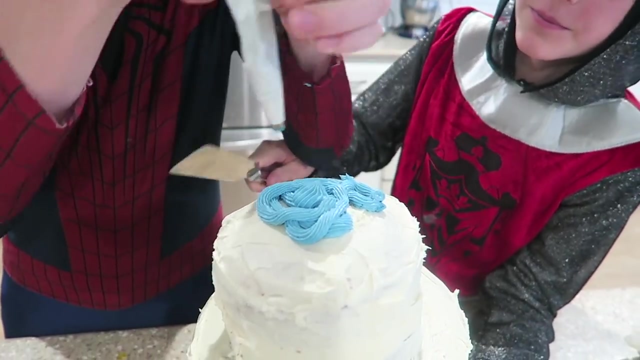 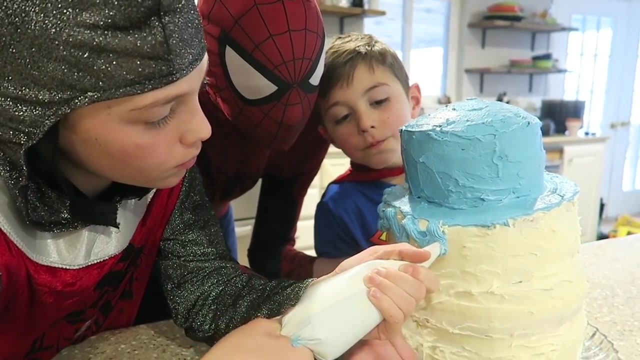 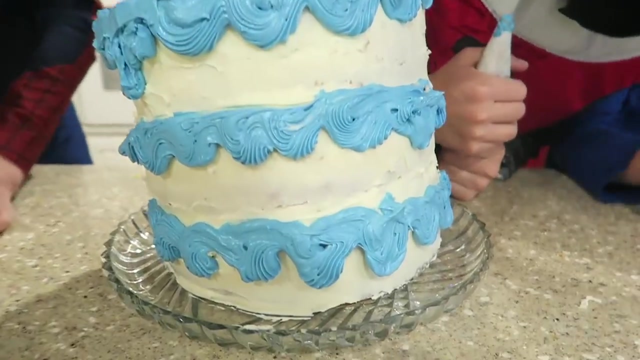 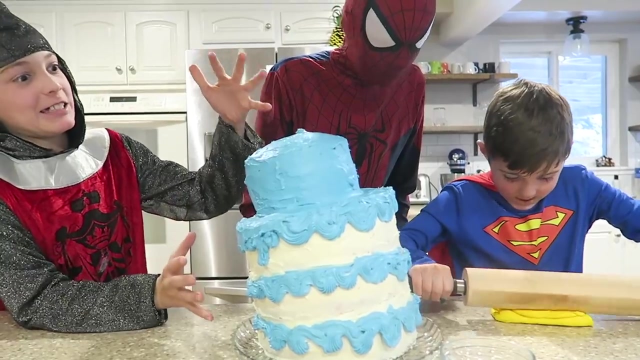 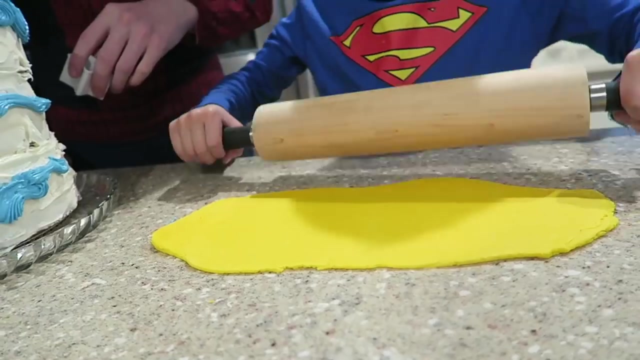 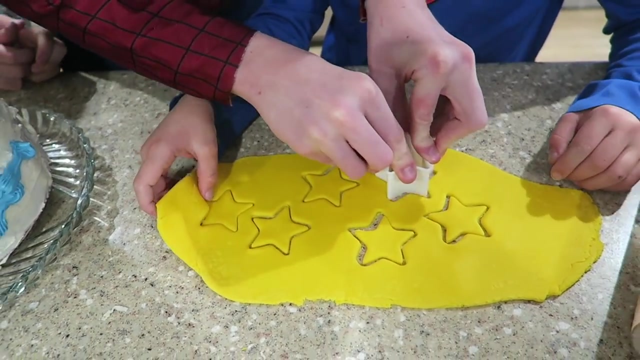 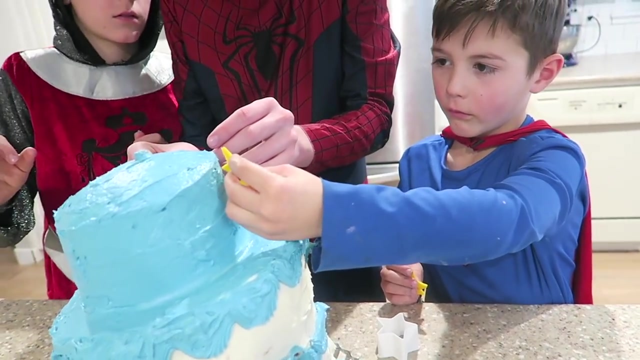 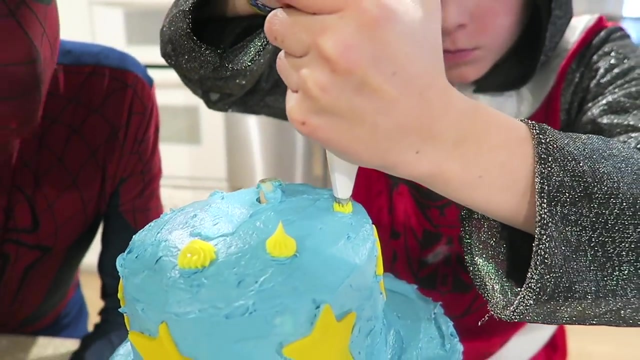 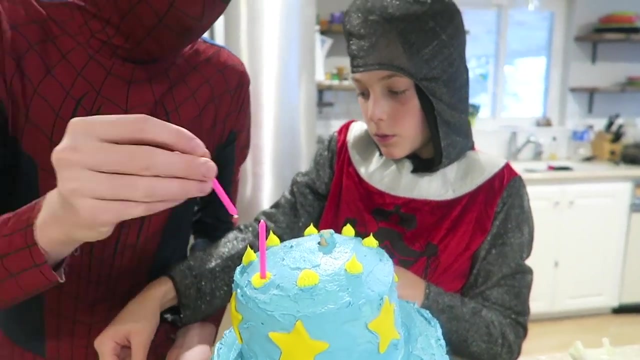 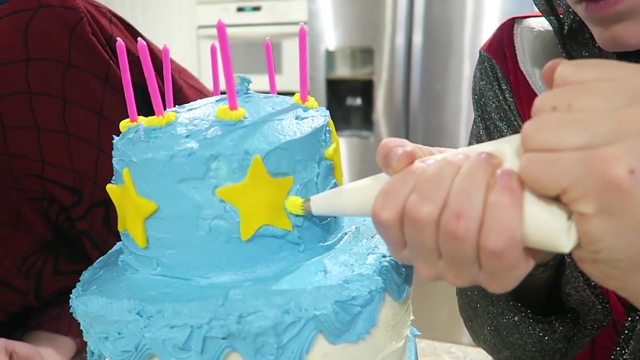 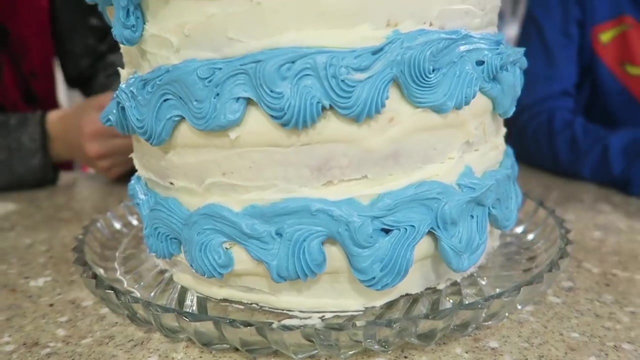 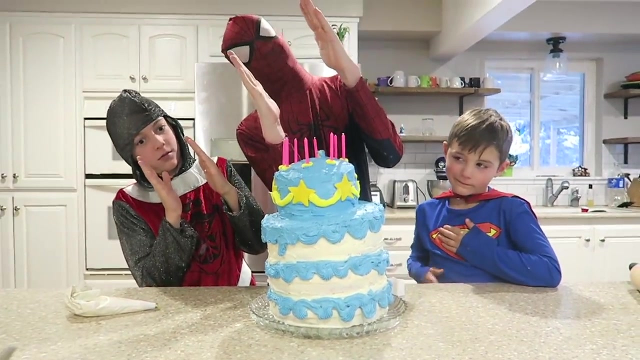 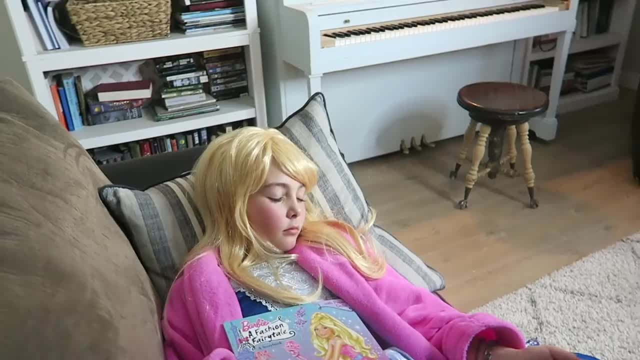 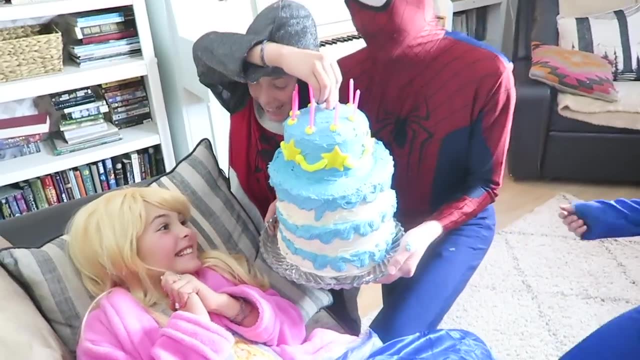 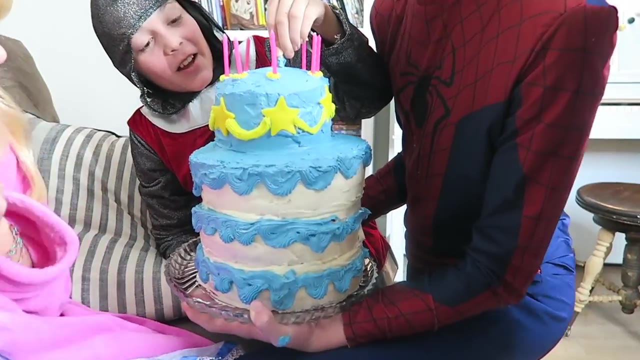 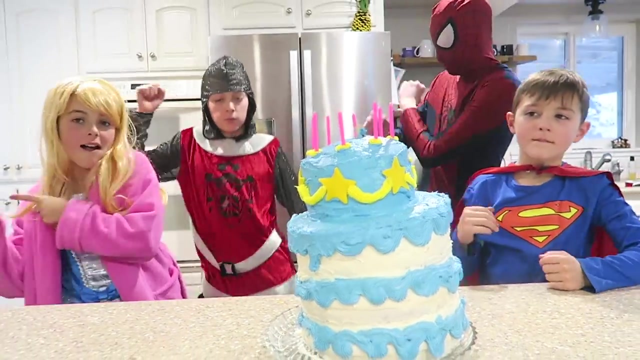 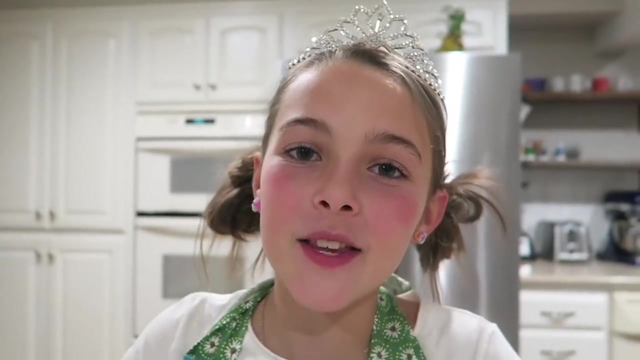 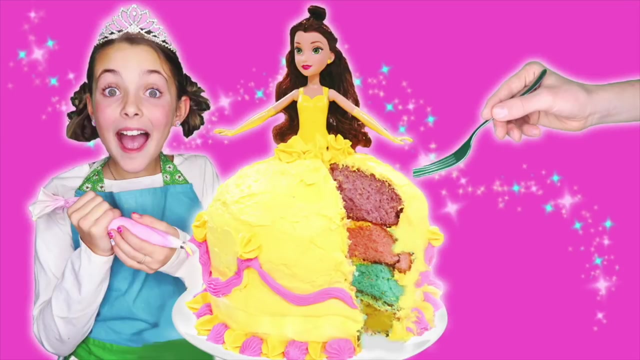 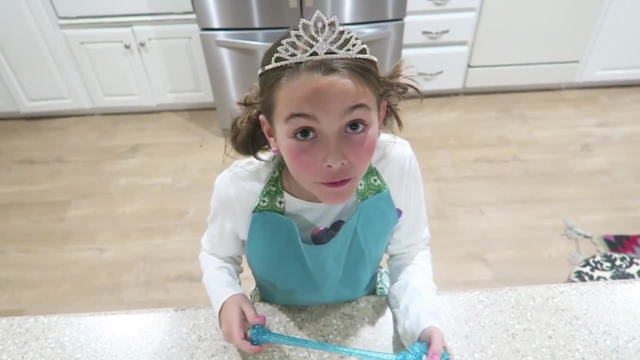 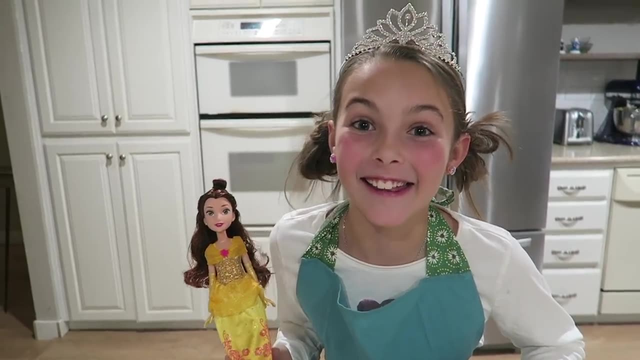 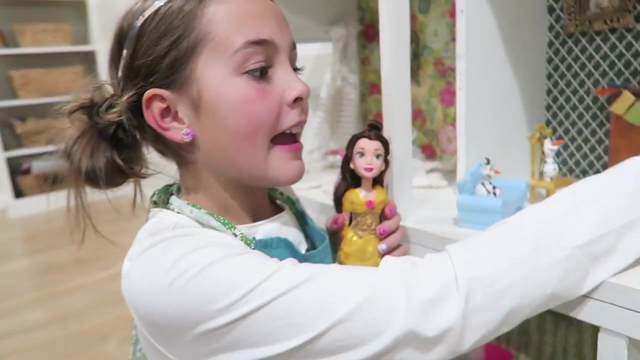 I love Beauty and the Beast. The new movie is coming out in a few months. I'm so excited. I got the idea from my dolls and their dollhouse. You want to come check it out? Okay, let's go. I got a big bell and a mini bell. 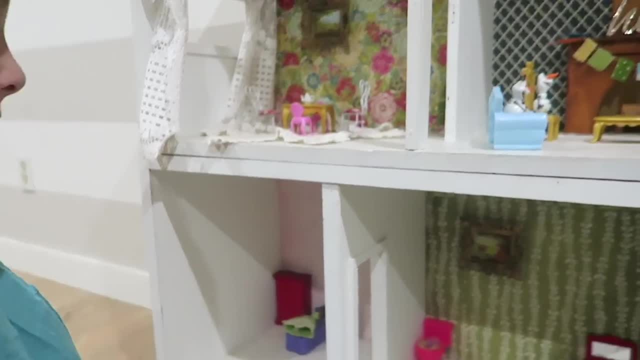 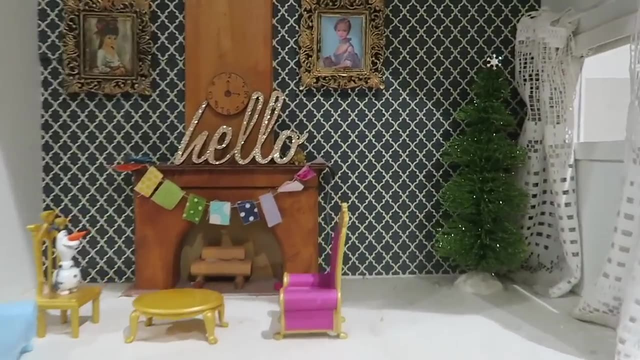 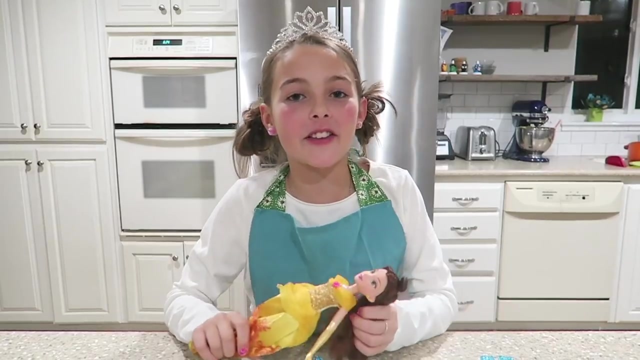 So this is the living room, this is the dining room, this is a bedroom, this is a bedroom and this is the bathroom. they have their own little tiny christmas trees. do you like the wallpaper? let's take our bigger bill and go make the cake. okay, so i'm gonna bling in all of the magical cakes, my magical princess powers. 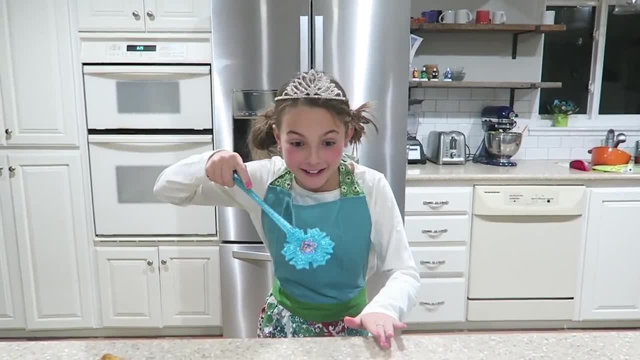 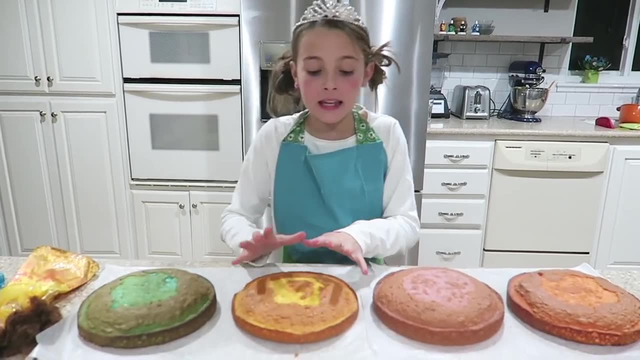 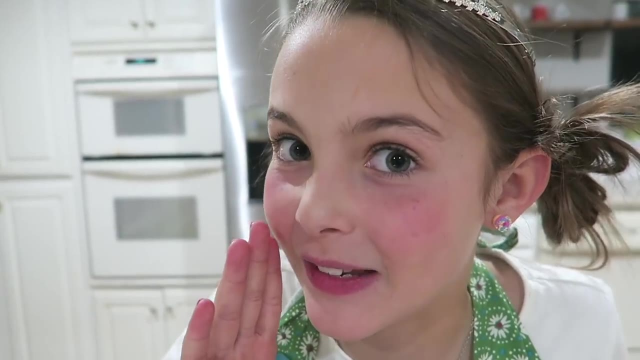 since i'm a princess- cakes, donuts and sprinkles. oh wow, these are so fluffy. this one is blue, this is yellow, this is pink. no, this is purple and this is pink. i actually made these ahead of time. let's get fancy. i'm putting the frosting on, so the cakes will stick together. 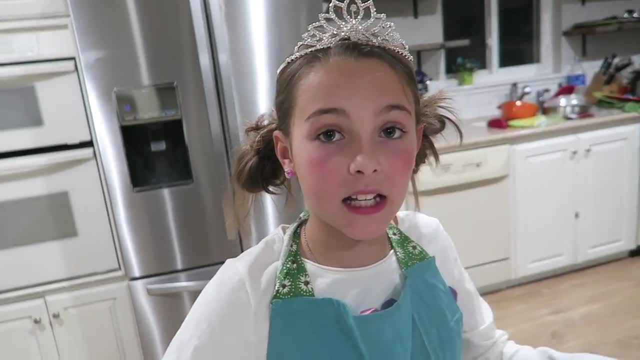 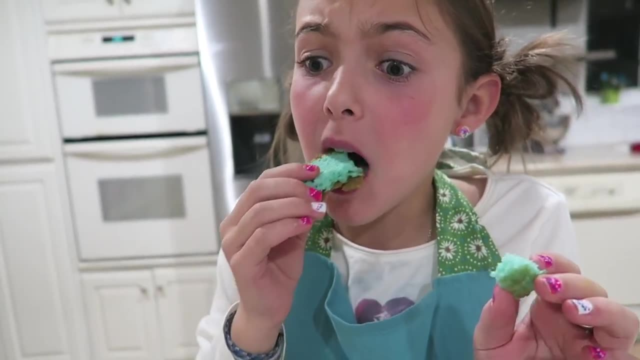 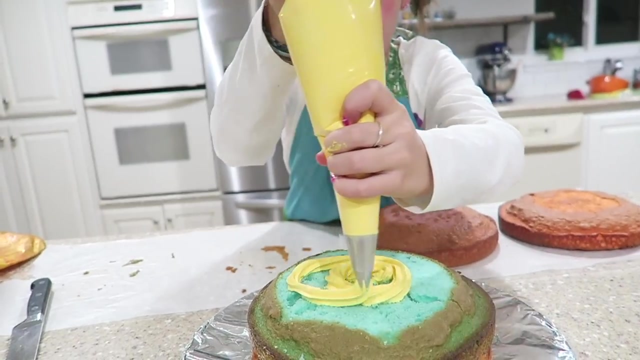 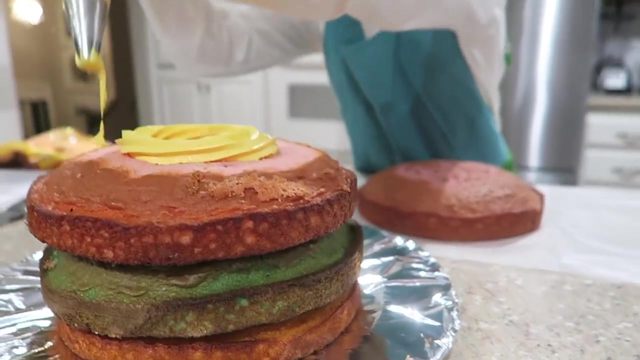 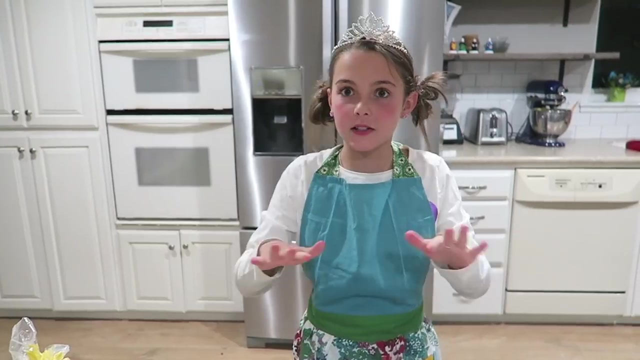 okay, so i'm cutting it flat so i have a good surface, so so i can put the next cake on. the blue is really good, i'm gonna do the thing again. last one: so i put the purple one on the top because it's more of a round. dresses are big. 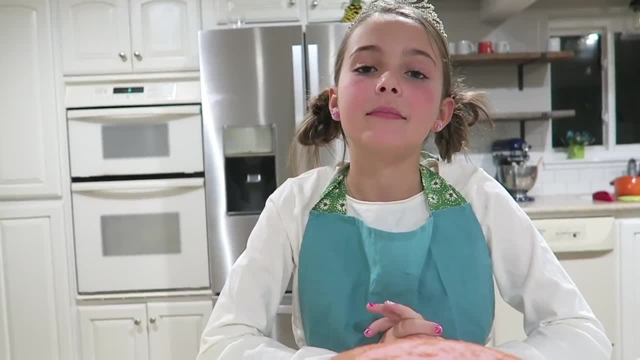 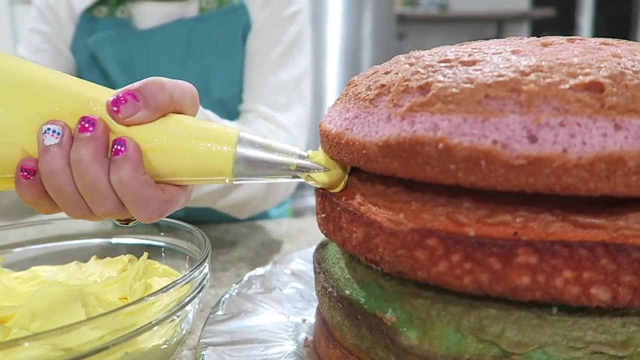 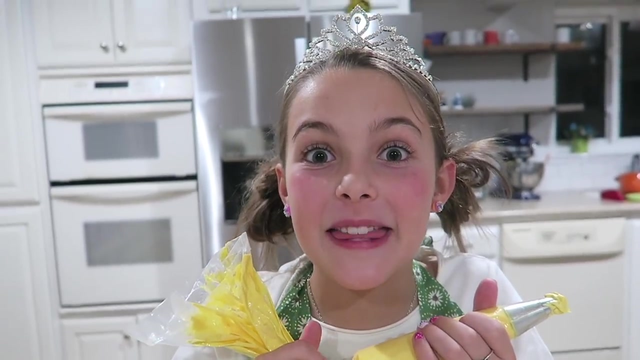 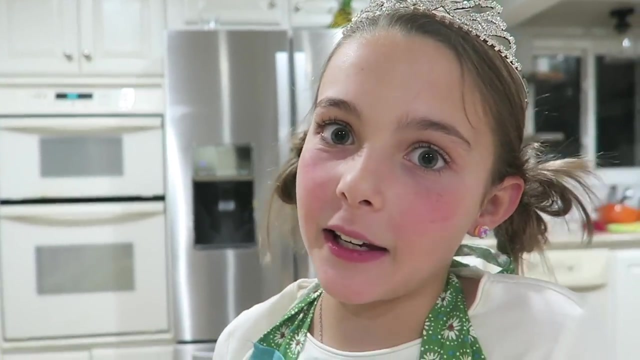 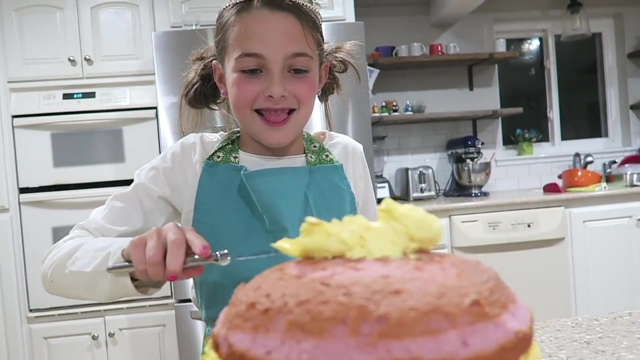 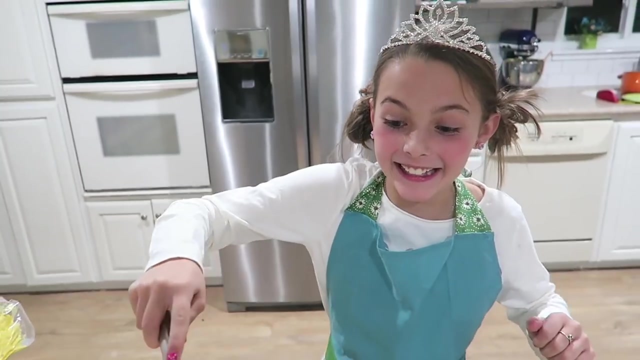 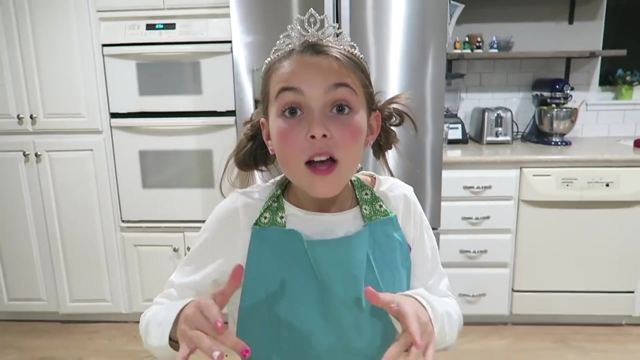 and poofy. so it looks like a dome- a dome like my head. it looks like a hamburger with extra cheese. i love hamburgers. did i mention that i like to eat food? now we're gonna make belle's poofy dress part. oh yeah, okay, i'm done. now this is the trickiest part. you have to cut a hole to fit her legs. 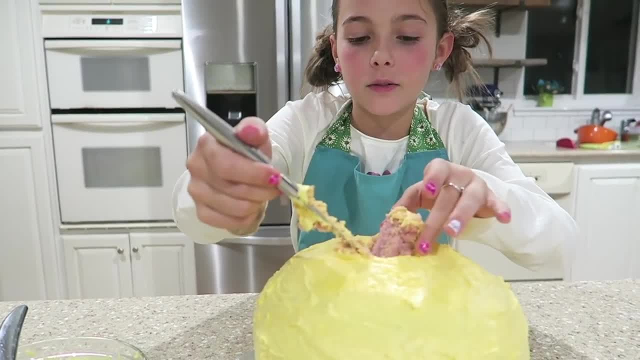 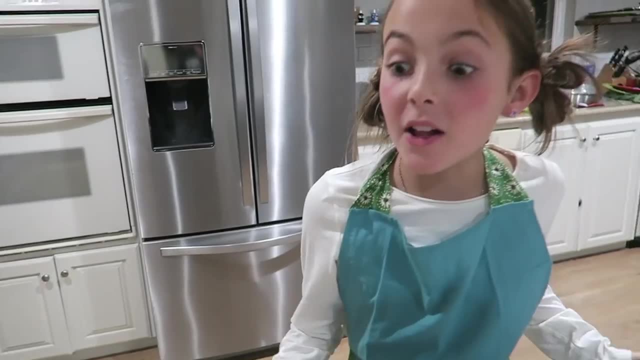 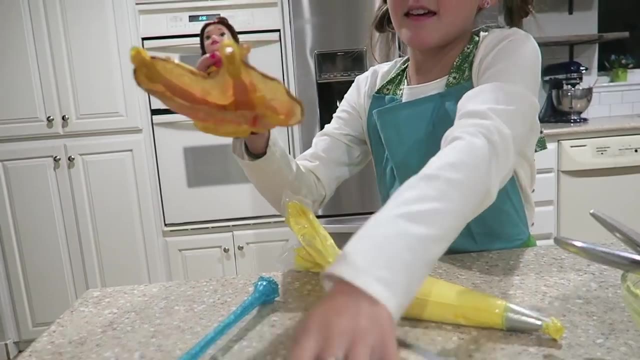 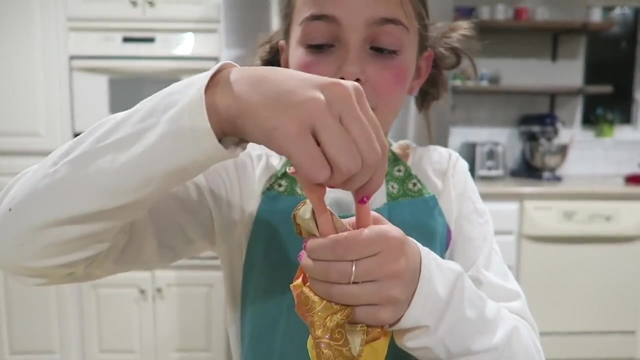 this is where it gets messy. you have to cut a hole to fit her legs. bell, quit reading that book and get over here get it, because she reads a lot. okay, now we gotta take her shoes off. her shoes are so pretty. you ready to dive in? let's do this thing. 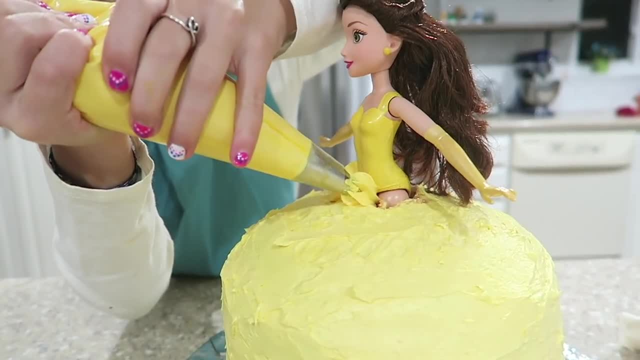 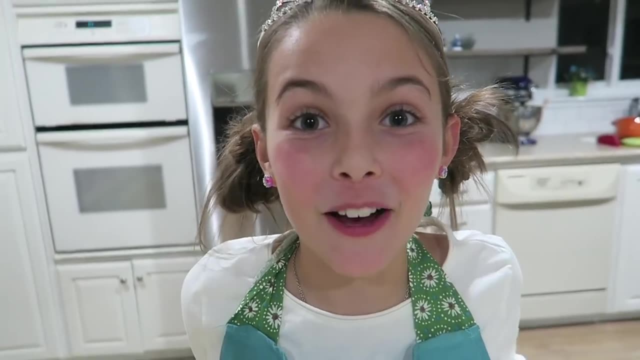 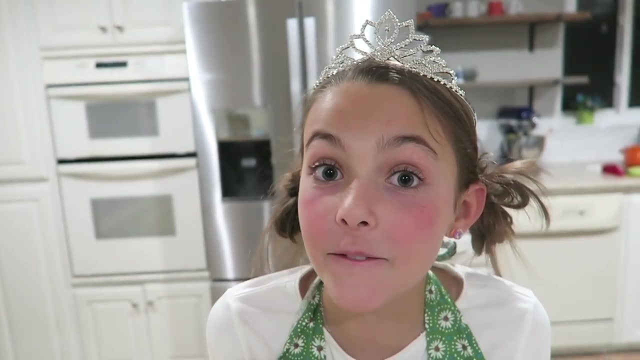 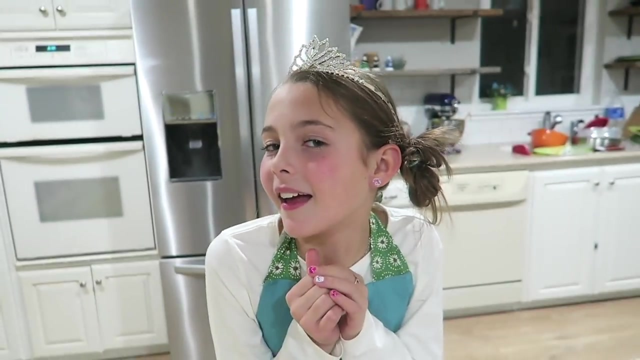 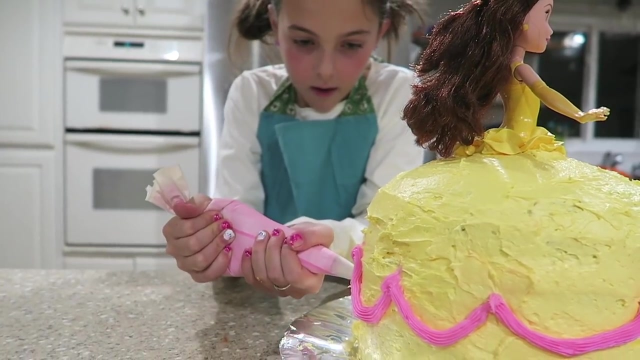 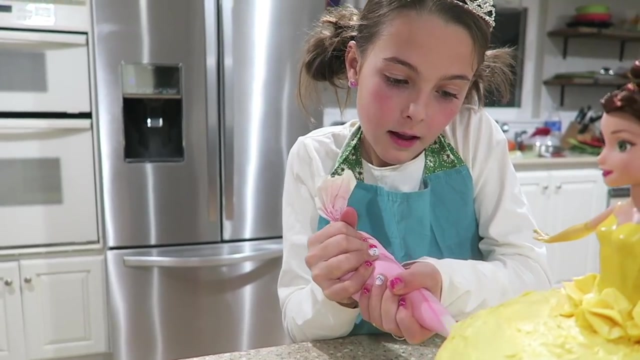 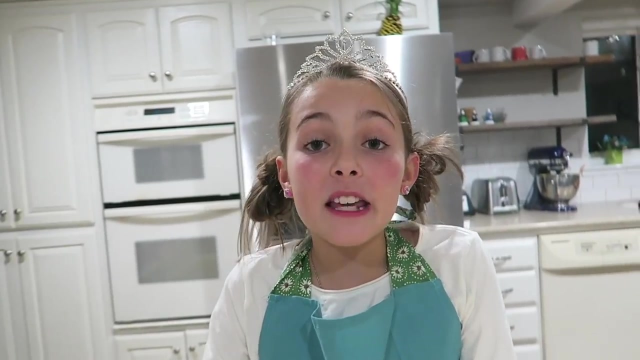 so now comes the fun part: pink. did i mention that i love pink and food? that's why i got these pink donut earrings? i got them for christmas from santa. they're amazing. i love this. oh, now i'm gonna make the bottom of her dress really pretty. i'm going to alternate yellow and pink. 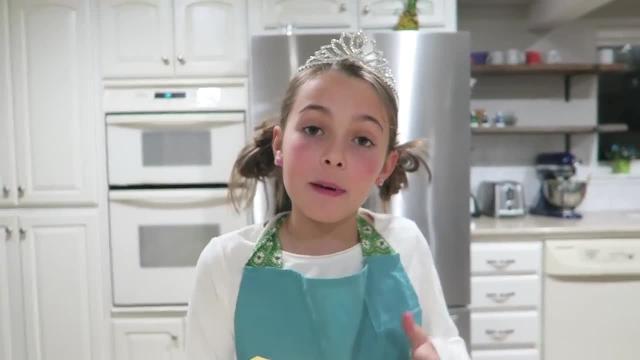 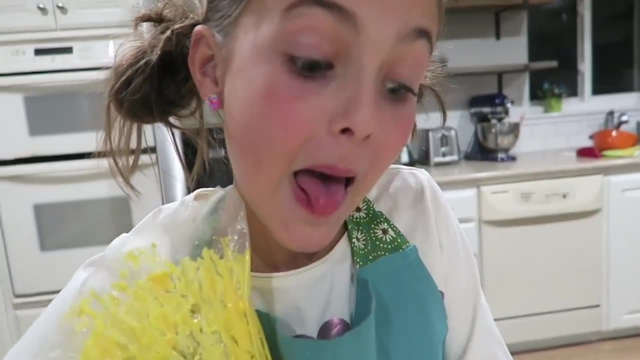 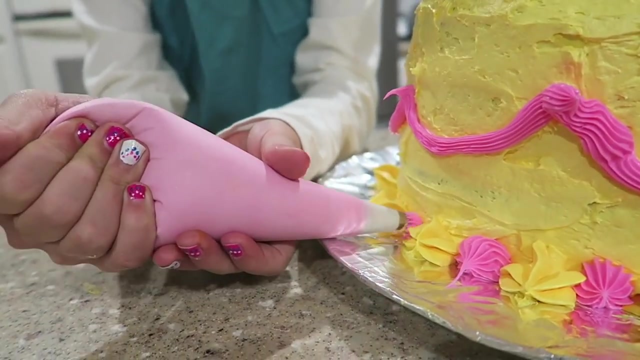 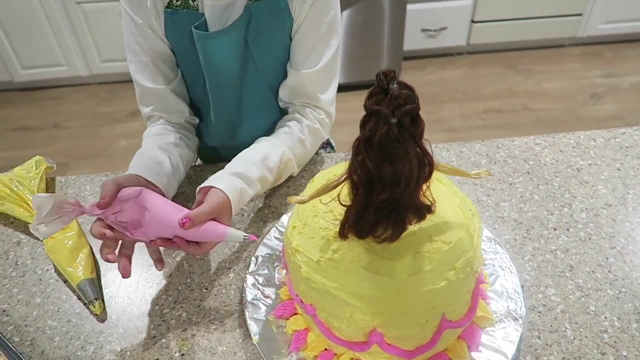 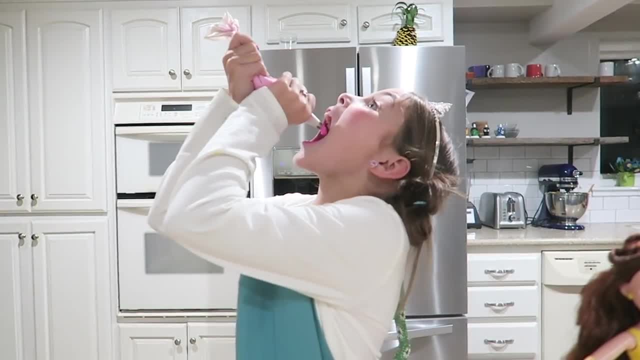 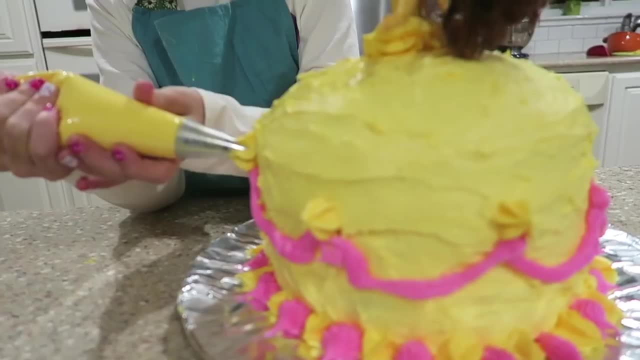 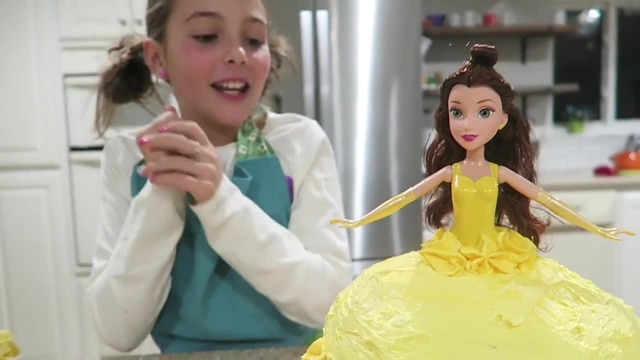 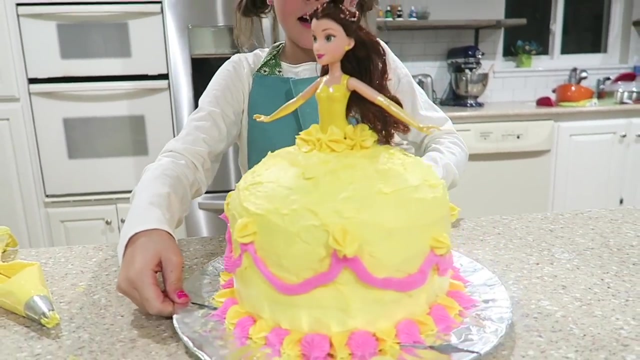 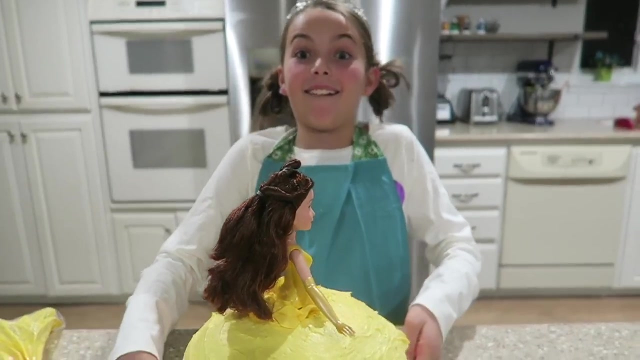 All done. Now I'm going to get the yellow and put like little dots up there. We're done. Okay, She looks so beautiful, Belle, take a spin, Isn't she so beautiful, So beautiful. I want to eat her. Oh my gosh. 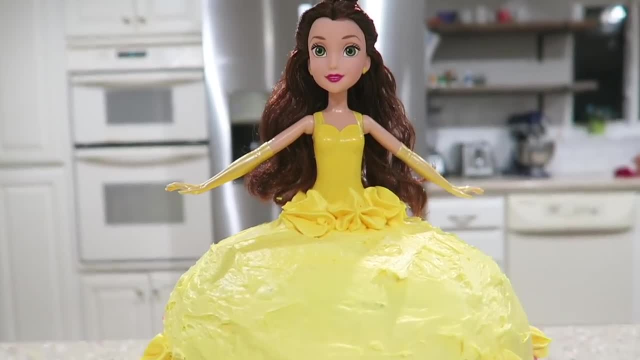 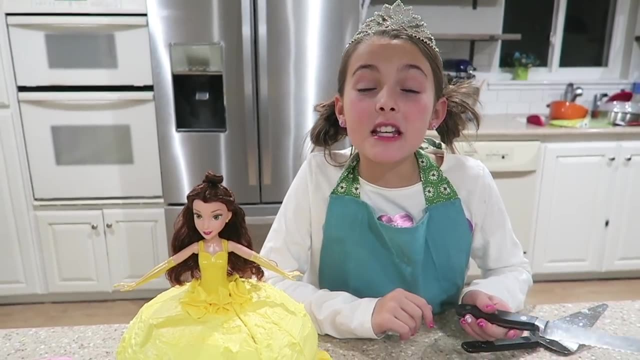 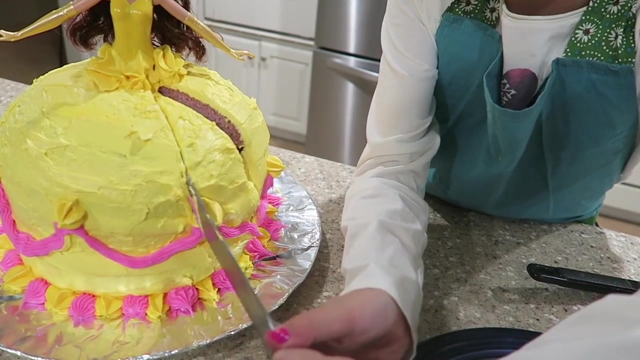 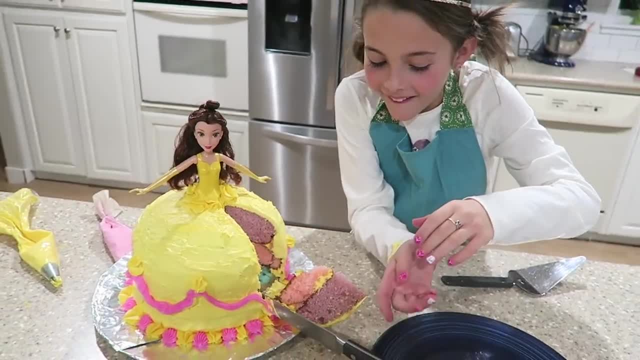 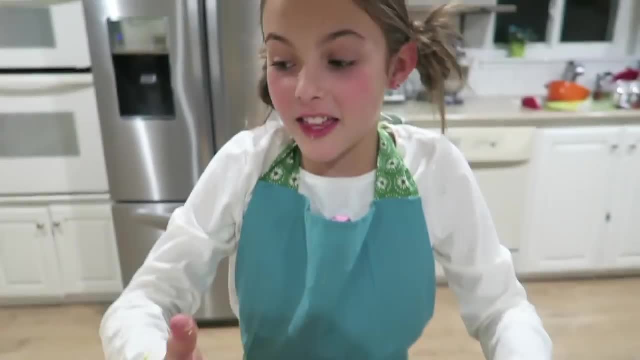 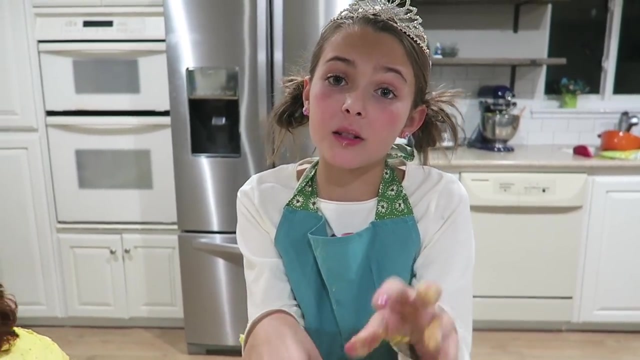 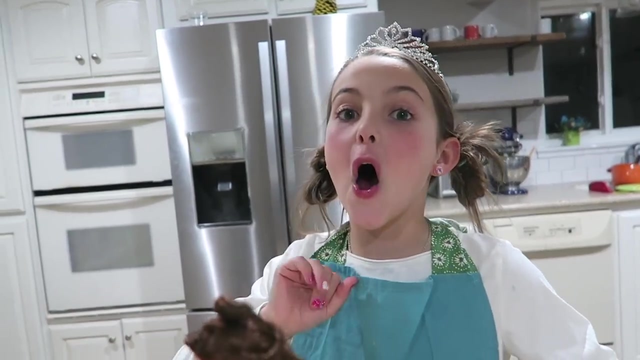 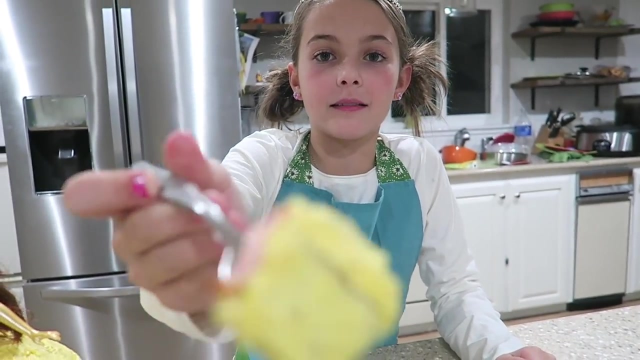 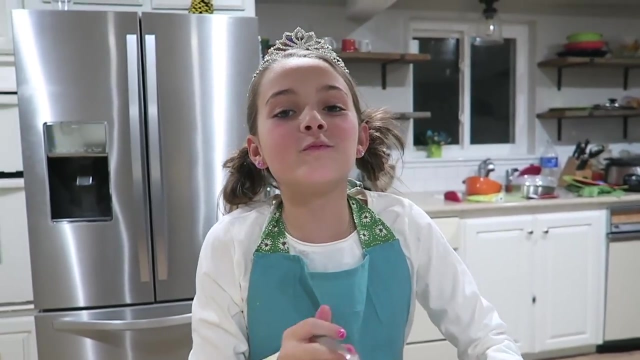 Oh, Look at all these rainbow colors. Oh, Oh, Oh, That was all. so one of the messier parts, because I came – the cake broke. All right, Now for the funnest part of all time: Taste test. There's one more time. 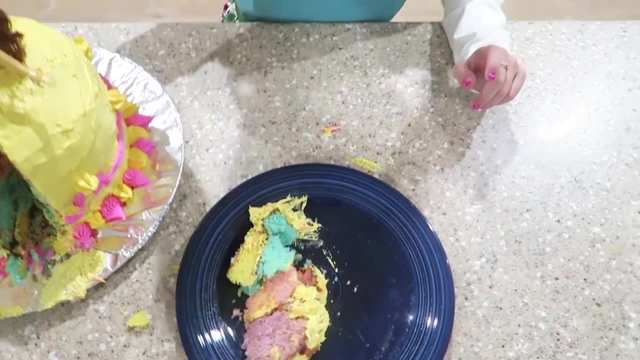 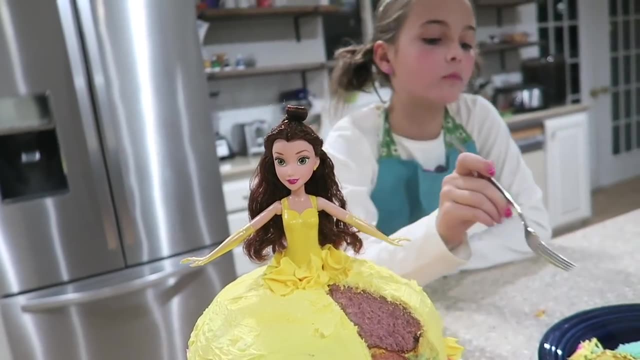 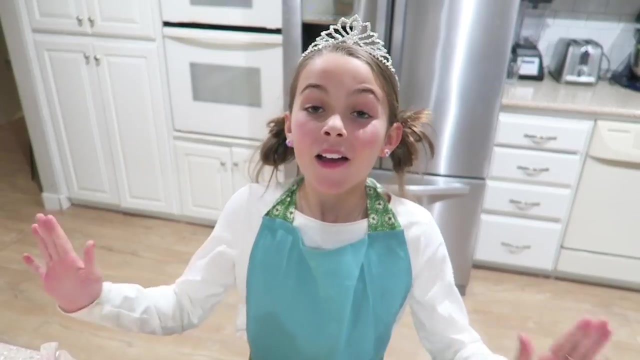 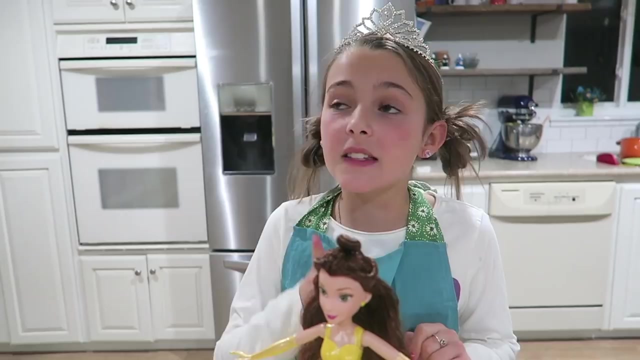 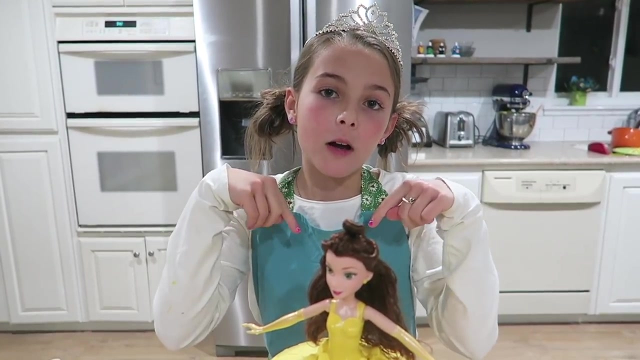 It's so good. Thank you guys so much for hanging out with me today on Kids Cooking Crafts, making this homemade Beauty and the Beast rainbow bell dress cake. Check out our other cake videos here here, maybe here and here, And don't forget to like, subscribe and comment below. 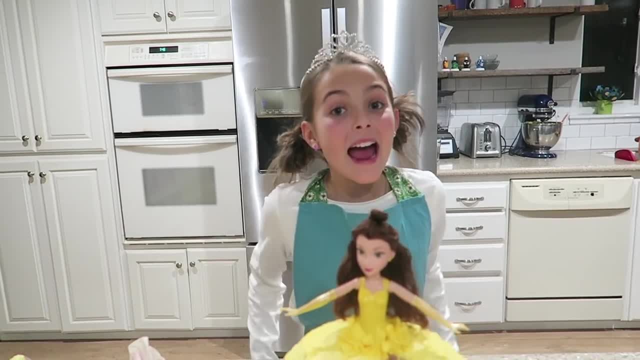 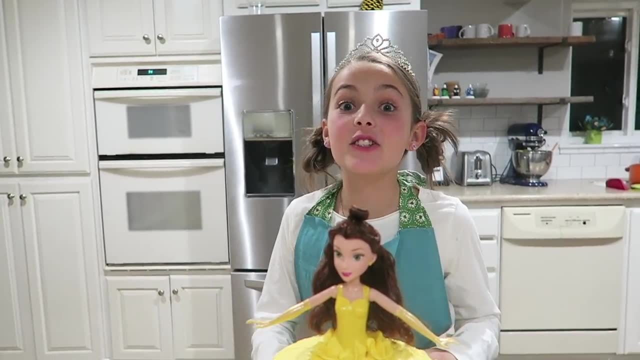 If there's something that you want me to make, tell me in the comments below, And if you make a dress cake like one of ours, take a picture and send it to me Now. I'm gonna call my friends and totally have them eat this cake with me. 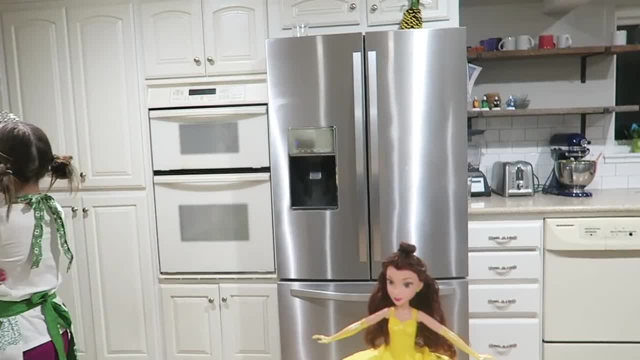 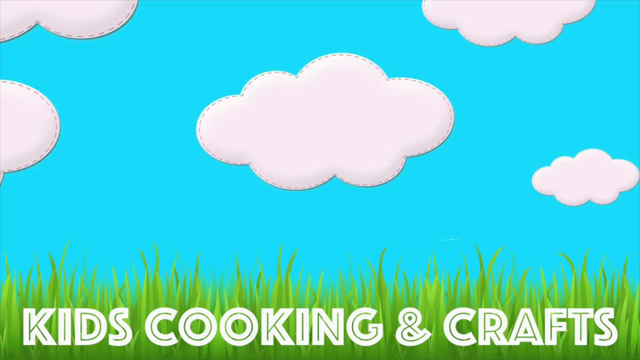 Oh hi, Kayla. Yeah, do you wanna come over and eat this cake? Yeah, yeah, let's do it. Thanks for watching and I'll see you in the next one. Bye, Bye.